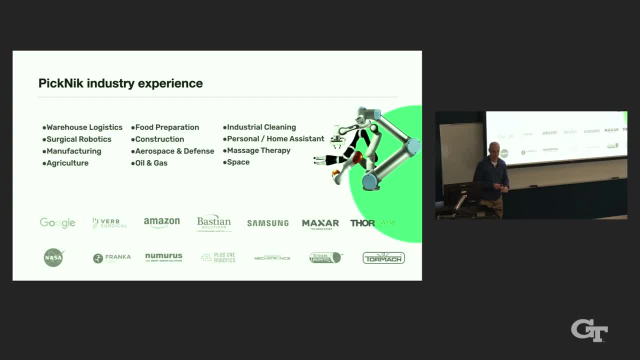 we work on sort of warehouse robots, where you will find lots of robots, But we also work on robots that are not as well-established, like not working robots that are five percent faster than a competition, but more like developed robot systems. that really isn't a good basis. 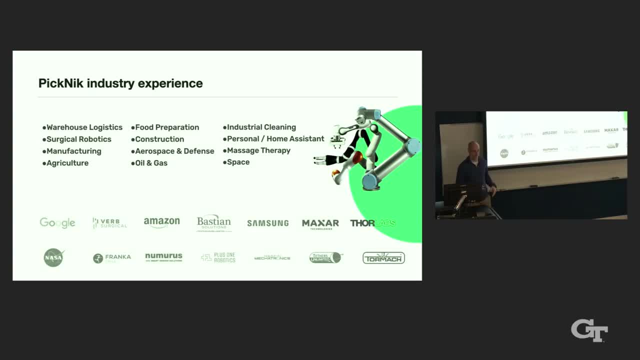 for comparison. So we've worked on kitchen robots, which is really a lot of kitchen robots companies now and ghost kitchens, but also in-home kitchens, Agriculture, fruit-picking robots. manipulating food is really hard. There's lots of perception, challenges and 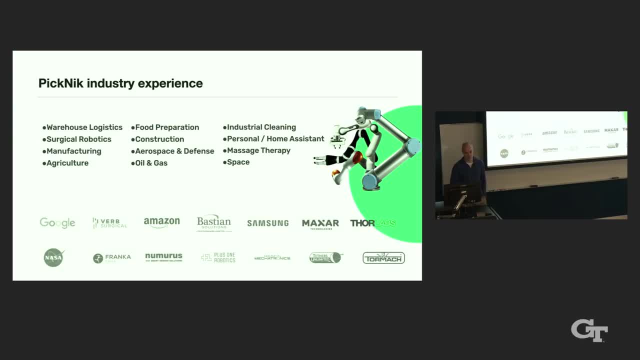 control challenges and construction. You see more and more robots, And lately also in space. We work with NASA, but there's also increasing interest from commercial space companies in what to do with robots in space, So we're happy to work with all of these companies. 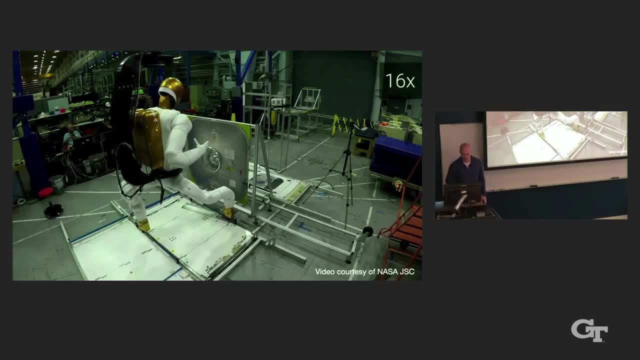 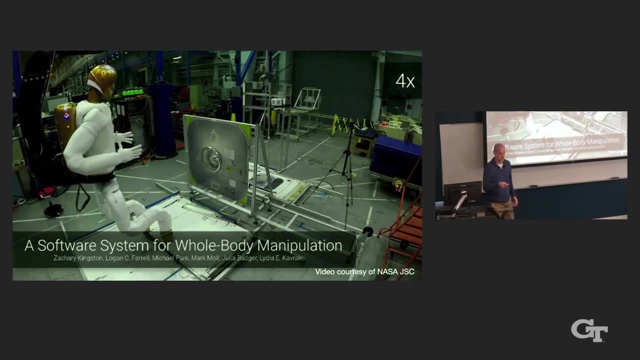 So, starting with space, this is sort of a motivating example to set sort of the stage for what I'm going to talk about next. So this is some of the earlier work that I did at RISE, And actually a lot of the results that I'm presenting today are based on work I did at. 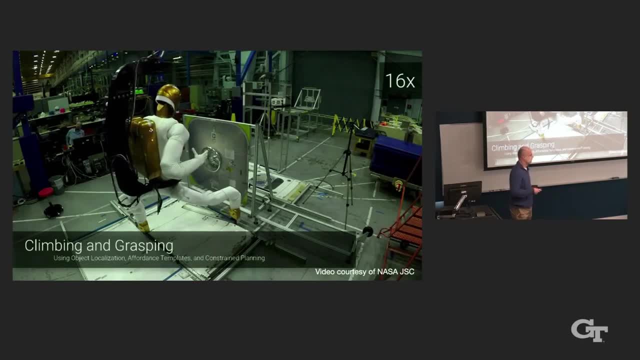 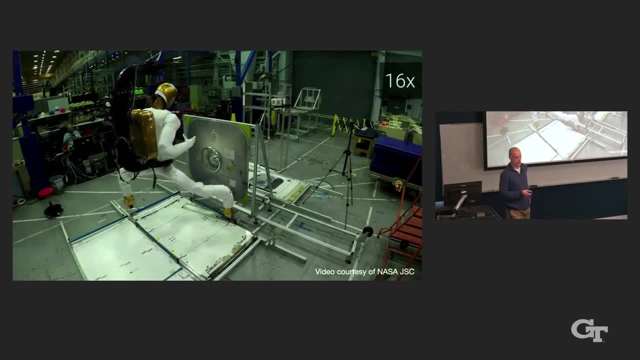 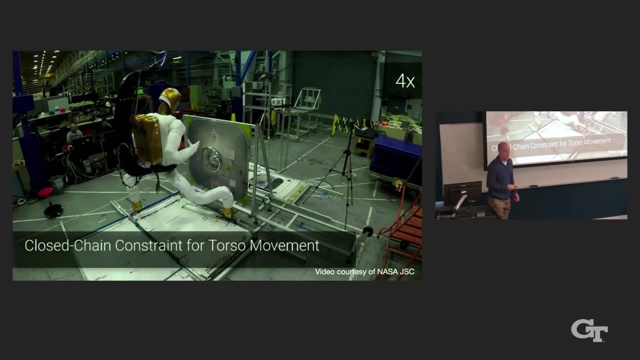 RISE. This is joint work with NASA, where we see a humanoid robot performing a routine task in the one-to-one scale models in the International Space Station. So the goal is to fetch a bag out of storage over there marked with the April tags, And to do so it has. 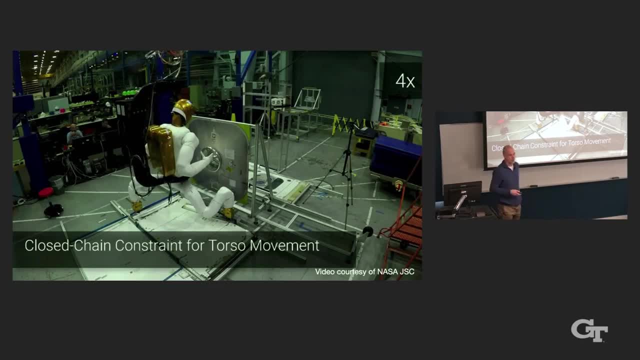 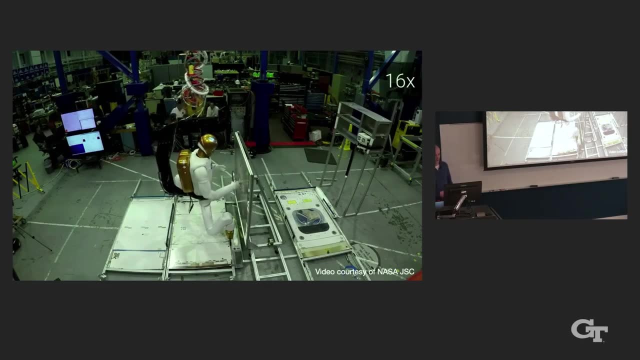 to walk across rails, open a door, take a few more steps and grab this bag. So you can see, the video has speeded up quite a bit And it takes a long time to actually do this, which is actually OK. Typically, this is something that we want. Mission Control. 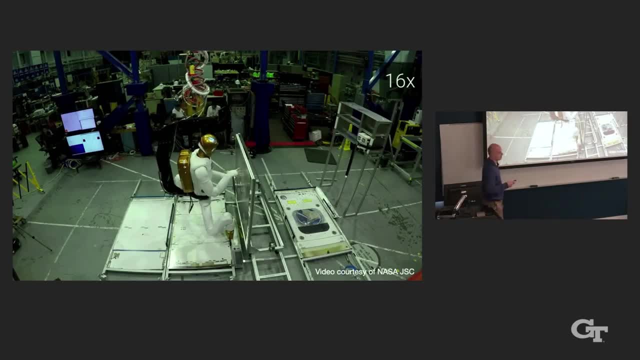 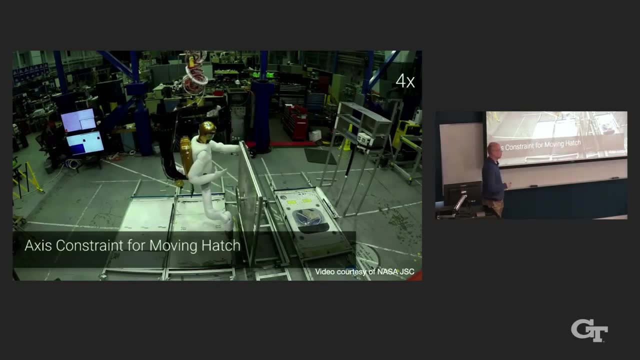 to do, And if they were able to completely autonomously script this event, then it doesn't matter if it's slow or not. The goal is to alleviate work from the astronauts, But the problem is that this cannot be fully autonomous. You cannot plan over that long. 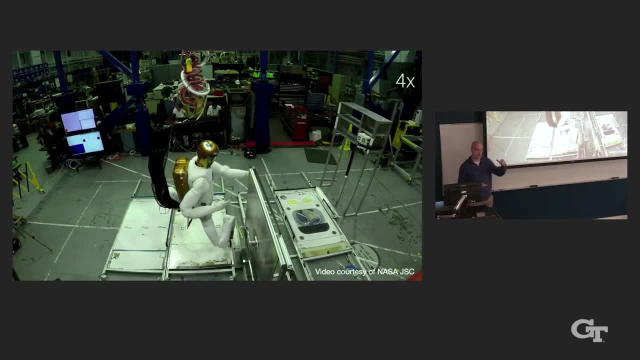 a time horizon, Most of the individual steps, we can be reasonably sure that they work. But the chance that all of it works and can be planned end-to-end just doesn't happen, And that's where we need some combination of autonomous planning and some human involvement. 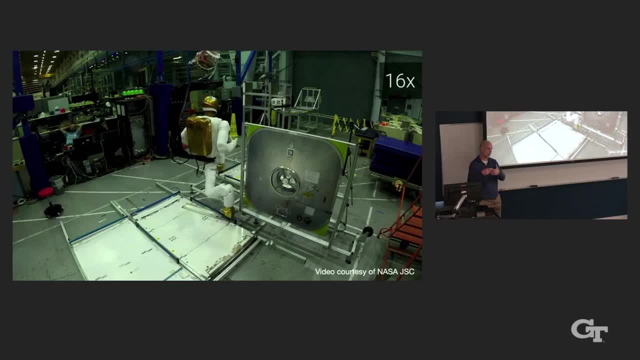 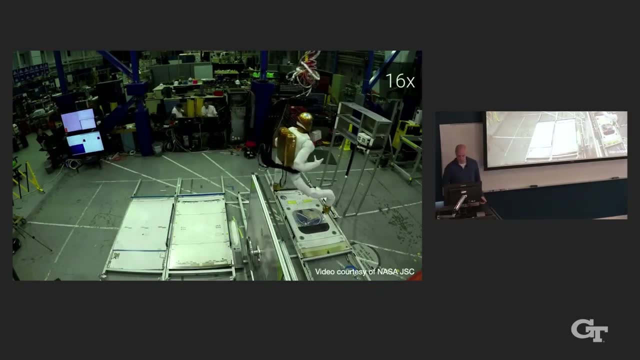 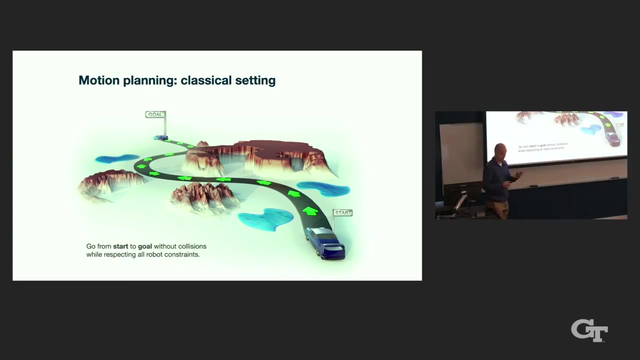 to make this possible. So I'll start with the motion planning And towards the end I'll describe our plan for making this more autonomous, with some human in the loop. So let's start from the very basics. So motion planning really is a very simple problem. 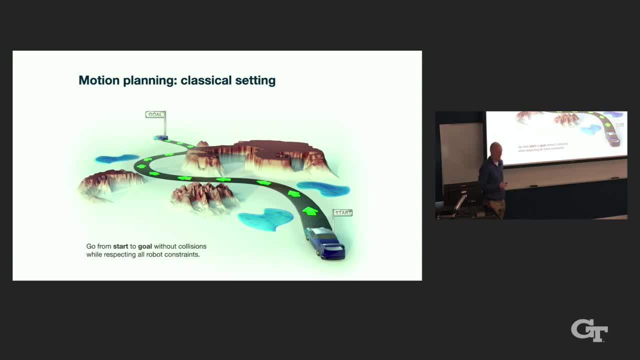 You think it would be solved by now, And Seth and I were just talking about this. Isn't this solved by now? Why are we still thinking about this? It's the problem of just getting from A to B without colliding with anything and while respecting kinematic and dynamic. 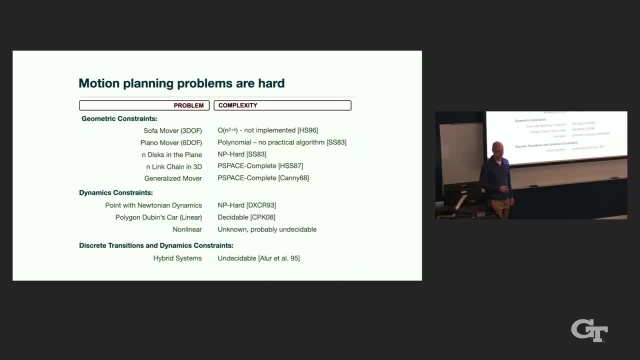 constraints. So some early results show that- mostly bad news- that yes, this problem can be solved, but in essentially exponential time. Any reasonable version of this problem is PSPACE-complete or worse. So we're non-computer scientists in the room. It just means that there's no known polynomial algorithm that 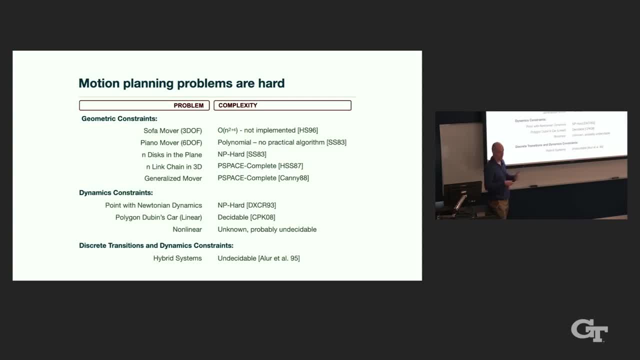 can solve this efficiently. As the number of dimensions grows of your robot, the number of degrees of freedom grows, this problem gets very, very bad. And if you introduce interesting dynamics for some notion of interesting, it becomes really hard to even determine whether 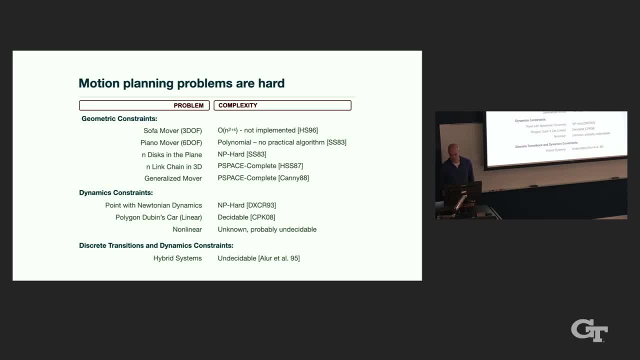 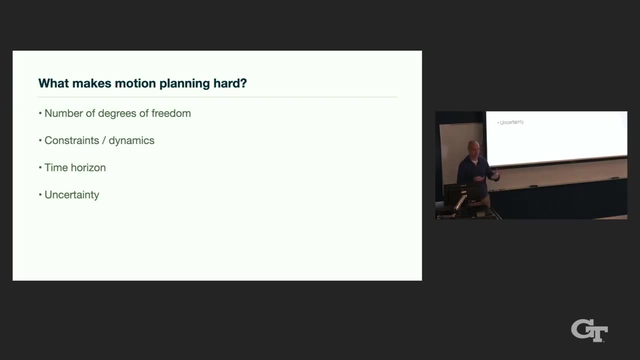 a solution exists. So this is the bad news. Luckily, there are practical ways to deal with this, as I'll talk about later. So, like I mentioned, the complexity is usually characterized in the number of degrees of freedom, like the number of joints that you may have, But constraints and dynamics usually 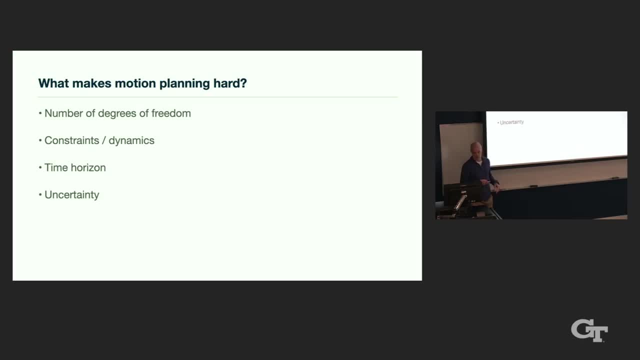 add some other notions of complexity, like whether, if you have- obviously if you have- second-order dynamics, then suddenly your state space grows quite a bit and you have more dimensions to reason about. Of course, that makes planning more difficult. The longer your time horizon is will also. 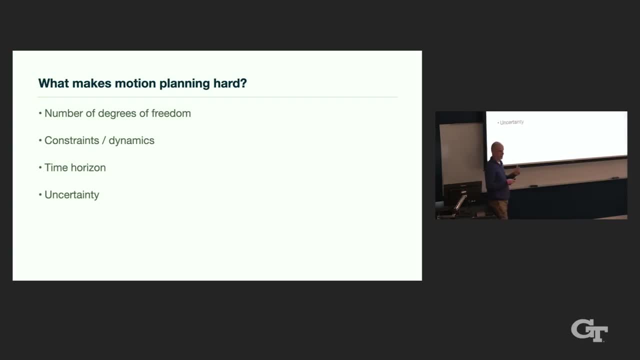 affect the difficulty And whether there's any uncertainty in perception or which really is not technically part of the challenging the planning problem. But as soon as you start doing planning in the real world, you have to account for perception of uncertainty, model uncertainty and actuation uncertainty. that will determine whether you can actually 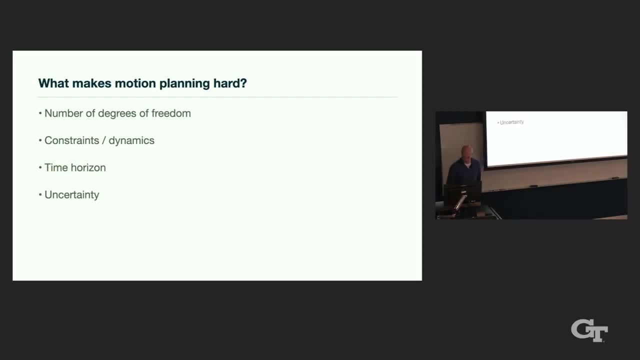 execute your plan or whether it makes sense to plan over longer time horizons. So over time, different planning approaches have come up. This is my rough taxonomy of approaches that exist today. So I have been working mostly in sampling-based planning. I'll give you 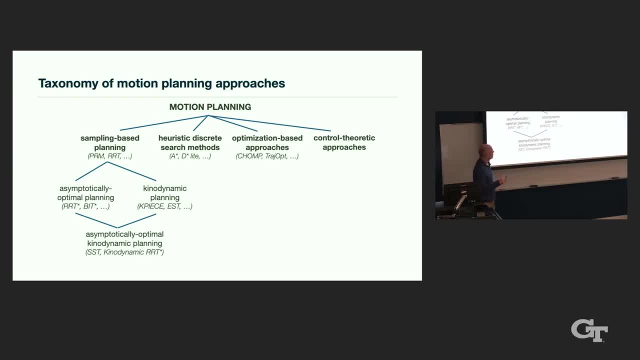 a brief review of that. But then there's lots of other approaches, like heuristic search methods, where we try to have a lattice of our continuous space And we search this lattice and we can efficiently search this and guarantee some notion of optimality with respect to. 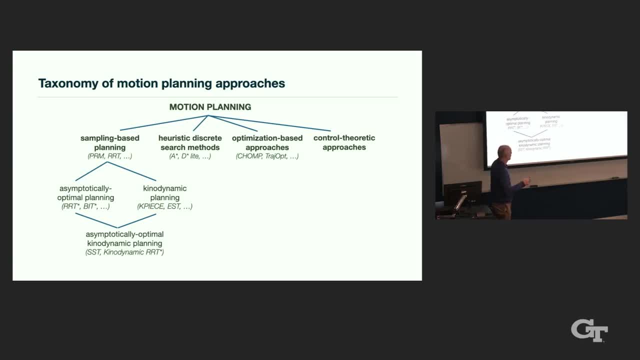 some cost function And, of course, optimization-based methods exist. Those would be very popular too, And if you initialize your initial trajectories randomly or in some way, you can still guarantee completeness, But typically they tend to be more local methods. And then, of course, there are control. 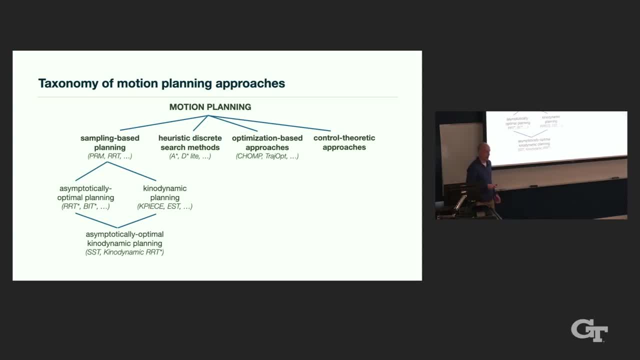 theoretic approaches that have been also very successful, but again over sort of more smaller time horizons. So within sampling-based planning, which I'll define and explain later, you can still account for dynamics. You have these kinodynamic planning versions of it And you can still account. 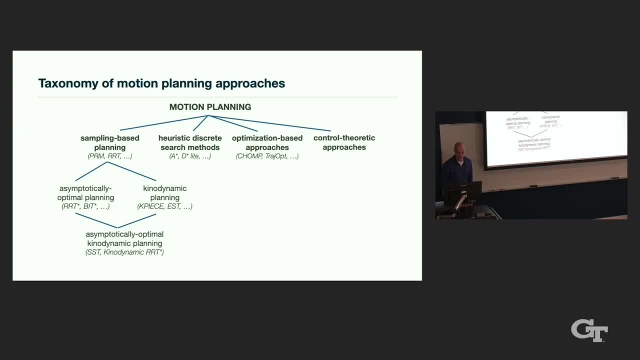 for optimality, And there are even combinations that try to do both. So, yeah, there's a lot of work in this area in trying to come up with different kind of performance guarantees and different kind of theoretical guarantees for these algorithms, And I'll try to give you a flavor of that. 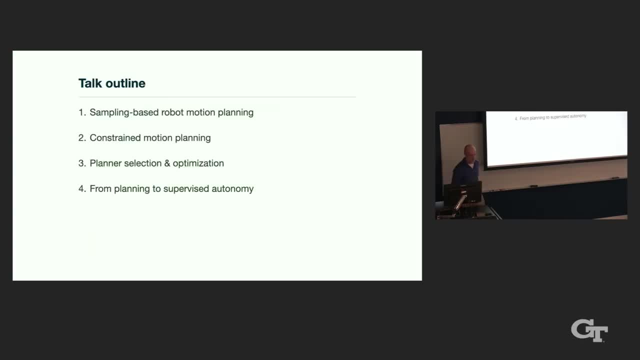 later on. So yeah, first a little bit of background to help understand. the rest of the talk is brief introduction to sampling-based planning. Then I'll talk a little bit about constrained motion planning, which is the way that we do motion planning in the real world. Typically, we're going to talk about the way that we're. 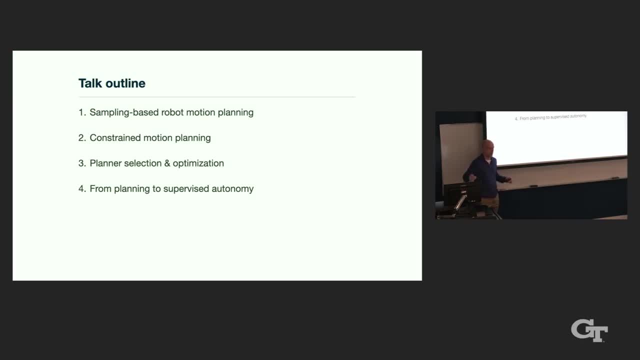 going to do it in the real world typically involves some task constraints. It's rare that we just move around in free space without having to worry about any constraints at all. Then I'll talk about a really practical problem that actually is kind of a big issue is that? 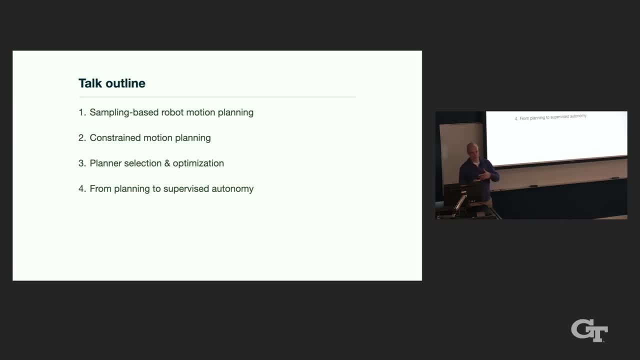 there's all these different planning algorithms And whenever you have a clever idea about a new planner, it's not really clear what you should be comparing against and how you do- or in any as a practitioner, like how you even select the right planner for your problem. 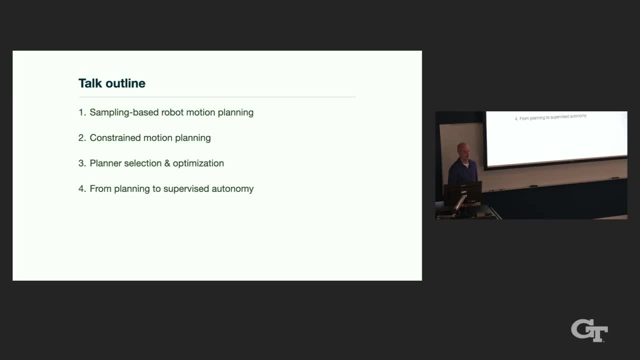 there's a lot of interest. There's a lot of yeah, I'll get to that later. There's a lot of work to be done, actually in sort of figuring out what makes what's the right planner for the job, And from there on we can switch to supervised autonomy and how we can combine. 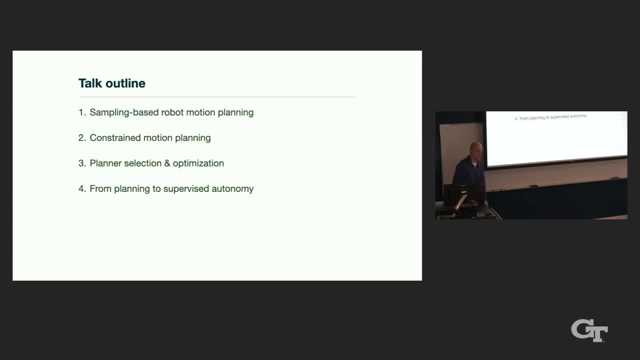 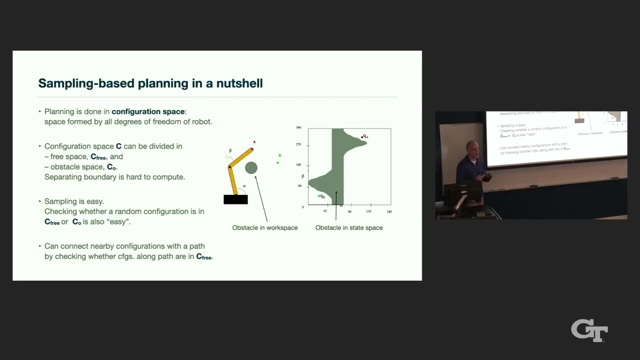 these planning as a building block to build something that is more functional for a fully autonomous system with some human oversight. All right, Sampling-based planning. All right, Sampling-based planning. All right, Sampling-based planning. Sampling-based planning is actually really simple, and the fact that it's so simple is: 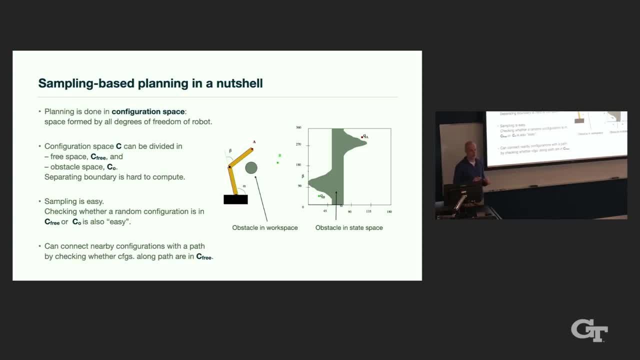 that there's a lot of a few operations that can be done very efficiently, and even though that doesn't seem particularly clever, the fact that we can do these operations very efficiently means that we can do them millions of times and we can actually plan very fast. 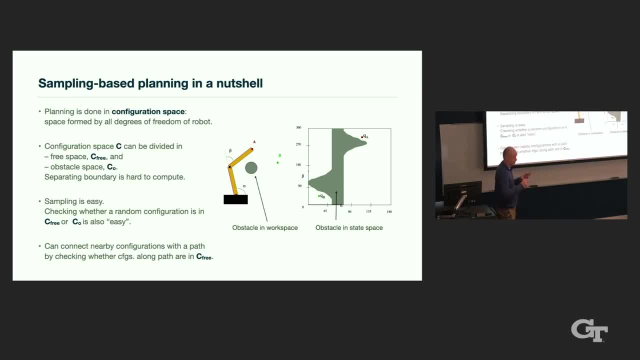 So the key idea is to understand configuration space. This is a very old idea. So let's say we have a two degree of freedom arm, the simplest possible arm. There's a joint here and there's a joint there and it's a circular obstacle. 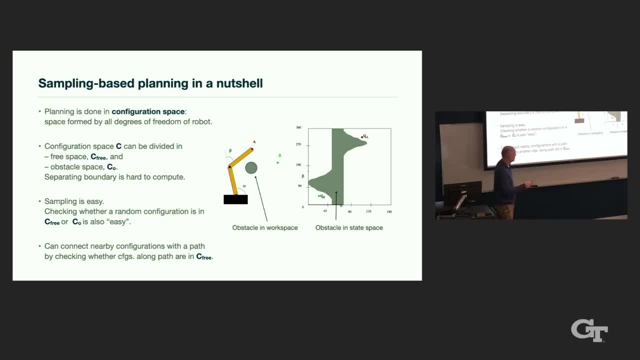 as a circular obstacle And we can basically plot the configurations over here in the right, where every point represents a robot configuration, And we mark configuration as in collision when it collides with the circle and white if it's not in collision. So you get this really weird shape. 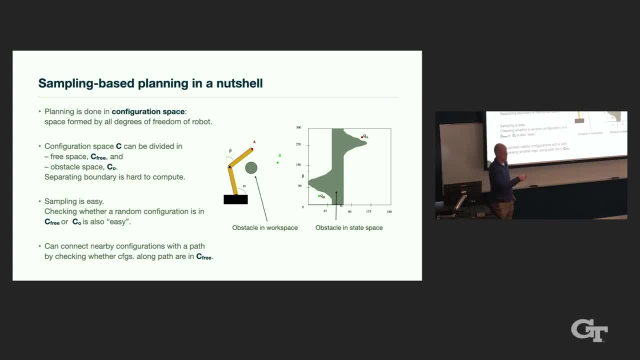 and it's not completely intuitive how a robot and the geometry of the environment maps to this shape, But this is the most convenient space to plan in. So if you want to find a path from A to B, it looks like there is no path. 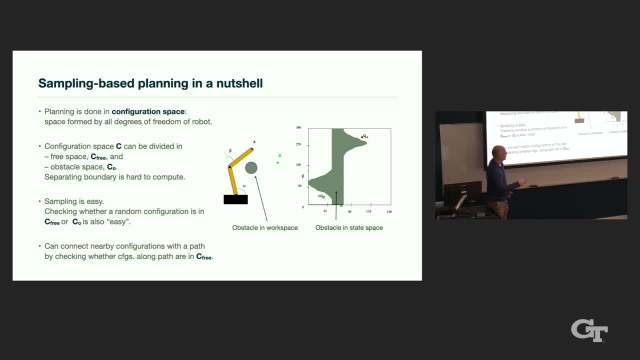 because there's an obstacle in between, But if we allow the arm to wrap around, so there's also interesting topology. essentially we can go from A to B by just sort of falling off the map here and well, or sort of go here and then come back here. 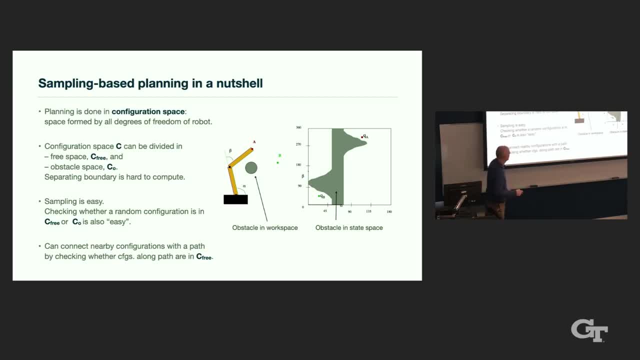 and then wrap around that way, right The angles could wrap around. The main point is that, even though computing this shape is difficult, generating random configurations is easy, just throwing points at the map, right, That's easy- And checking whether a configuration is in collision. 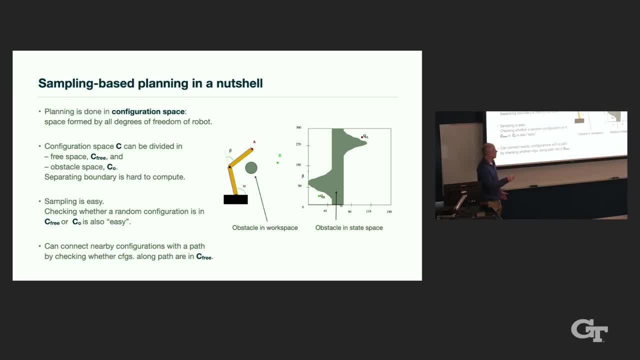 is also easy. We basically have to figure out whether two rectangles intersect with a circle or not- Also pretty easy. And connecting configurations to nearby configurations- essentially just doing linear interpolation and angle space- is also easy. So there's a number of operations that we need. 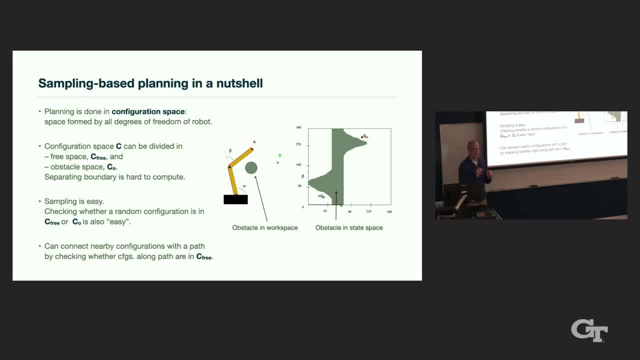 I'm kind of skipping over a lot of details, but just sampling configurations, checking whether they're valid and connecting them. they're all reasonably simple operations And we can combine these operations now to do actual planning. Just to give you another data point. 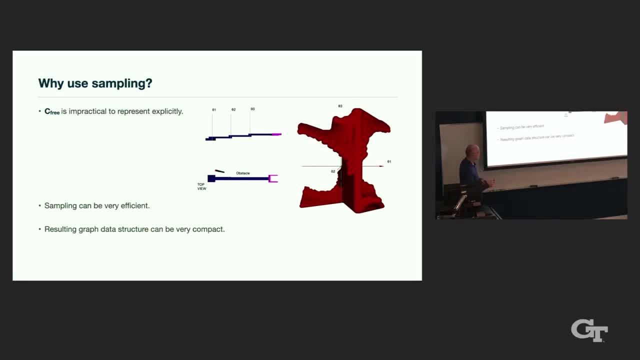 of why this might be a good idea. So this is a similar robot. Now it has three degrees of freedom. It's seen from the side, It's a planar manipulator seen from the top and there's one cylindrical obstacle. 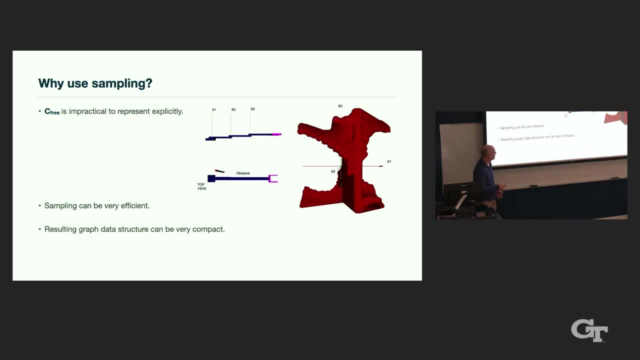 Really simple, the most minimal scene that you can think of, And this is already kind of the complexity of what this cylinder might look like in configuration space. It's very non-intuitive. You don't want to compute this shape And, in fact, the algebraic complexity. 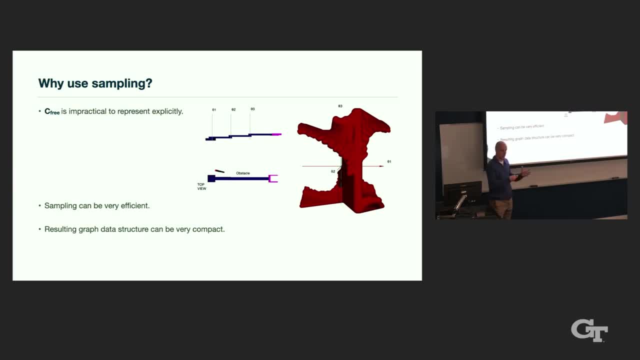 of this geometric object is what makes motion planning so hard. This computational complexity of this shape is what makes motion planning hard. Essentially, for an optimal path, you'd be touching these boundaries a lot, So you kind of need to know the boundary. So we kind of are going to bypass that optimality for now. 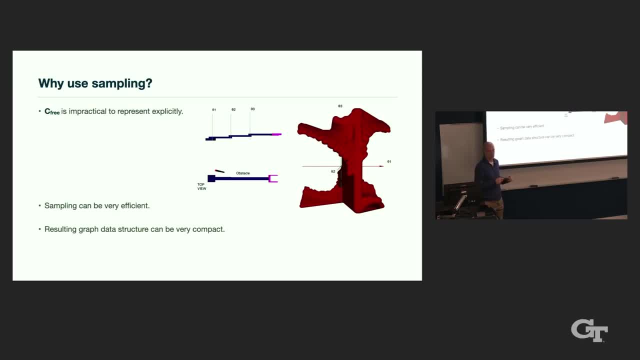 I'll come back to that later. I'll just say let's just compute a feasible path and not worry about computing this shape exactly. We don't necessarily want to sort of trace out the boundary So we could sample efficiently, construct a graph. 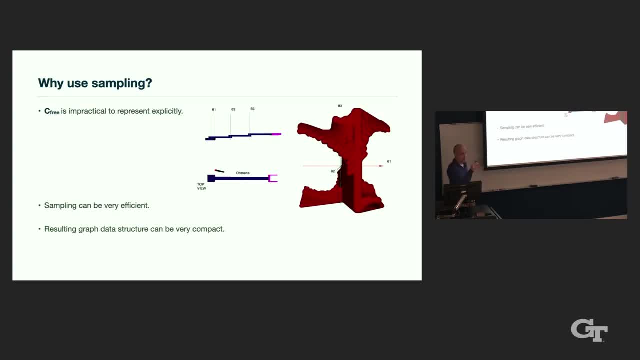 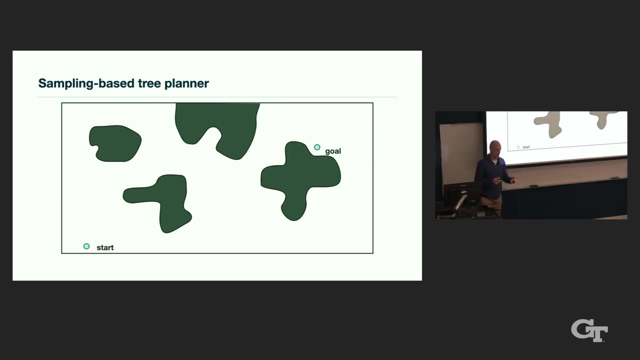 where configurations are connected to ones that can be connected with straight line interpolation, And this graph structure can be represented very compactly, unlike this really complex weird shape in high dimensions. So what might this look like in 2D? So again, imagine we have a 2D, a two-joint robot. 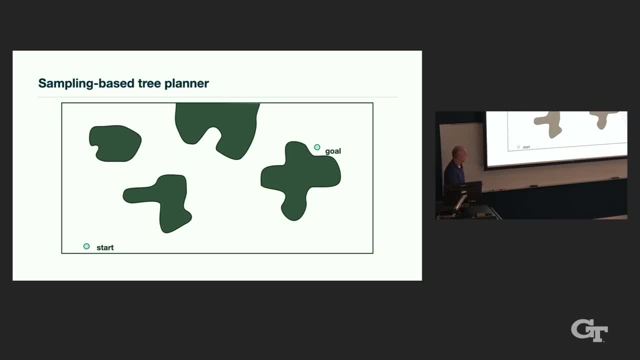 and we have. each dot represents a robot configuration. Let's say we start here, We want to go there So we could sample and construct a tree while we go along. So each time we select a node in our tree and randomly extrapolate from it towards the greater known. 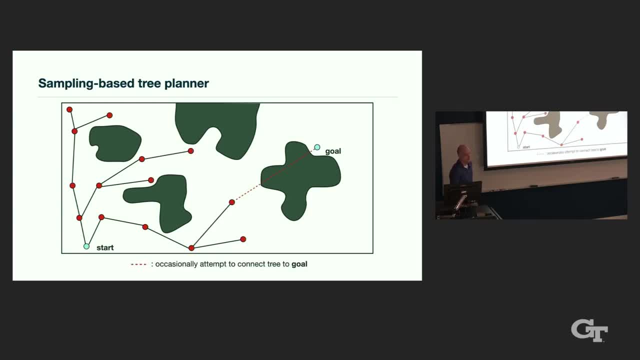 And then keep growing a tree that way. Every once in a while what we might do is try to find a node in a tree and connect it straight to the goal. Let's do joint interpolation and check along the way: are we climbing anything or not? 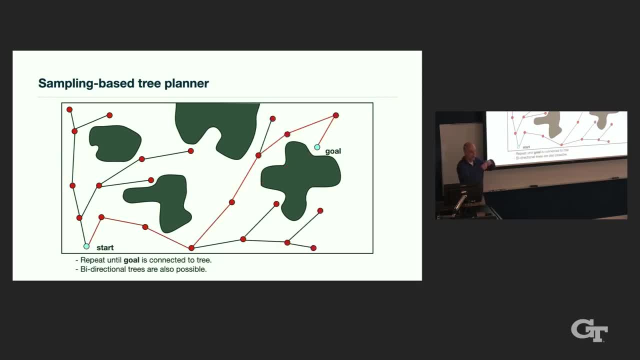 In this case it fails, And then we just keep going and keep growing our tree expanding everywhere, And there are lots of different heuristics to do this. I mean, one technique is just to sample uniformly everywhere in this space and then find the nearest node in the tree. 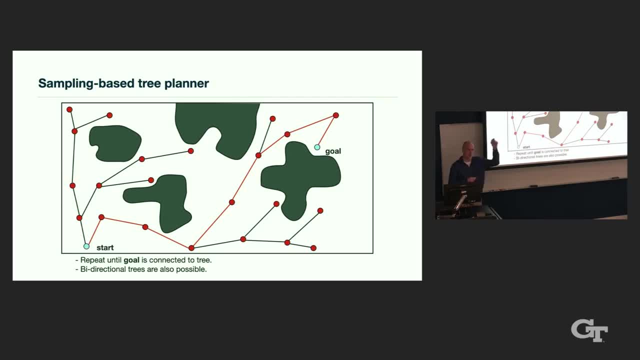 and then grow from that nearest node in the tree towards that random sample. But there's lots of other heuristics. For a while there was just. every robotics conference had like 10 new ways to do sampling, motion planning, And you still see new papers every once in a while. 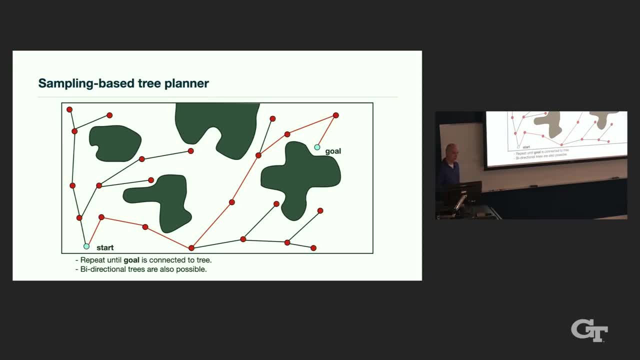 for slightly different problem settings depending on what kind of theoretical guarantees you care about. So this showing just one tree, many cases more efficient to grow two trees, one from start to goal and one from goal to start, And every once in a while try to connect these trees. 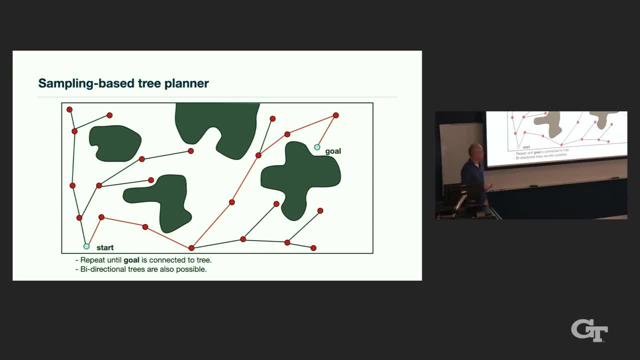 And you can just grow a graph. It doesn't have to be a tree. You can just basically try to connect every new node in your tree to every k nearest neighbors. Just do it. There's efficient data structures for finding nearest neighbors in space. 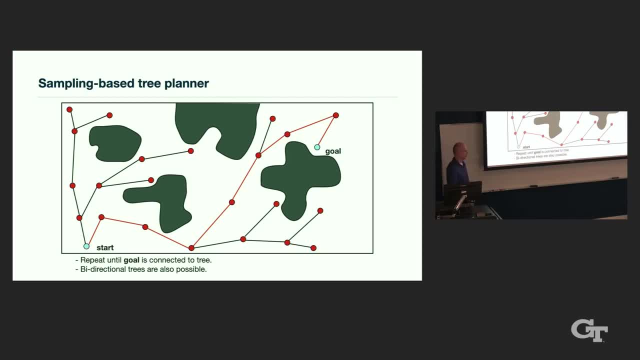 And we can just construct a graph if you want. And the graph has the advantage that basically it's useful, It's a reusable object. If your start and goal keep changing, then you can reuse the same graph over and over again. So this is this 2D example and I kind of pretend that we know. 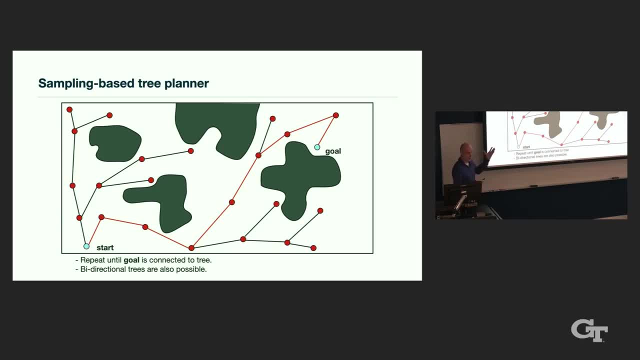 where these obstacles are. but what the point of the sampling is planning is that in general, we don't know what they are, And in higher dimensions we typically try to not compute that at all. So all we are doing is we don't know. 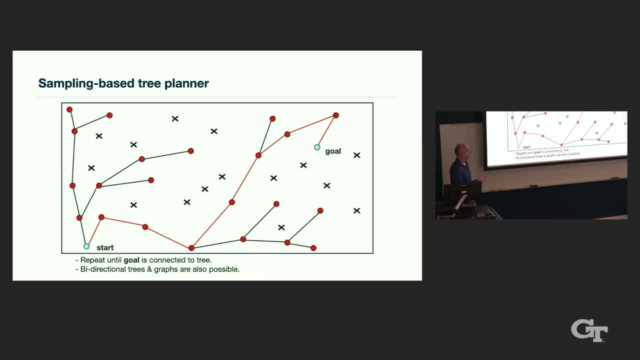 where these obstacles are at all. We don't know their shape, We just sample, And every once in a while we'll sample bad samples. We throw them away with these Xs and we keep the good samples only and keep growing our tree that way. 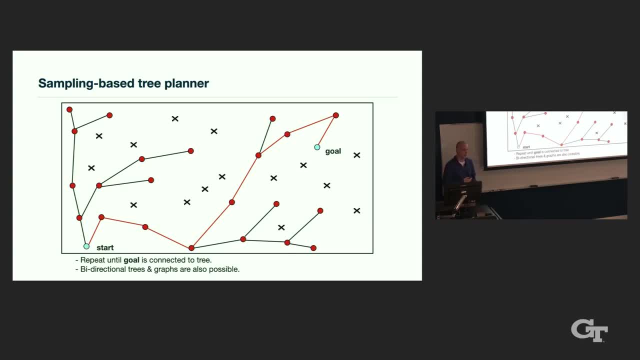 But we don't need to know anything about topology, necessarily. We don't need to know anything about the shape of the obstacles. All of that is left implicit and that's all fine. All we're doing is just sampling points and have some notion of distance and some notion. 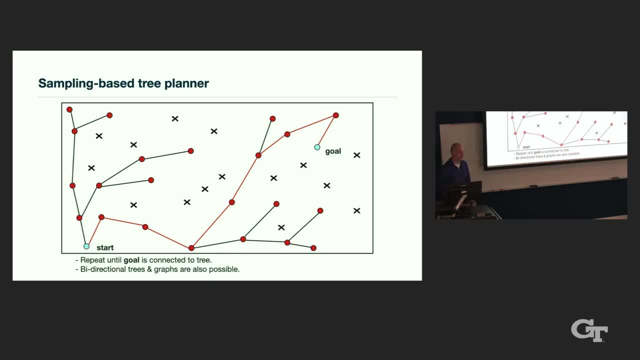 of interpolation and that's all. That's all we need. So it really doesn't matter if you're planning in a Klein bottle or a torus or regular Euclidean space. Sampling-based planning will just work. So yeah, I already kind of alluded to this. 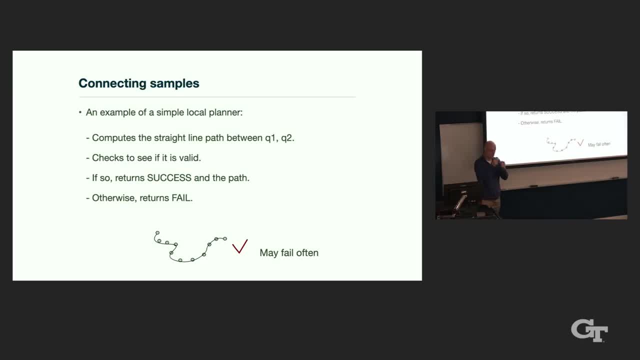 How we connect samples is basically: you find two samples that are somewhat nearby and compute a straight line path in configuration space and we just interpolate at some resolution and keep doing collision checks. And there are fancier ways to do collision checking where we actually have continuous collision checking. 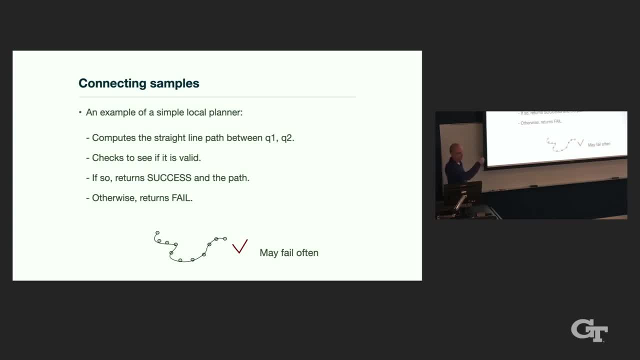 that automatically determine the step size. but the simplest way is just check at some resolution And if all checks succeed, then you say there's a valid way to go from A to B. You keep that edge. So, despite the randomness, we could still give some theoretical. 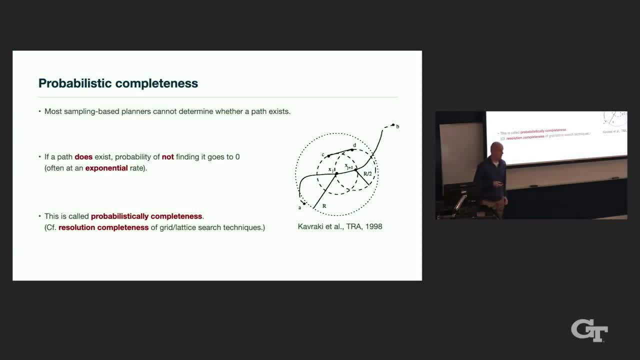 guarantees. So the one thing that we cannot do is determine whether a path exists or not. I'm sorry. whether a path does not exist, So it's semi-decidable. If a path exists, we will eventually find it, But if it doesn't exist, we won't know for sure. 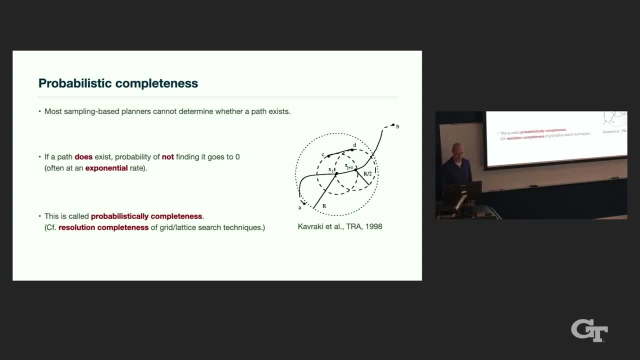 You can keep sampling and keep going forever without knowing for sure. But if it does exist, the good news is that we will find it with probability 1, often at an exponential rate- where basically, we're basically, as time goes on, the probability of not finding it. 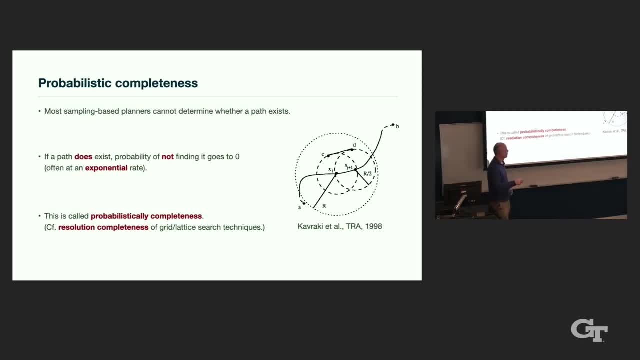 goes to 0 exponentially fast, And here's a sort of intuition for that. So let's say we have a path that goes from A to B And we know that. let's say there exists a path with clearance r for obstacles. 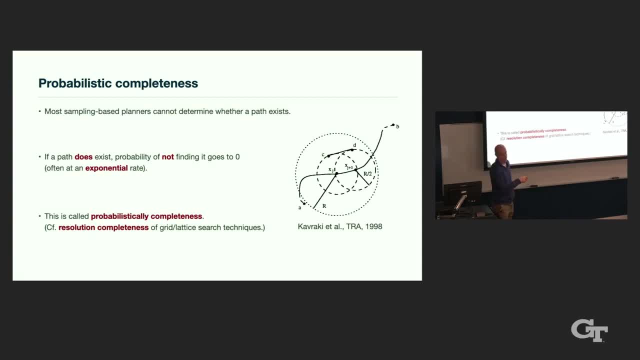 Somewhere along this path. we are like a distance r away from obstacles, So we can use that to essentially tile the path with little disks or spheres in higher dimensions of the radius r And inside that each sphere we can, we can make smaller spheres of size r over 2, spaced apart. 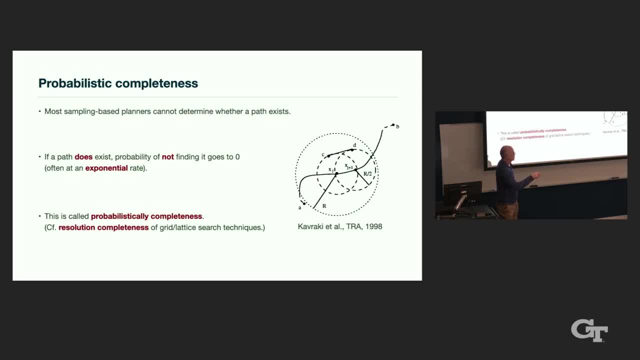 at distance r over 2. That means that from any ball we can connect to any other point in that ball. So as we keep sampling, eventually we get sort of samples inside each of these balls. So the probability that basically one of these balls 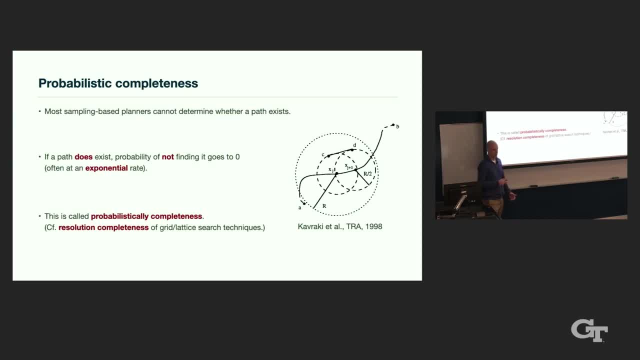 will remain empty. as we keep sampling, more and more goes to 0 really quickly. So it's just a matter that there's a non-zero- yeah, a finite- probability of finding a hit in each ball And, as time goes on, the basic, the probability. 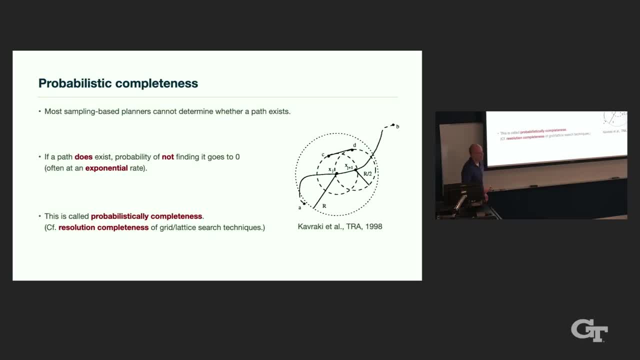 of not hitting any. all of these balls goes to 0 really quickly, So it's a really quick intuition for it. There's more details to the proof And this is, you know, proven a long time ago by Lydia Gavranki. 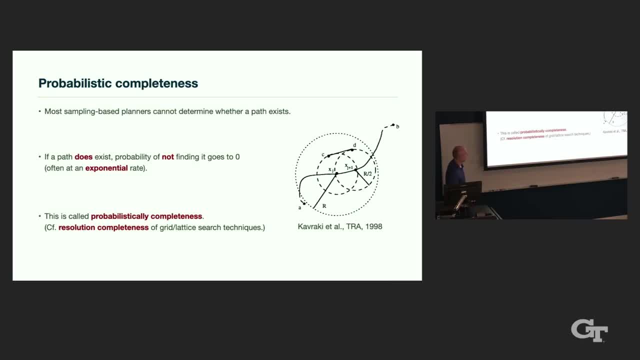 And this is the notion of probabilistic completeness. It is very different from the traditional completeness and also different from resolution completeness. So with grid-based search like A star and variance, we decide some resolution beforehand And we have to kind of decide what the resolution should be. 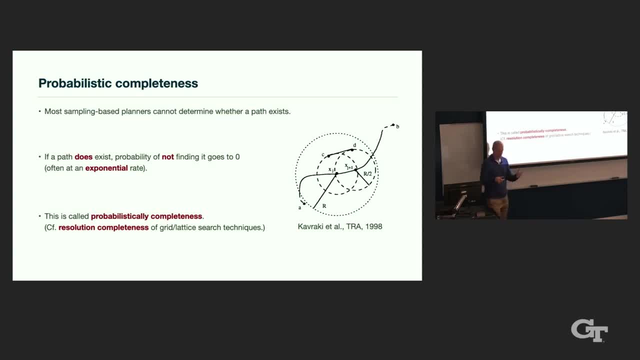 for shoulder joint versus wrist joint or however you want to discretize your space, which is non-trivial. but you basically pick your resolution beforehand and then do your search And, given that resolution, you might find an answer. But if the resolution was too coarse, 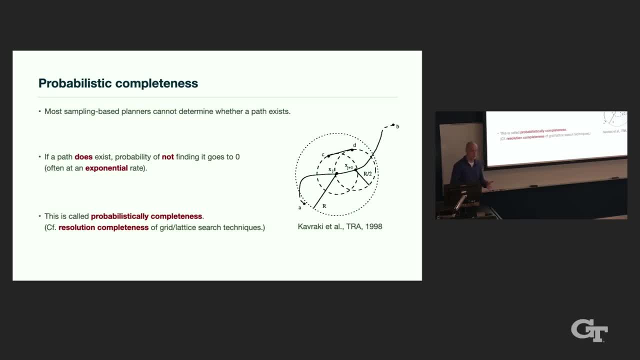 in any one of your dimensions, you have to refine and do it again, And here we don't have that problem of having to refine, We just keep sampling and we don't have to start over again. So this, what I just presented, is basically a way. 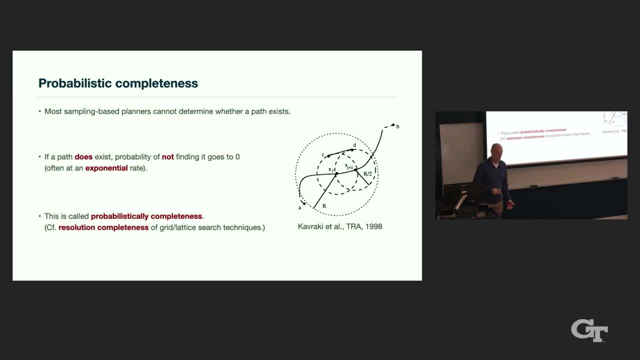 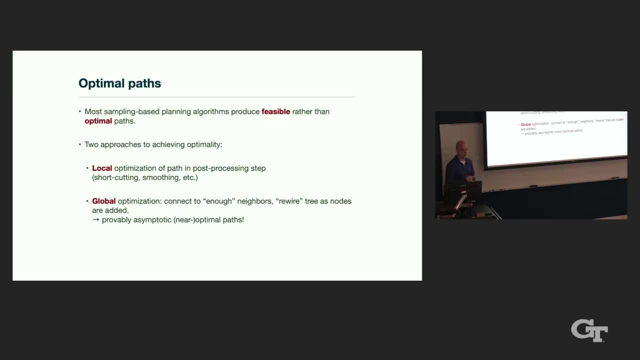 to get feasible solutions. In many cases we actually do care about optimality and we like to find something that is close to optimal. Optimal can have different meanings. Usually people assume shortest path. whether that's useful it's debatable. because shortest path in joint angle space. 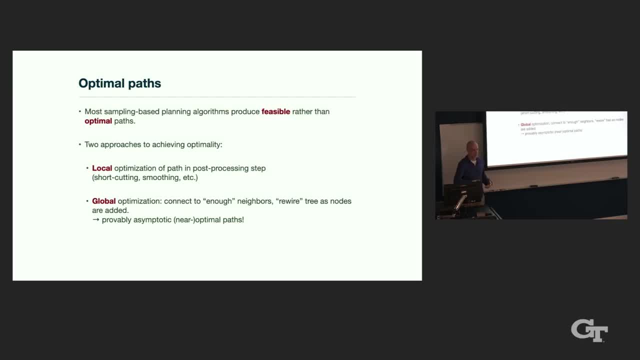 doesn't always mean shortest path. Usually it doesn't mean shortest path in the workspace by any normal measure Like swept volume or end-effector displacement. But yeah, you can come up with your notion of optimality and optimize it with respect to that. 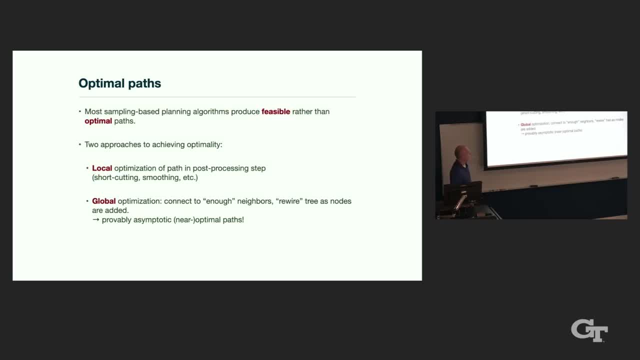 There's two ways to achieve optimality. The simple way that people have used for a long time is local optimality, that we compute a feasible path first and afterwards. we just perturb the trajectory. We can do some sort of short-cutting. 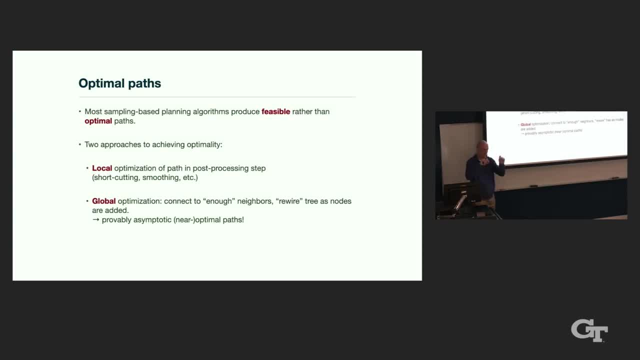 where we just sort of see if there's a straight line that connects different points along the trajectory, to see if we can cut out some part of the trajectory, Or we can use some other kind of optimization approach where we just iteratively move the trajectory points around. 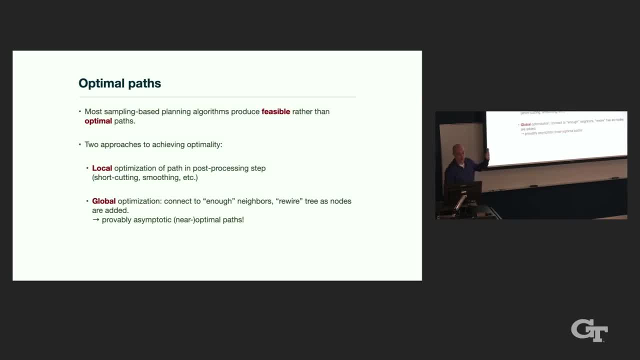 until we settle on the local minimum. That's typically very fast and for the longest time people were satisfied with that. It seems good enough. It was fast and basically people focused on the harder problem of finding a feasible solution In high-dimensional space. that really. 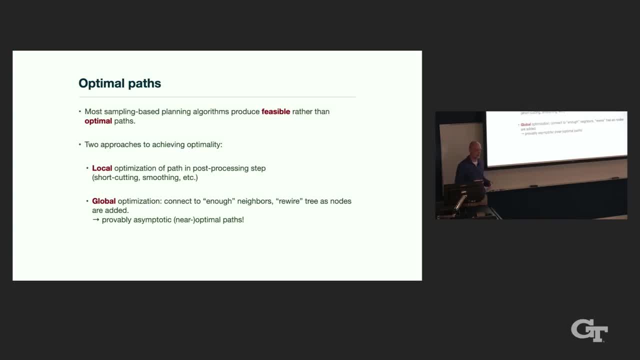 is the harder problem of finding any solution at all. And then locally refining. it was an afterthought. We have our bag of tricks, We apply that. That works fine. Eventually it was shown that actually with some tweaks to the algorithm that seemed small. 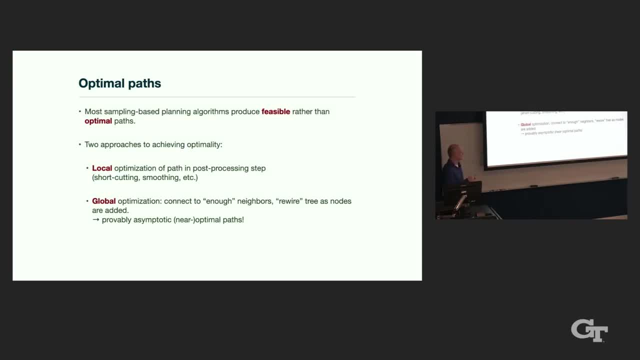 and to prove that that was optimal was really hard. actually, you can get global optimization as well. So when we construct a tree that I showed before, every once in a while we need to connect, rewire our trees or rewire certain subtrees that are. 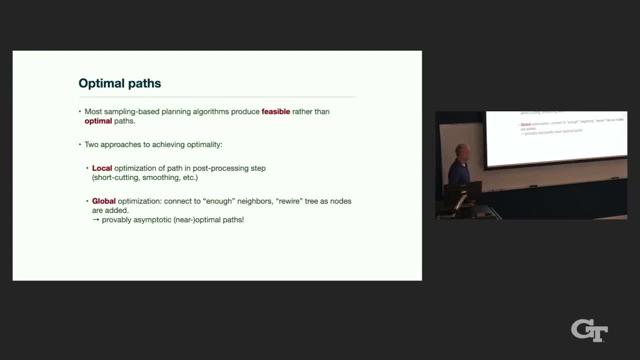 connected to another part of the tree and maybe do some extra bookkeeping, And so there's relatively small adjustments but huge proofs. to prove that it's like, I think, the original paper from Sertac, Karaman and Frizzoli of like 80 pages or something like this: 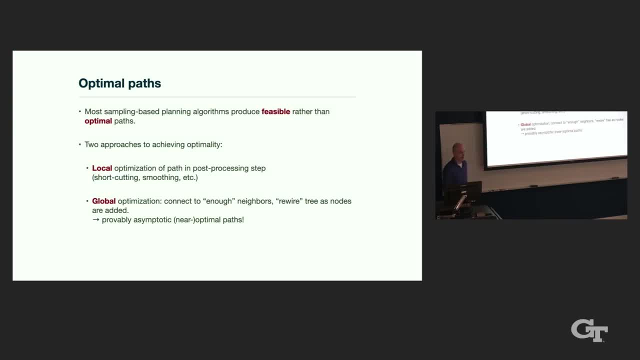 that slight changes to a very basic algorithm result in optimality, But it can be proven that this actually results to optimal. It will also be proven that the original process is guaranteed to be not optimal. so not just that, details do matter. So that's the basics. 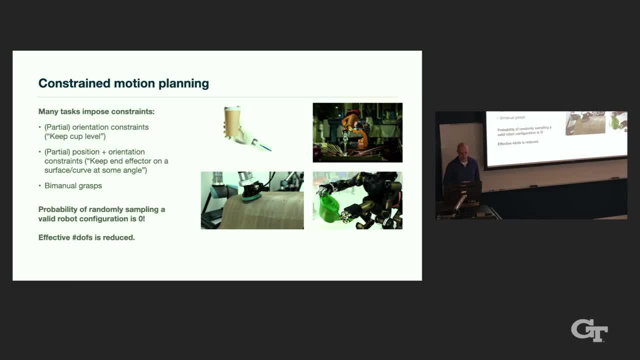 OK, That's the basics of sampling-based motion planning. Now I want to move on to sort of constraint motion planning where it seems like none of what I just talked about is going to work. So in practice there's lots of task constraints. 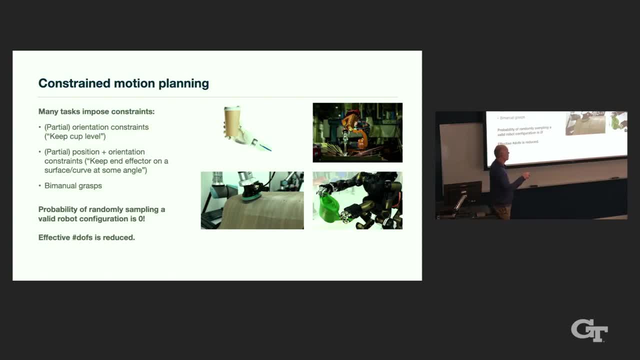 Whenever you try to do things with manipulators- things like keep a cup level or following some sequence of well patterns or sanding a surface or doing bimanual manipulation- where we're holding things with two hands at a time- we're losing. 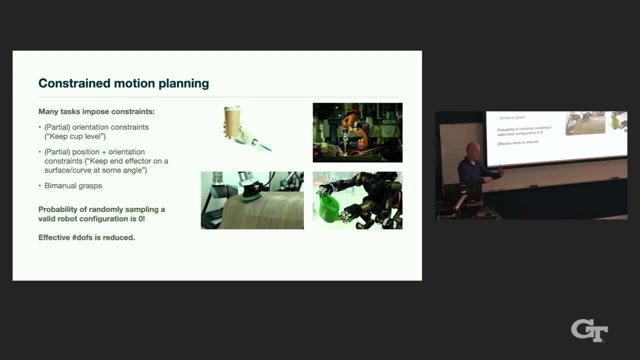 degrees of freedom because of the task, And we have our degrees of freedom on a mechanism, but the task is sort of removing some of them. We cannot independently change each degree of freedom. So what that means is that if we randomly sample configurations, 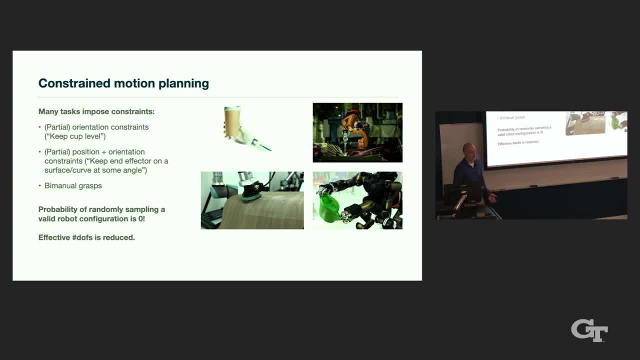 the probability that our sample configuration is valid and basically holds the cup level or is on the surface while sanding is zero. So sampling seems like OK, we've lost everything, We can't do anything anymore. Or it's not entirely true. 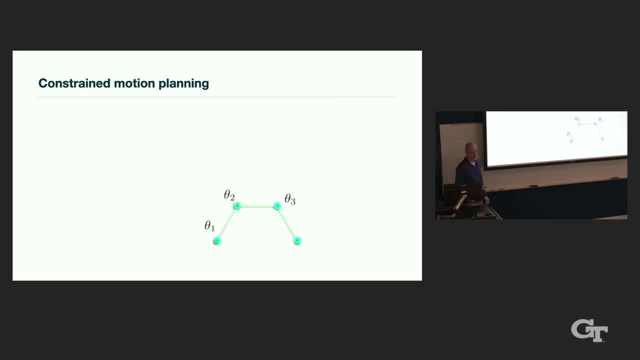 So let's look at a more illustrative example of what constraint planning really means. So here we have a three degree of freedom planar linkage, So we have a three dimensional configuration space And let's say we want to find a path between these two. 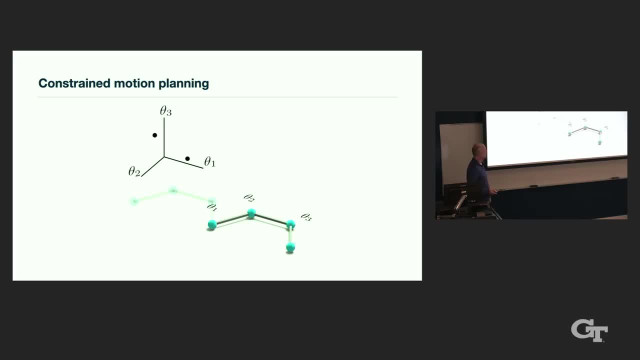 configurations, But we force the path to lie on a curve. We just want our arm to move along the arc of the curve, And what that means in configuration space is: now we have a reduction, We have a reduced configuration space. So instead of a three dimensional space, 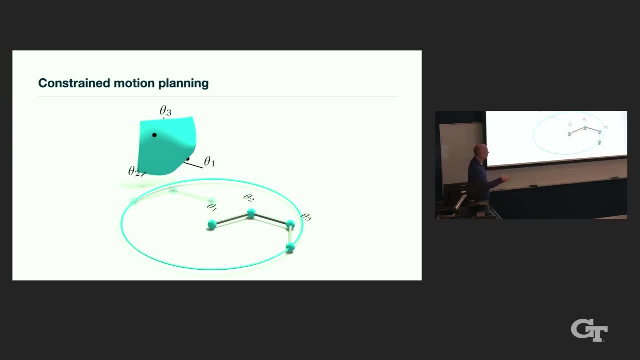 now we have a two dimensional space. We remove one degree of freedom with this constraint and we have to move along on this surface. So one possible path might look like this: It's tracing out a curve on this circle and it's also tracing out a corresponding curve. 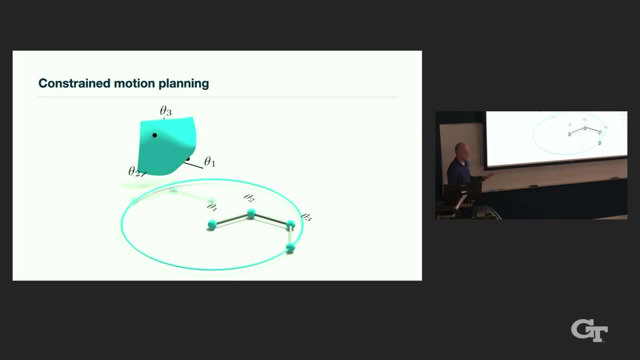 on the surface. So that's effectively what we're doing with constraint motion planning. We have the constraints, introduce this lower dimensional manifold and better than the high dimensional space. The high dimensional space is the original configuration space But effectively we were planning on this surface. 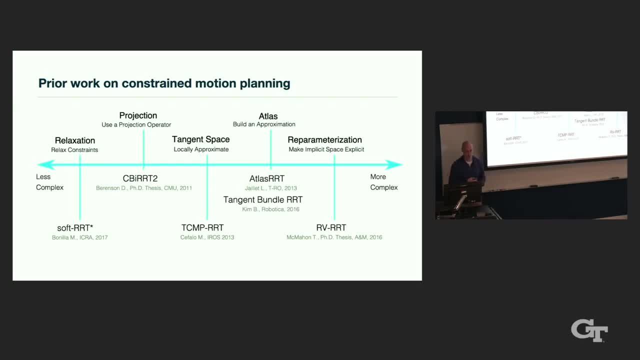 So lots of people have thought about how we can deal with this. Usually people have augmented existing sampling based planners in various ways with additional bookkeeping to make sure that the samples land on this manifold. So towards the less complex side of dealing with constraint. 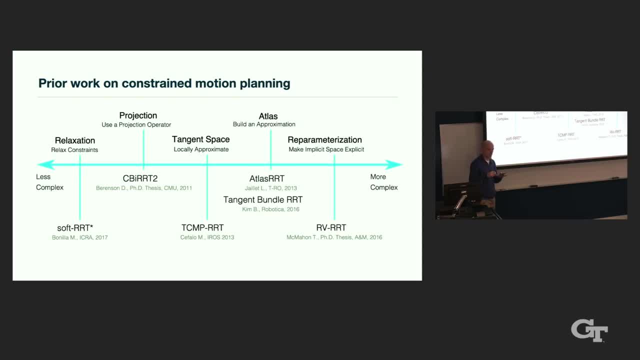 is constraint relaxation, Essentially just pretend that we don't exactly have to be on this lower dimensional manifold. Let's just inflate it a little bit And now we have a non-zero measure volume that we can sample from. So we still can sample and pretend. 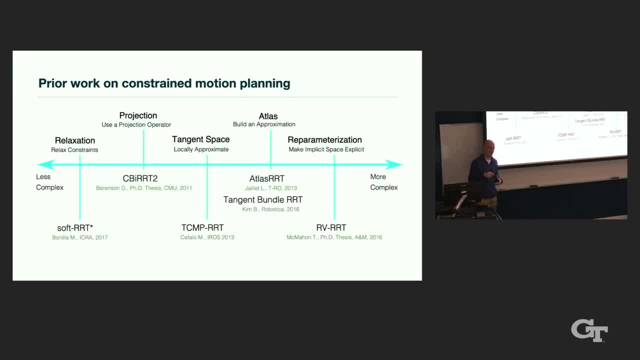 that everything that's not inside this inflated manifold is in collision. Everything that's inside that manifold that's now been inflated a little bit is valid. That's the simplest trick, Basically. just don't deal with it at all, Just fudge it a little bit. 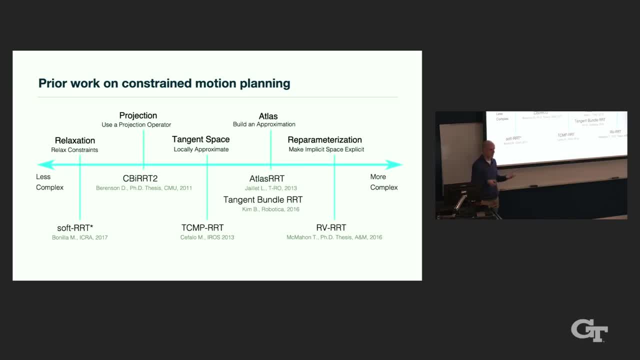 Then you can use things like projection. We use something like: we have an implicit constraint function. We use Newton's method that if you're off the manifold we minimize it until we are on the manifold. And then there are fancier tricks where we're actually 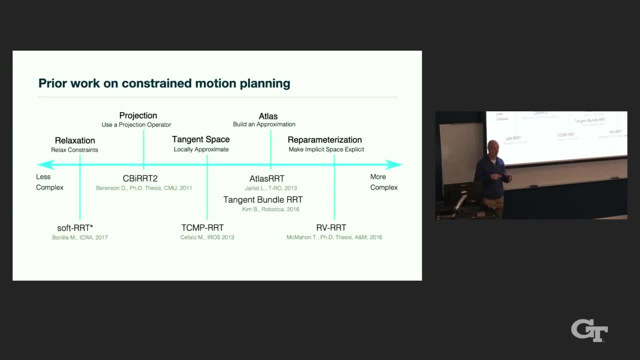 building an atlas. so we're constructing tangent spaces to our manifold and keeping track of that And as we walk along the tangent space we keep track until we fall off the tangent space and recompute the tangent space and keep going. So there's lots of bookkeeping over here. 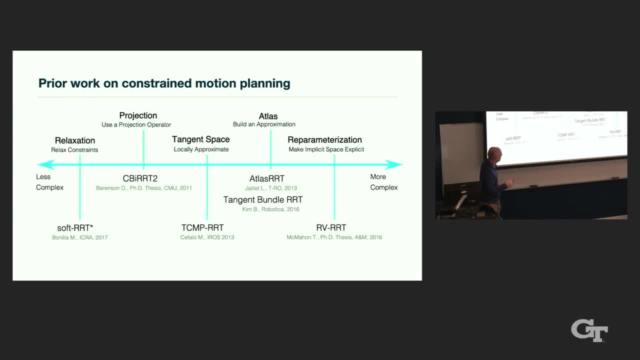 But in some cases it actually is worth it compared to the simpler techniques. And, of course, if you can just re-parameterize, instead of having this implicit manifold, have an explicit manifold that you can directly sample, then that's probably the better way to go. 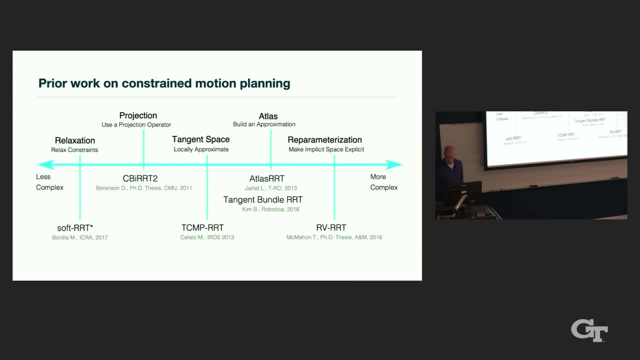 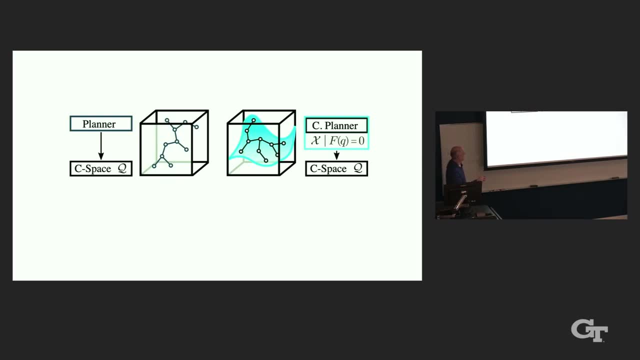 But in many cases you cannot solve for that explicit manifold. But roughly speaking, these approaches would treat the problem like this. So we have our configuration space where we grow a tree with a planter And now we can configure it. We have some constraint motion planning. 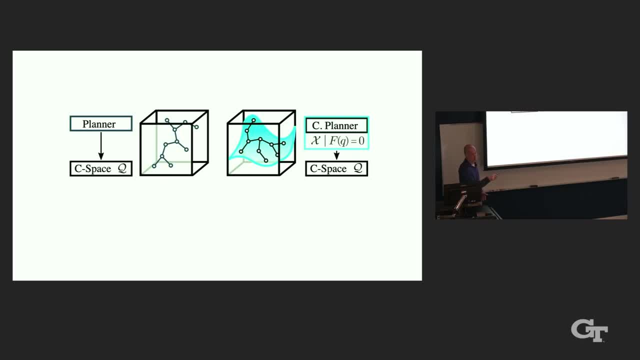 We have some special planter that's been modified to only sample things that are inside this manifold and still from this configuration space queue, And it turns out that this may not be the best way to think about it because it kind of limited the way people 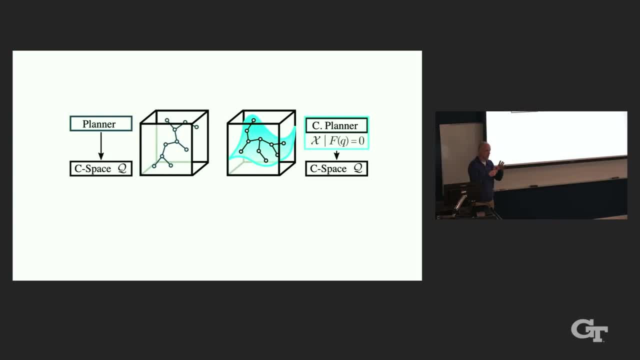 were thinking about which planters we could augment And there was all kinds of sort of inelegant solutions that were required. You know, it didn't have the separation of concerns because there's one way to sort of do this high-level reasoning about where 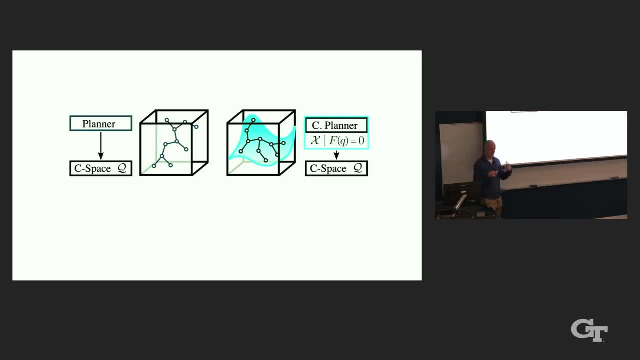 to search next is exploration exploitation bias that you always have to trade off, that you have to deal with in any kind of search and planning. You have to figure out what's the most promising way towards the goal and where should we search next to ensure completeness. 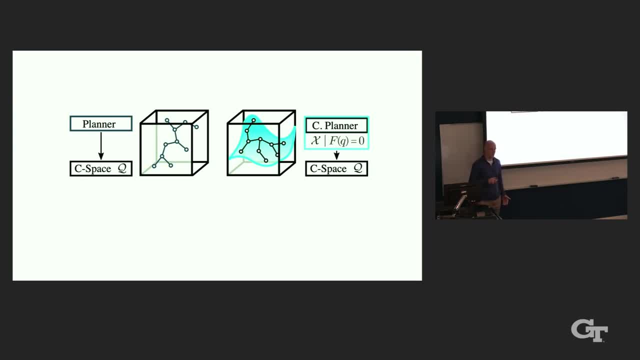 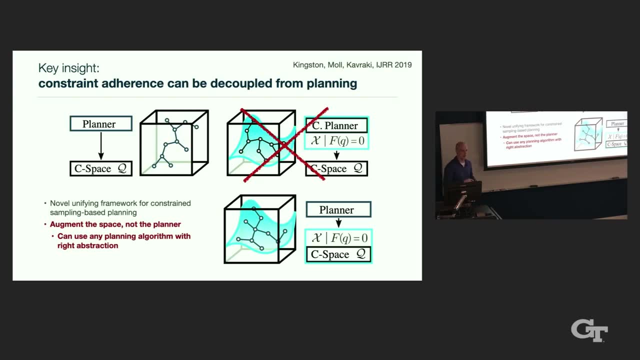 And that seems completely separate from how should I sample constrained configurations? So what we realized is that it's much better to kind of create an abstraction that we sample over implicit spaces. So we have our set of x, where all the configurations where f of q equals 0. 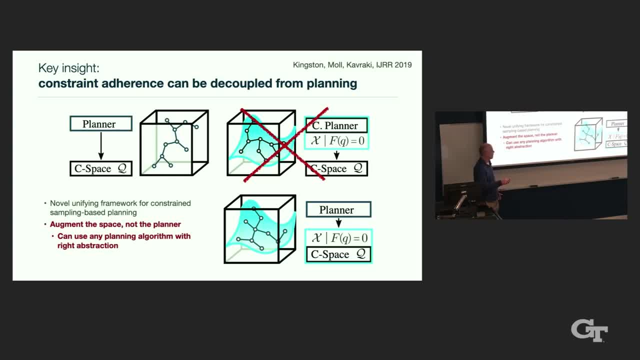 And this is now part of this space. So we really have a plan that operates over this new kind of space, And all it knows is that this space supports interpolation and it supports sampling and it has a notion of distance. It's not Euclidean distance and it's not 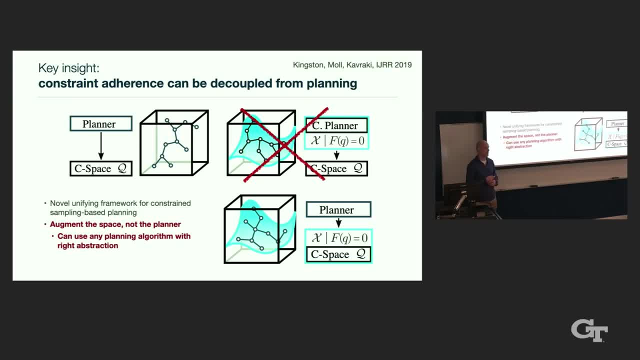 standard linear interpolation. But the plan doesn't care? Sure, It shouldn't care. And now that we've decoupled these things, we can choose them independently. We can play with our heuristics for how to search high-dimensional spaces independently. 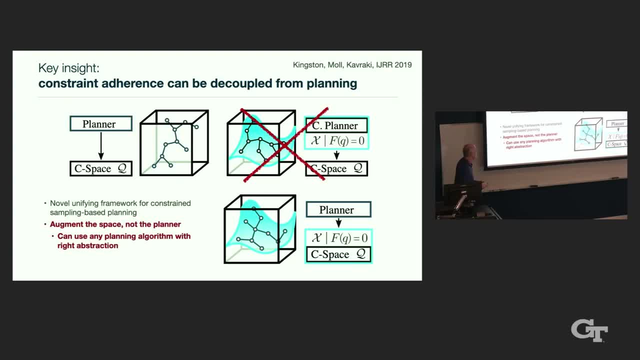 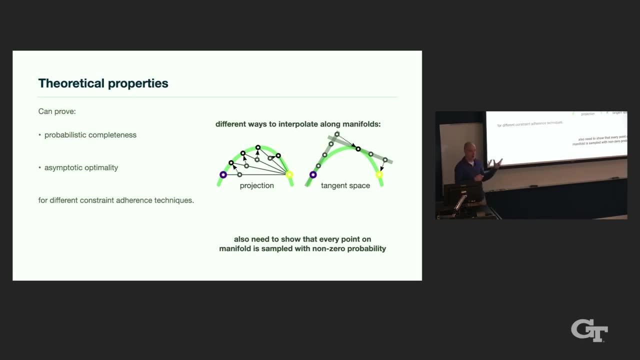 from how we deal with these constraints. So, yeah, we need to augment the space, and not the planner, to deal with constraints. Now that we've decoupled these things, we wanted to go back to these original papers and say, oh, Can we really mix and match any of these previous techniques? 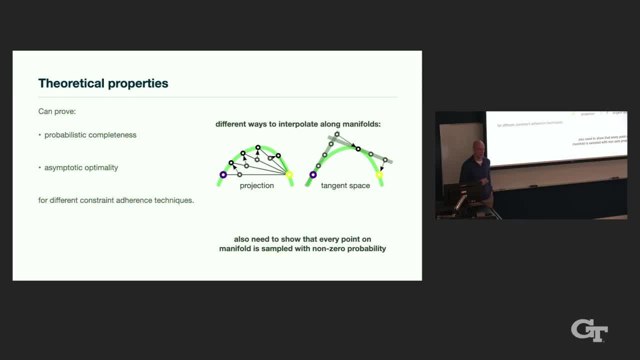 that were tied to a planner and show that it really isn't tied to the planner and show that you can really throw any planner at it and use projection with any planner you want and still ensure that you have completeness and optimality, Because previously these proofs were: 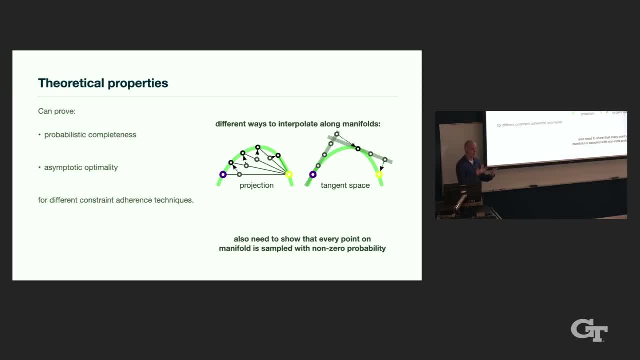 specific to that combination of planner and constraint satisfaction. So if we decouple it, well, who knows, Is it still true that we have completeness and optimality? If we decouple it, Can we somehow use projection or tangent space methods for a new planner? 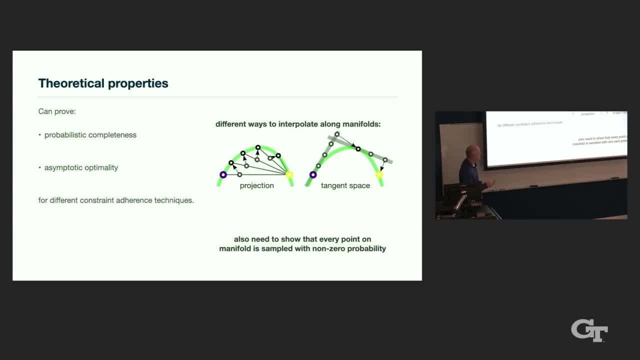 And we can show that. yes, this is still true. So, projection: the simple idea is that you interpolate from A to B, take a small step from A towards B, and then you use something like Newton's method to take that f of q constraint function. 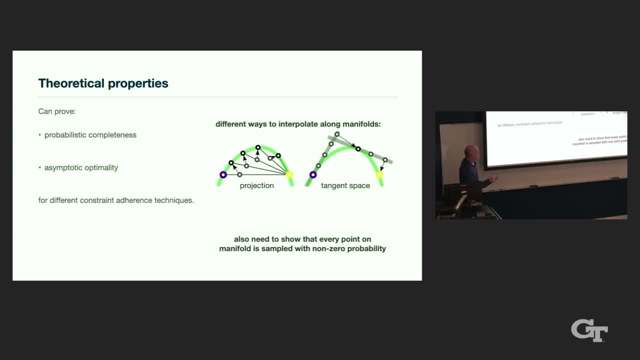 and follow the gradient of that until you're back at 0 and then repeat, And that way you can kind of walk along a manifold And tangent spaces. you clearly construct tangent spaces And you keep walking along that tangent space until the error is too large. 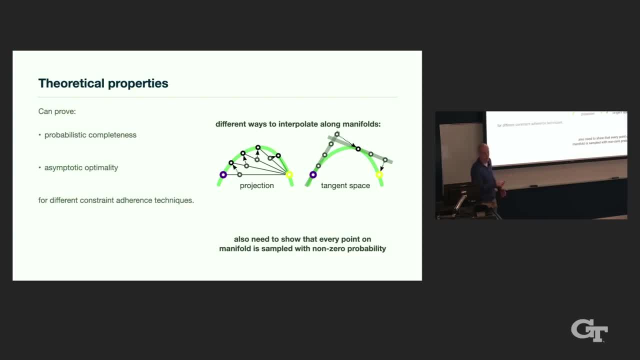 And then you recompute a tangent space pre-projection and keep going that way. Those are two simple techniques And they can be combined with almost any planner, And you can still show that you didn't lose anything. You can still show that you have completeness. 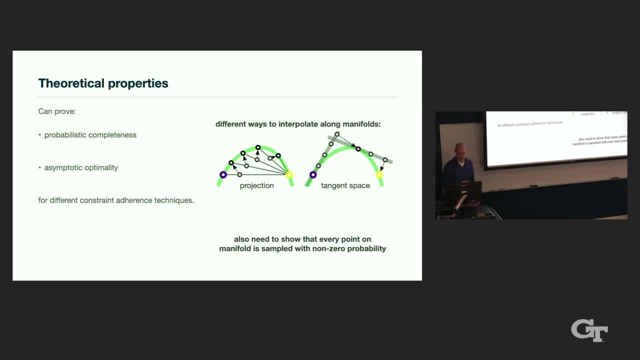 with the right planner You can still show you have optimality. There's some technical details showing that each point is sampled with non-zero probability And the simplest way to see that is that let's say you have a torus as your constraint surface. 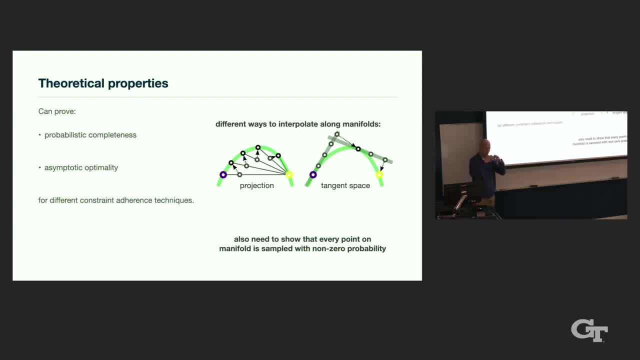 as the hole in the surf embedded in 3D. As that hole in the middle gets smaller and smaller and the embedded space gets larger and larger, the probability of sampling in the middle goes to 0, especially if that hole kind of shrinks up. 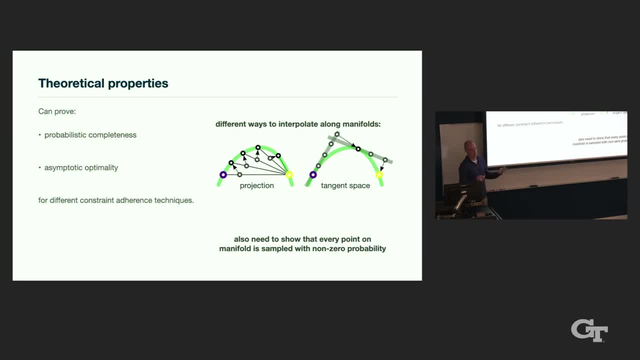 So if the path requires you to go through that hole, basically you're out of luck. So you kind of have to make some assumptions that when you're projecting onto that, manifold this constraint, manifold, every point needs to have some non-zero probability. 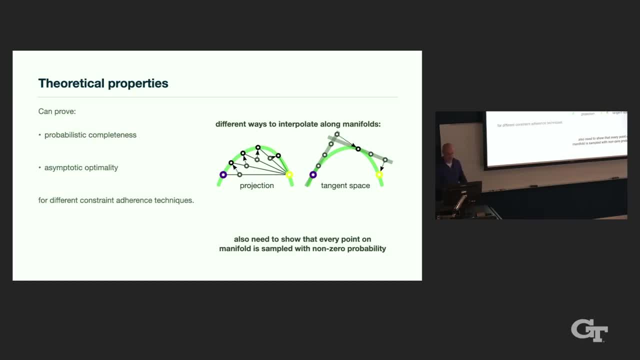 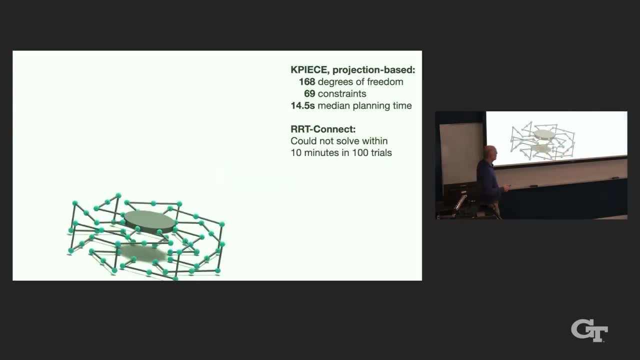 So you can show that you're projecting onto that surface, But under those mild assumptions, you can show that these properties still hold. So what does that buy us? Well, now that we can choose independently, we can take some unusual combination of planner. 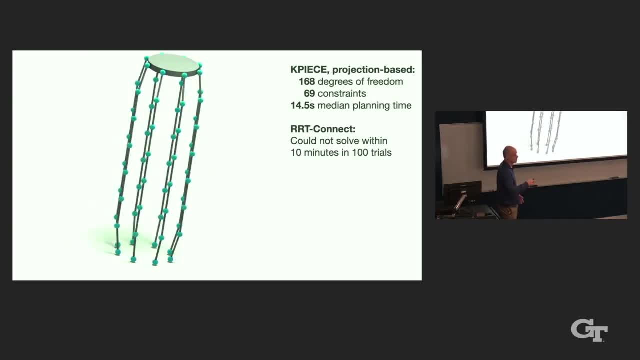 and constraint combination. In this case we take kps, which is kind of an involved planner Normally you wouldn't think of it's already doing a lot of algorithmic work. You wouldn't think of let's add something complex to it. 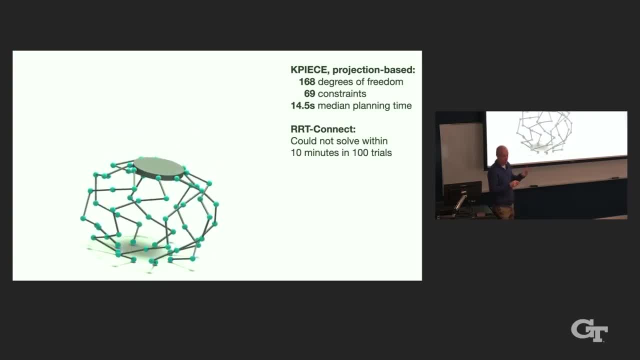 an already really complex You wouldn't think of. it's already doing a lot of work, But in this case, now that we decoupled it, it doesn't matter. And it turns out that this mechanism, which is kind of a toy example, it's using these linkages. 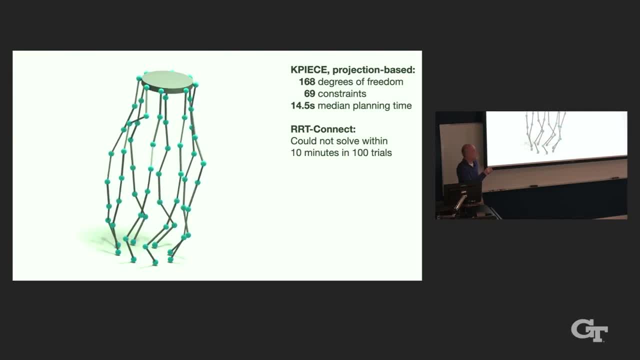 with spherical joints and modeling it with these points, with distance constraints, And these points are all attached to these disks And of course, that's how we get to lots of degrees of freedom. lots of constraints, significant planning time, but not terrible given the high number of degrees of freedom. 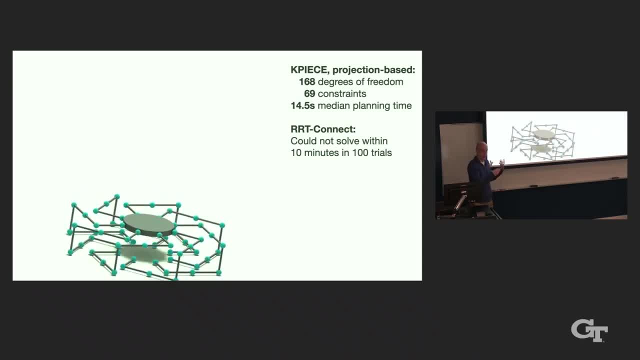 But if you use some version of RRT- which is what most previous work used- to augment the constraints, you couldn't solve it at all. Some of these heuristics do matter a lot for constraints, And this is not to basically say that RRT is a bad planner. 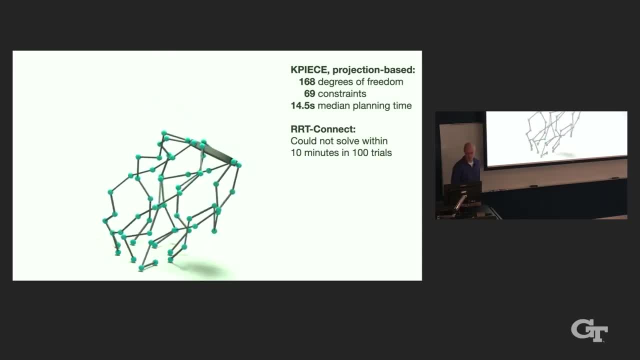 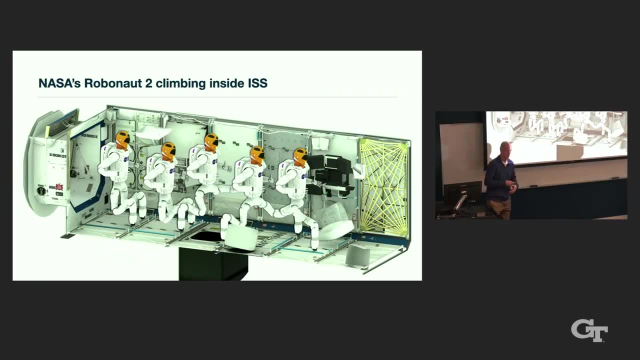 It works really well in many cases, But for this particular instance it was not a good fit. Of course you may not care about that particular toy example. It's just sort of an example to show that things can get really bad, but it's. 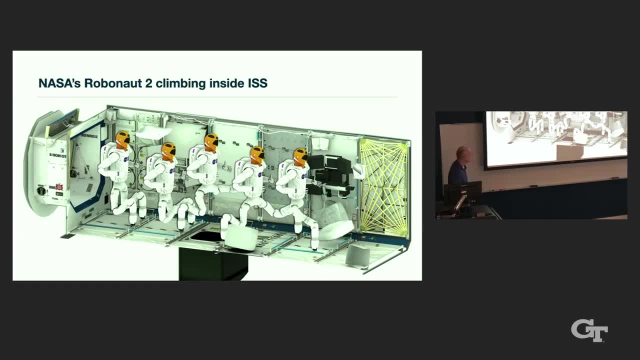 unsolvable one way and really fast another way. What we do care about is examples like this, where we're working with NASA Johnson Space Center on trying to climb across handrails And this seems like oh a nice open environment. There are hardly any obstacles. 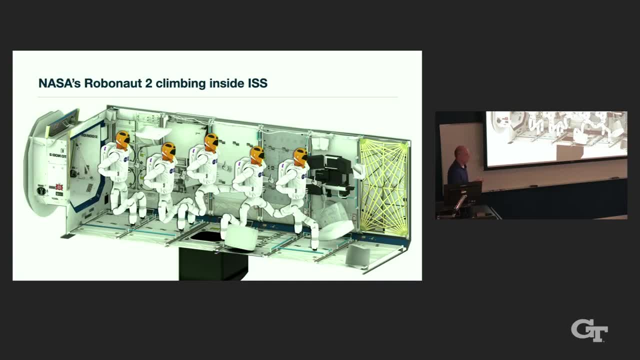 How hard can it be? But again, there are lots of constraints because we basically have to keep this torso upright, for not very technical reasons, I mean, there's no up in space so you can walk on the ceiling. But NASA really doesn't like it. 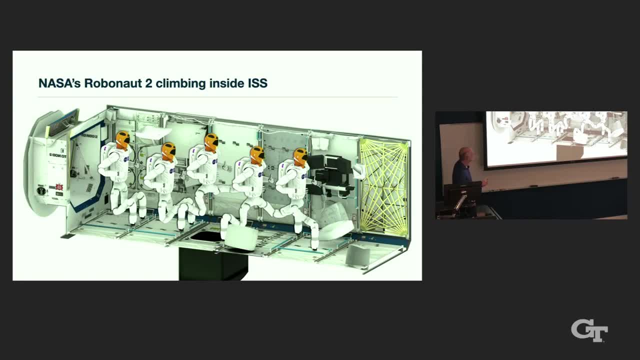 They really want their robots to walk on one side And also just do experiments on Earth. There's a gravity offload mechanism, but it only works in one direction. It doesn't compensate for force, not for torque, So we have to keep the body upright. 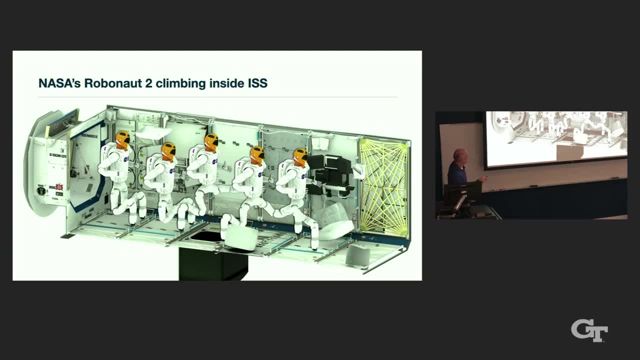 We have the legs attached to these handrails And the robot is really tall. It's hard to see, but it cannot stand straight up, So it has actually a very limited space and it needs to do these really weird spider-like motions to walk across handrails, even though it doesn't seem. 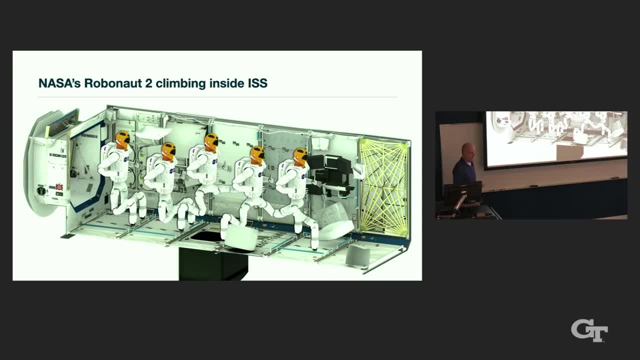 like. the environment is very cluttered And of course the NASA people try to just use pure IK to say: why do you need planning at all? Just take two feasible IK solutions and use some version of IK-based techniques to just go from one post to another. 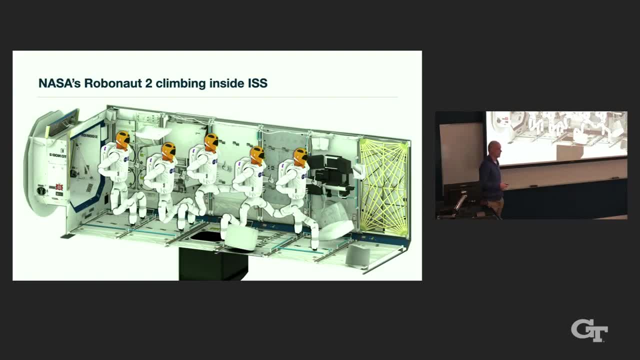 do some sort of interpolation Doesn't work. You should say what IK means. Oh, Sorry, Inverse kinematics: Yeah, Sorry, Thank you. Yeah, So there's simpler techniques that you can imagine being useful in something without too much clutter. 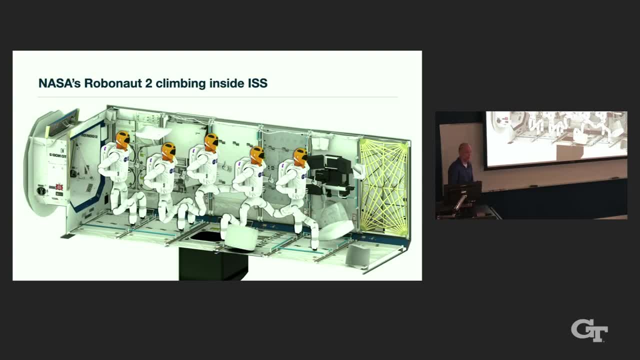 That you think. oh, we use the inverse kinematics of the system to sort of move around locally And surely that will get us across handrails from one handrail to the next. Doesn't work, There are too many local minima. 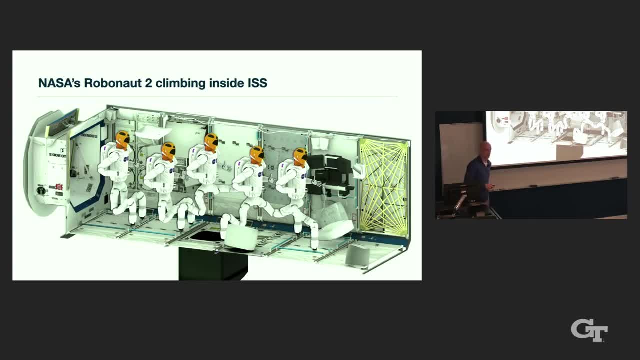 You reach too many joint limits, There's all kinds of reasons that it doesn't work. So you really do need planning, And this robot has 30-some degrees, Some degrees of freedom. You don't plan for all of them at the same time. 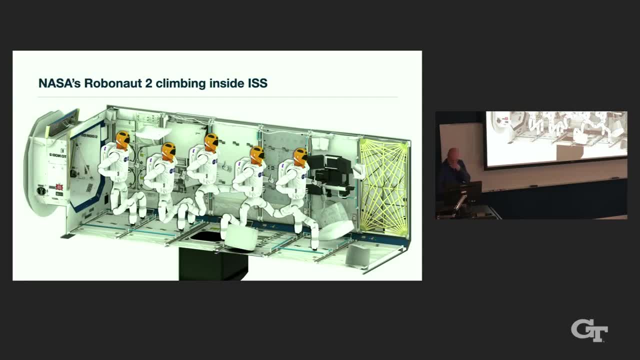 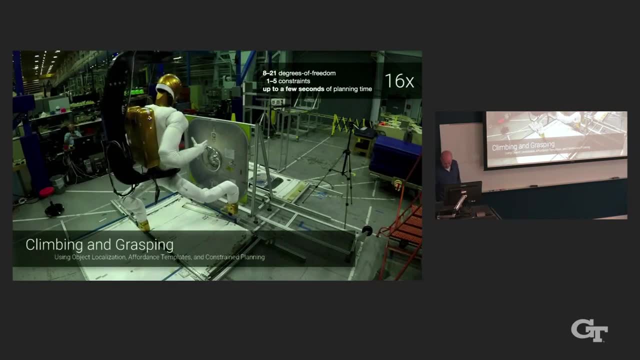 Typically you plan only for the legs or only for the arms, But the example video here showed that. I showed this before, But now we have some context for appreciating the difficulty when we're, for instance, opening this door. Let's see. 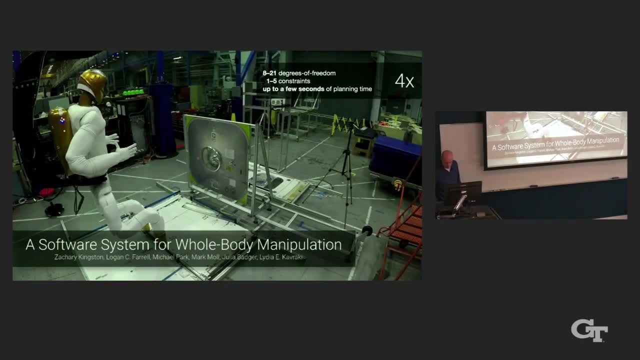 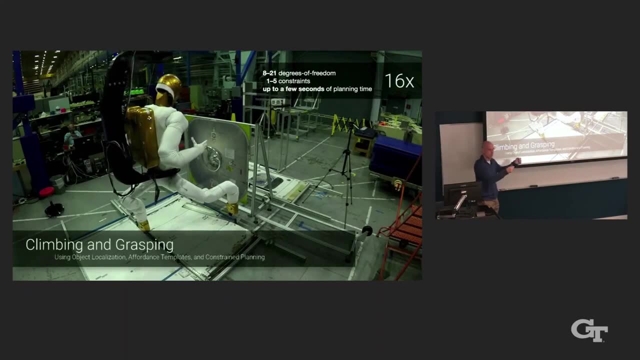 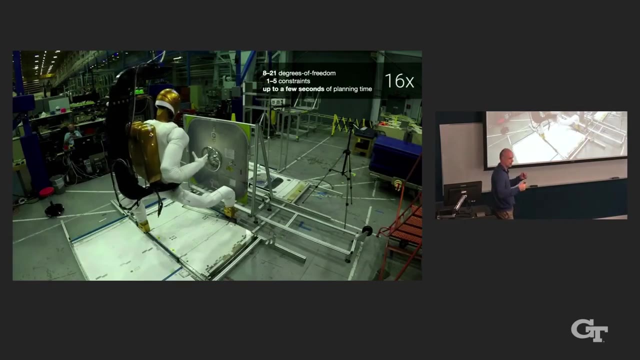 How do I? Oops So when it's opening so it steps from handrail to handrail. Eventually it turns the valve. When it slides open this door it's having. it has two feet attached to the handrail and needs to move its body. 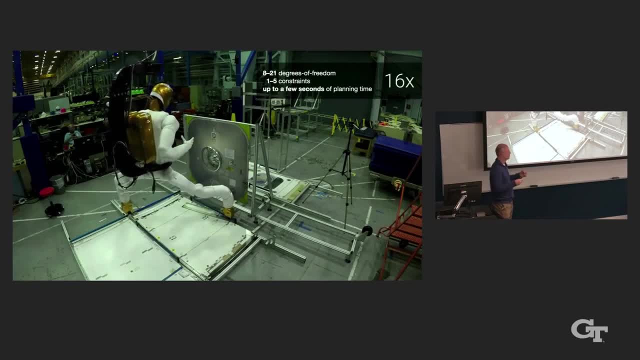 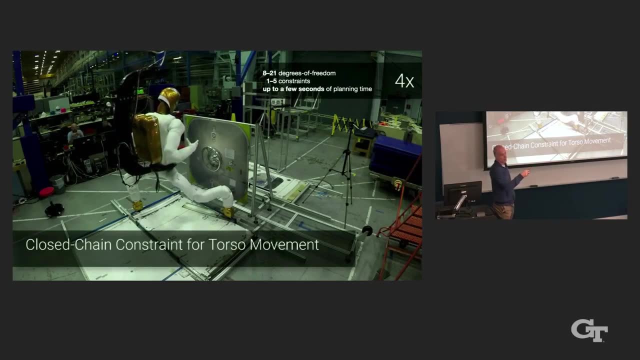 So they have these closed chains that really reduce the degrees of freedom and move its hand. So each step, we're planning for different numbers of degrees of freedom. The highest number is 21.. When we're opening this door, we really are planning for 21 joints. 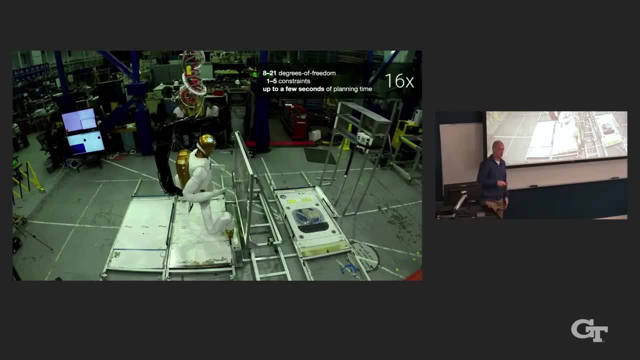 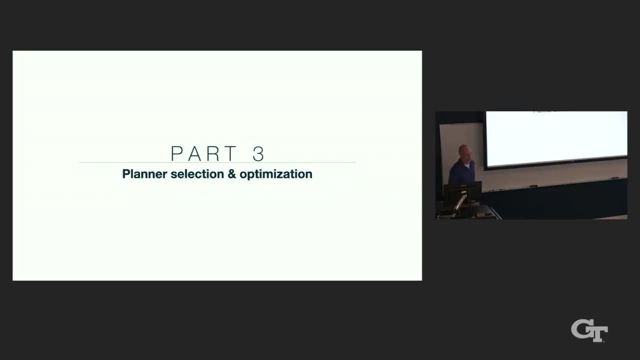 And we have lots of constraints, And it still takes only a couple seconds, which, compared to execution time, is nothing. You see, this is sped up heavily. So execution time is now the dominant factor, not planning time. All right, Now I wanted to talk about something really practical. 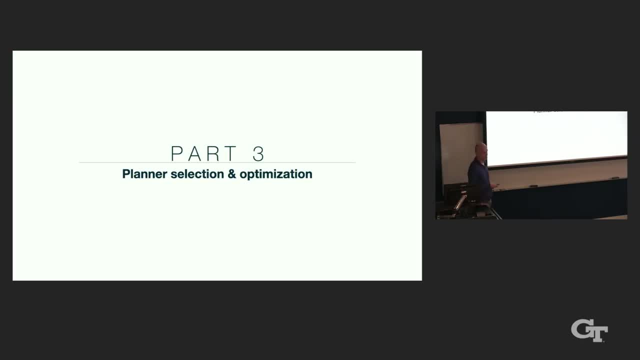 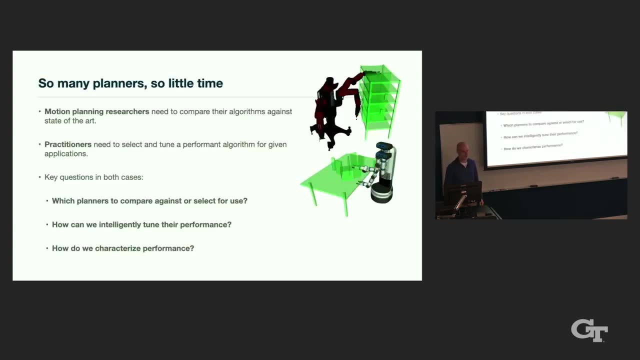 And I think it's maybe also important lessons here to be learned for really anybody who's doing algorithmic robotics on how to do a fair comparison and how to do reproducible research. So now that we've decoupled constraint satisfaction from planners, we have an even larger combination of things. 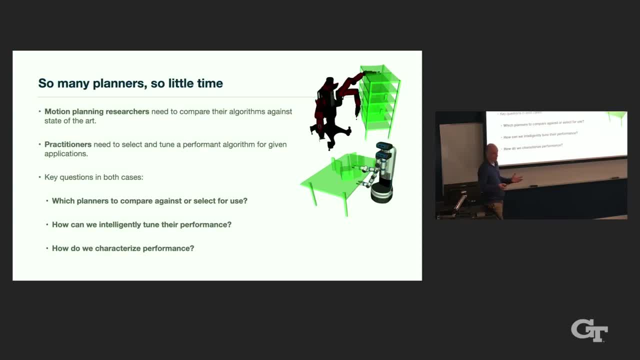 to try And even if you forget about constraints, there's lots of motion-planning algorithms And if you have ideas for a new, better way of doing planning, how do you show it's better? What do you compare against? And in practice people may not care about what's generally. 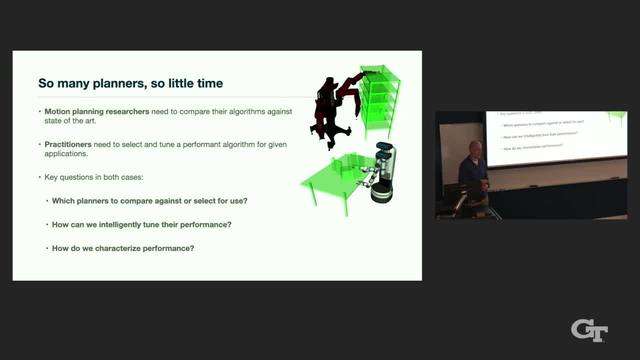 the most sophisticated algorithm. They want whatever works best for their robot doing their tasks. And questions are: what should I compare against? Which one should I use? How do I tune performance? There's lots of magic constants in these algorithms that may be hard to tune. 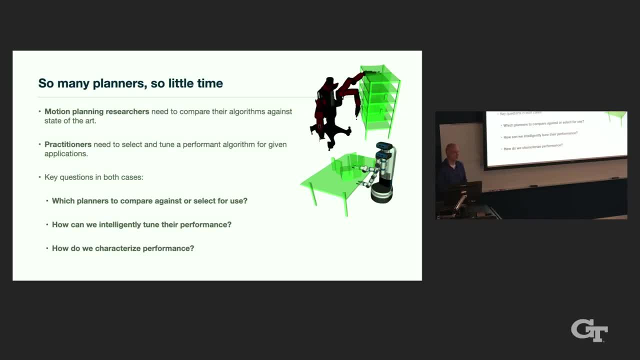 And the typical person wouldn't know how to tune. Even the authors themselves may just accidentally- it's just a trial and error- arrive at something that seems to work OK. It may be far from optimal, And even the notion of optimality is not so clear. 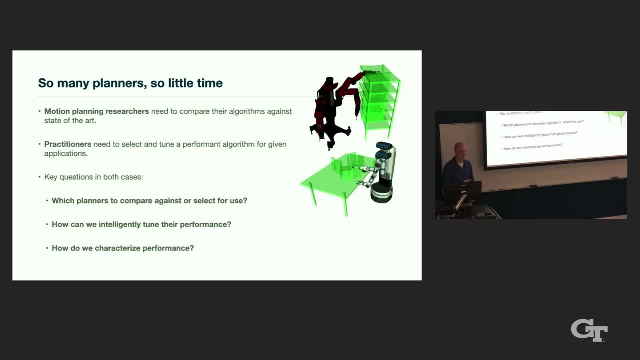 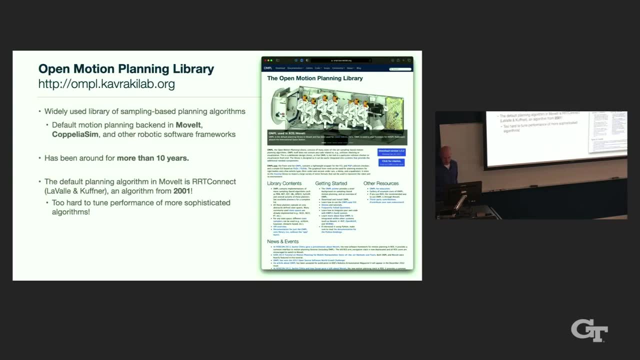 What does optimal even mean? Is this: fast as planning time, Fast as execution, Some combination of both Or something else entirely? Just to give some more data on why this is so bad, I've been leading this development for the Open Motion Planning Library. 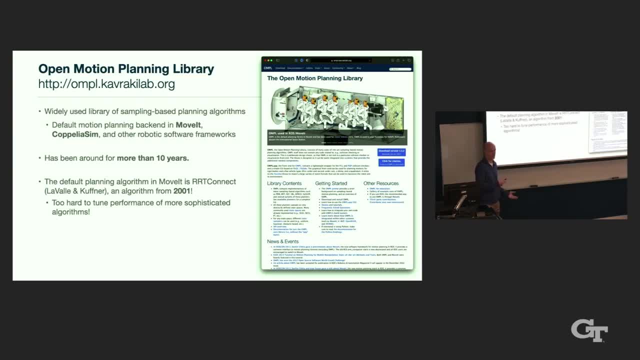 It's a commonly used library. It's used inside of moveit. In this case you use ROS for promotion planning. It's also used inside CobaliaSim. It used to be called VREP. It has lots of different algorithms And it's been around for more than 10 years. 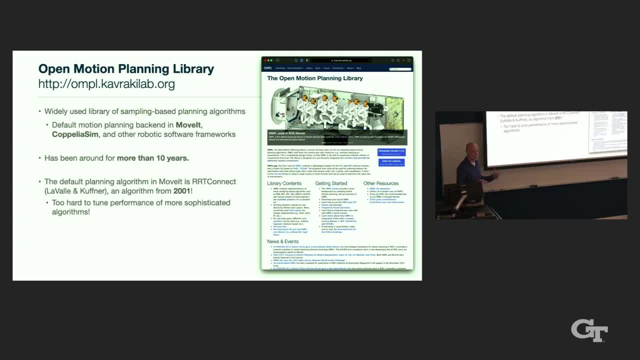 And if you use it today, with moveit, for instance, the default algorithm that it uses is RT-Connect. It's an algorithm from 2001, Steve LaValle and James Kovner. It's really simple. Essentially, it's this bidirectional tree idea. 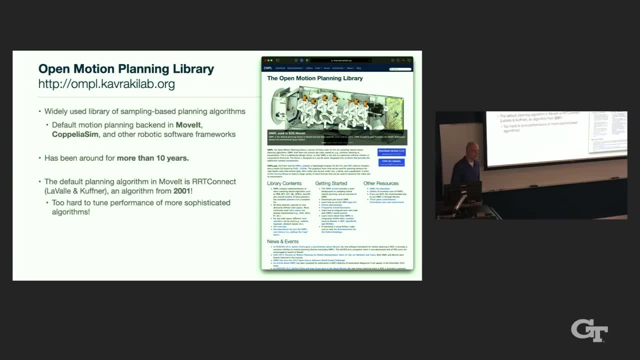 And it has maybe one parameter that typically you don't have to tune. There's a sort of autotune in OMPL that will select some reasonable default for the particular configuration space that you have And it seems to work pretty well. So no tuning works reasonably well. 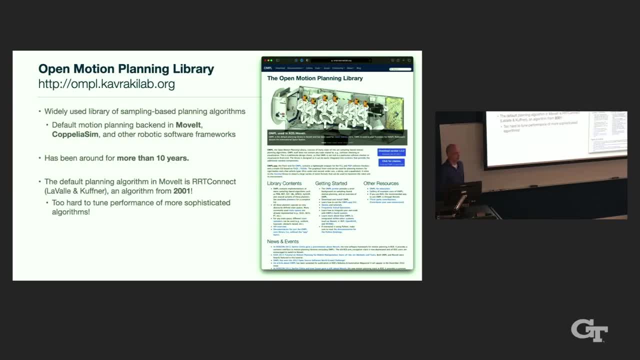 And people say, OK, great, I'll just use that, Because if you use anything else, performance will likely be much worse. So that's kind of like that's not great For us. the motion planning research is like oh. 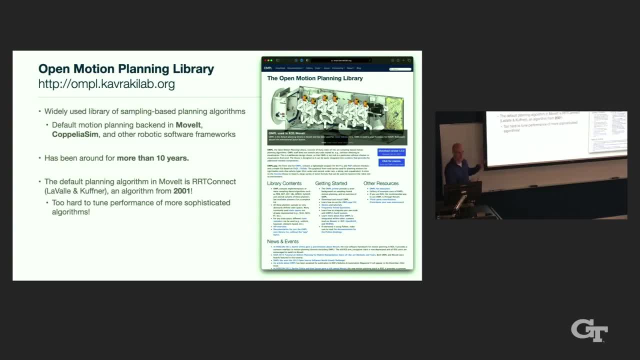 I don't want people to use this algorithm from 2001.. I have nothing against Steve LaValle and James Kovner. It's a great algorithm- But hopefully they've made some progress since then that they can show like: hey, you can really. 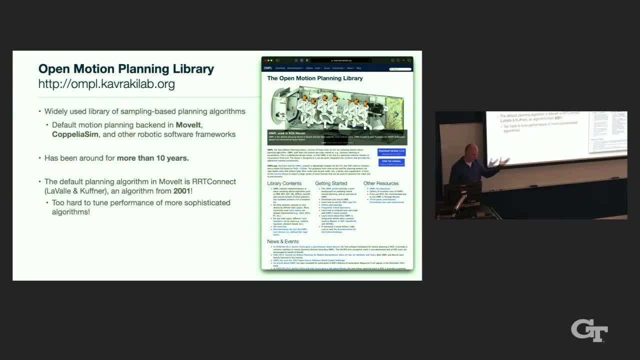 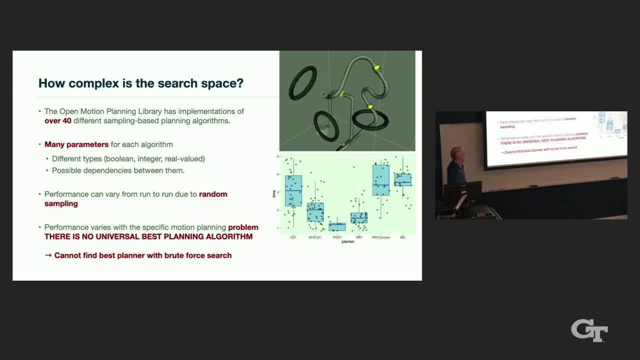 get much better performance if you use, you know, RT-Connect. You know this algorithm from last year or this year. So yeah, there's lots of algorithms And there are many parameters for each algorithm. You know there's Boolean things where 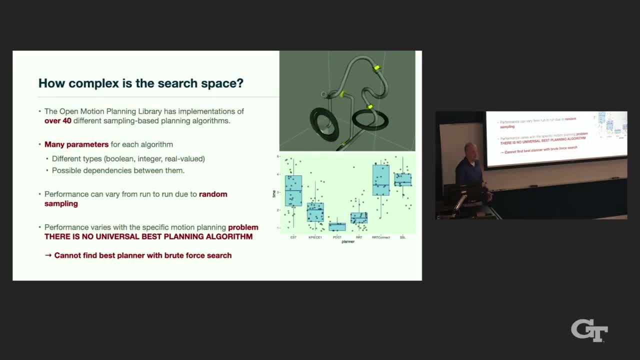 the certain flags are enabled: integer values, real values, certain dependencies between them that may not be particularly well-documented, Of course that's partly on me, But there's some interactions between these parameters that cannot be chosen entirely independently. And since we're doing random sampling, 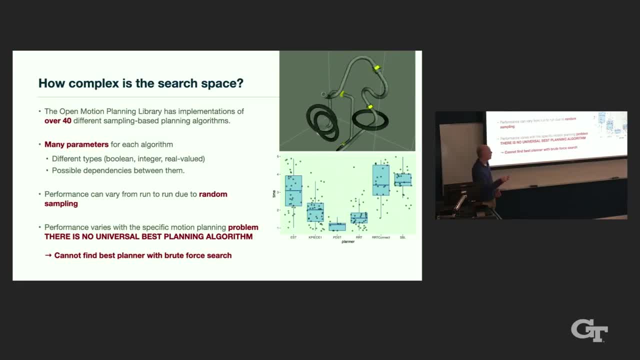 just one run won't tell you the whole stuff, But you really need to look at the whole distribution. So this shows solve time, like how fast you solve this problem for a handful of selected planners, And it shows these box plots, sort of interquartile ranges. 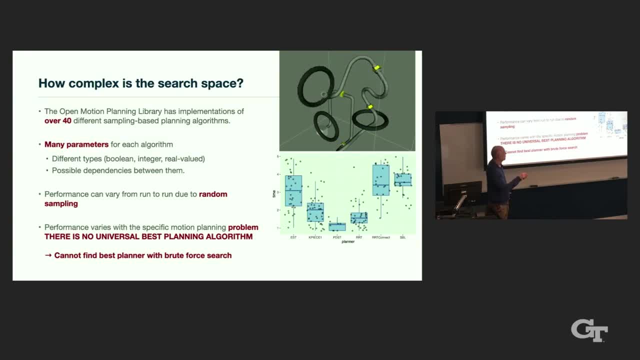 So this gives you 50% confidence to evolve for typical performance for solve time. But you see that the distribution can vary wildly. Which one is better? Well, this one is probably better in this case, But there's still a fair bit of overlap. 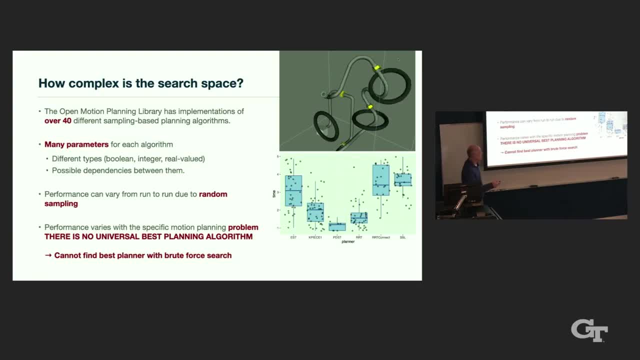 between these distributions, And this is also very much problem- independent, Your problem may look nothing like this. It will likely not look like this, So basing your selection on this problem is probably a bad idea. So there's really no universal best algorithm. 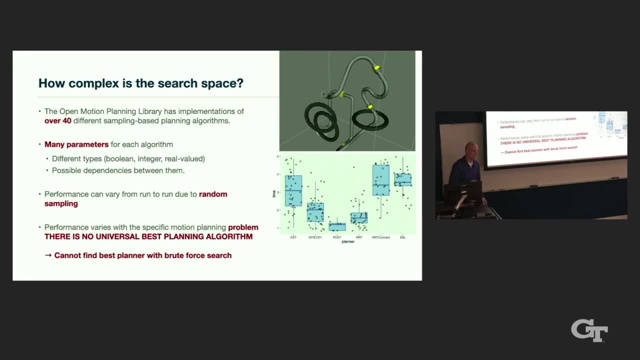 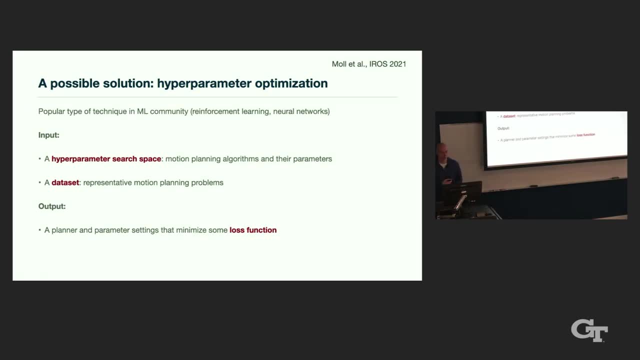 And it's impossible to do this with brute force. So that's the key problem. So one solution around this is hyperparameter optimization. We see this more and more in the deep learning community as well, that this again, all kinds of neural network. 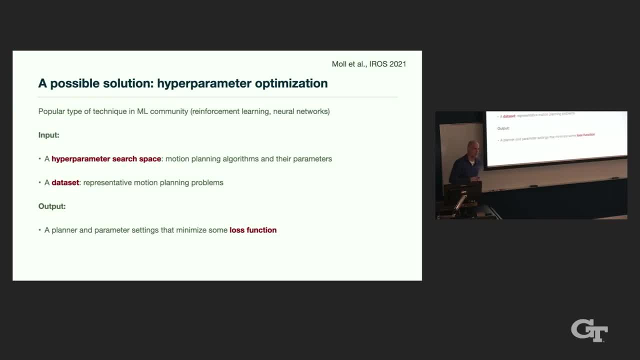 architectures with all kinds of magic constants that affect performance a lot, And typically you see results reported for the configuration that worked. But somewhere in the footnote you see: oh actually we did this search for who knows how many compute years to find a reasonable architecture that worked. 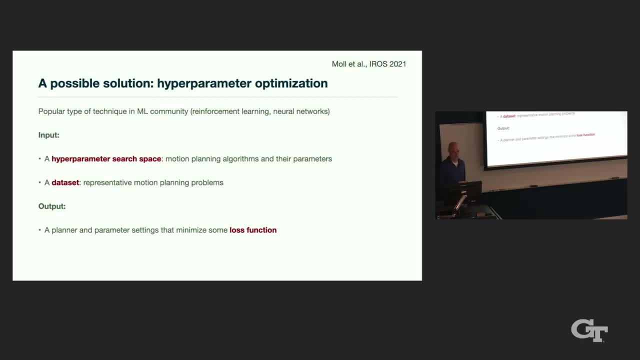 So it's a big problem in machine learning and reinforcement learning. So we have some sort of search space for all our hyperparameters And we have some representive Right, Representative motion-playing problems that we'll use, And then we have to characterize the thing. 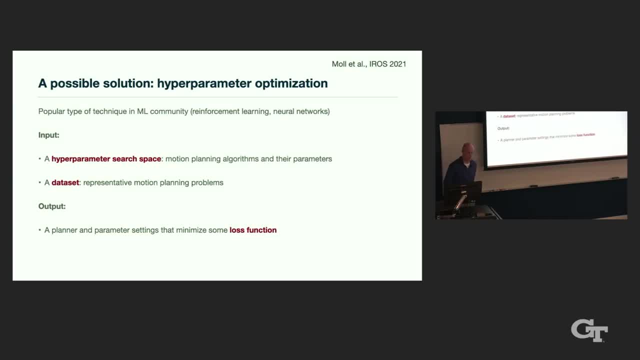 that we care about, with some loss function, so some indicator of performance, And this actually turns out to be the hard part. I mean, the fact is like, hey, using hyperparameter optimization is the solution. It's not exactly the solution, because we still 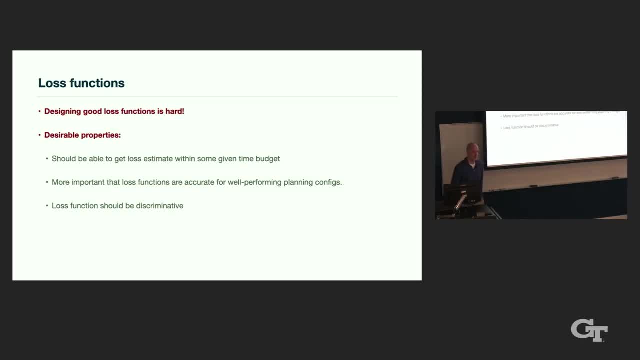 need to have some way to quickly assess performance. that may not involve solving problems completely, So we need to be able to get some lost estimate within some time budget, whether we solve the problem or not, And it's also more important that these lost functions. are more accurate for things that perform well. There will be lots of configurations that if you choose random parameters for them, they'll perform terribly, And it's important that we can discriminate somewhat between terrible and truly terrible. We care more about discriminative power. 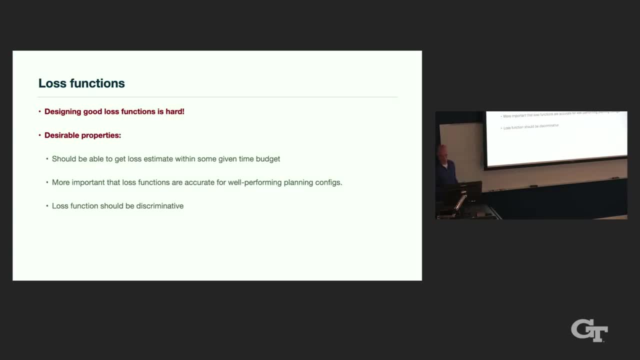 between things that are good and very good, Right. So here's a proposed loss function that seemed to work pretty well. that captures conventional wisdom about what we should optimize for. Most people care more about planning speeds, Just find plans as fast as possible. 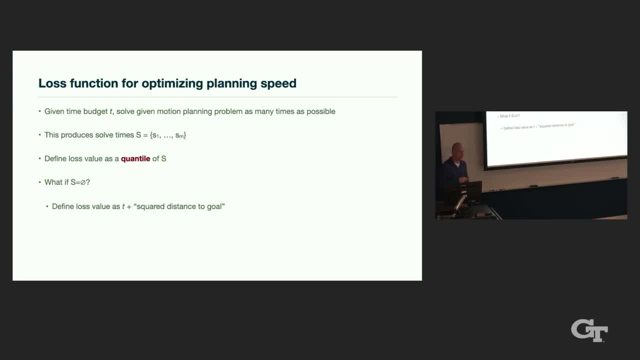 And then afterwards, with a little bit of post-processing time, we can optimize and get things that are locally optimal. So, given some time budget, we can take one of our problem instances and solve it as many times as possible. And we solve it, let's say, m times. 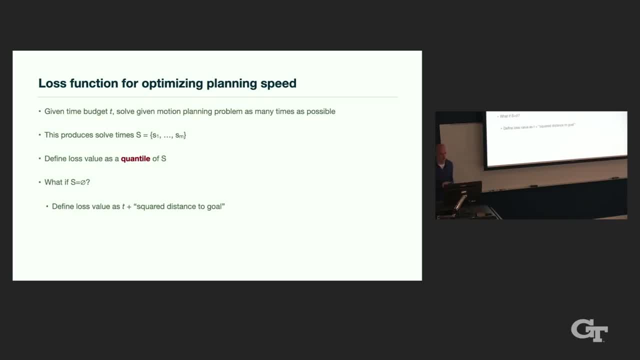 And this is the s1 through. sm is a series of solved times And we can define our loss value as a quantile of s. So we take the 50% quantile and say, OK, this is the median, And the median may not always be the best choice. 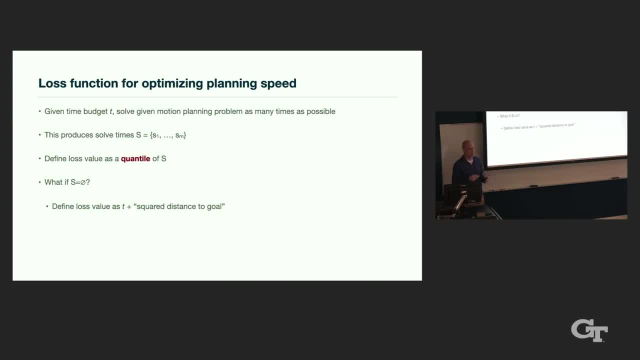 Because in many practical cases we want some bound on the variability, We want a predictable behavior, So maybe we want something that captures some of the variance as well. So that may be an argument of using a higher quantile. If we take 70% or 80% quantile, then we 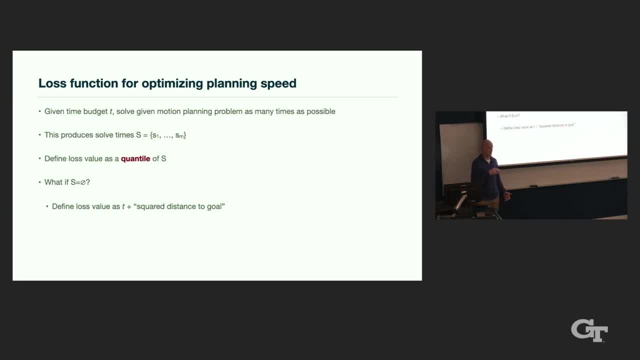 capture some of the tail and say, OK, we want something that, in the worst case, doesn't perform much worse than this. And of course you could say, well, I want the 99% quantile, But estimating that reliably is really, really hard. 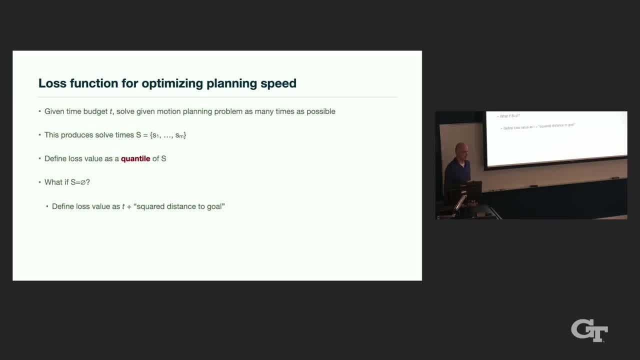 So something in between median and 99 is usually a good trade-off between estimating something that captures variance but it's not too hard to estimate. Can someone think of a reason why you want a lower quantile, Let's say the 30% quantile, 25% quantile. 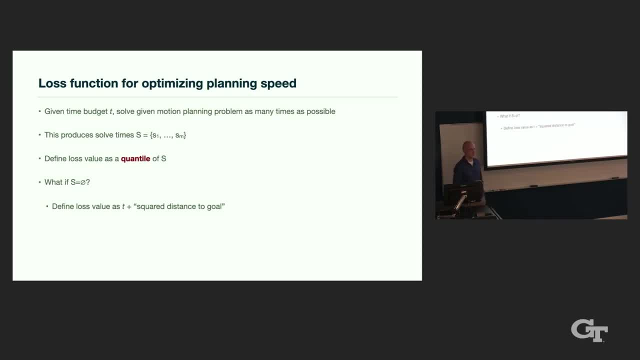 There are reasons to do that too. We could rerun, Sorry, Rerun, Restarts, Restarts. Yeah, actually, it's most useful when you run multiple instances of the same planner in parallel. Essentially, you terminate whenever one of the planners 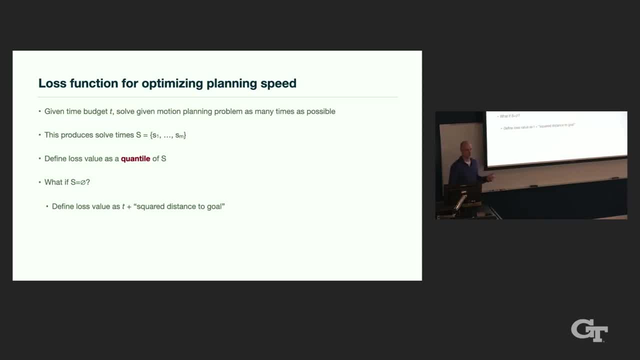 wins. So you have this random behavior, You have this distribution of outcomes. Essentially, you have all these different slot machines that you can pull in parallel, and only one of them has to be a winner. So the variability can be large. So then it makes sense to solve for something. 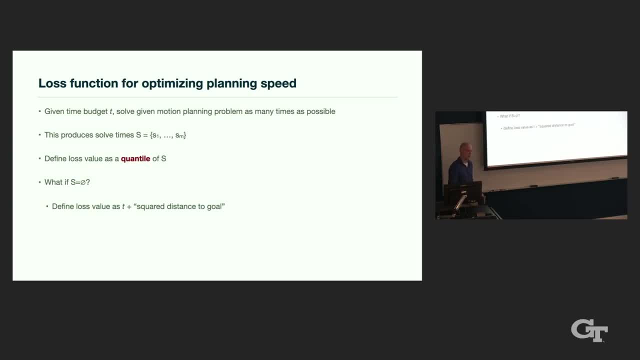 that has maybe a lot of variability, but still a low median. so a lower quantile actually can give you a benefit And you can show, with this kind of parallel running of independent runs of algorithms you can get nonlinear speedups. This is a well-known property of a lot of randomized algorithms. 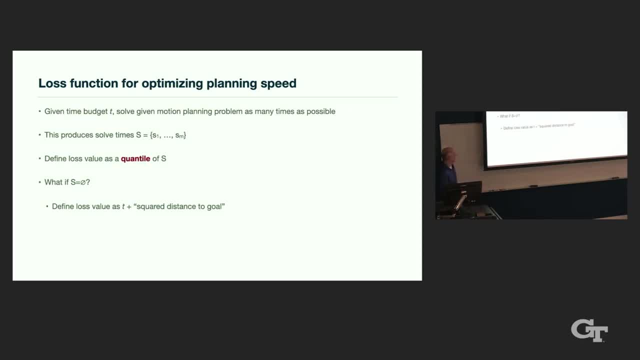 that have this property. So it's possible that within some time, budget t, we find no solutions. In that case, s is the set s of solved times is empty. In that case we can define the loss value as t plus square distance to goal. 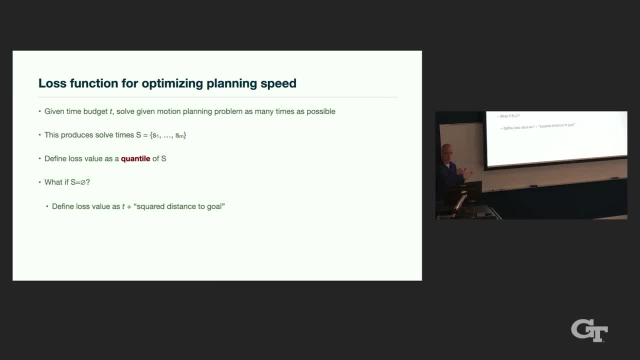 So, even if you solve nothing at all, we get some number, that kind of captures- how close did we get? And this loss value is always guaranteed to be higher than this quantile of s, since we basically start from value t. So discriminate between the ones that solve it. 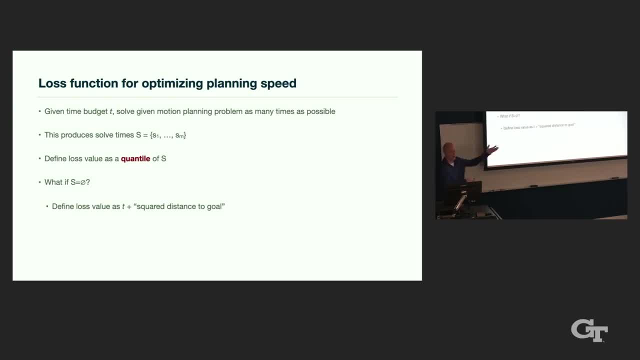 and the ones that don't solve it, And between the ones that don't solve it, we have some way to gauge which ones are better. All right, So we Definitely always use, at most time, t to evaluate this. We are more accurate the more values we have. 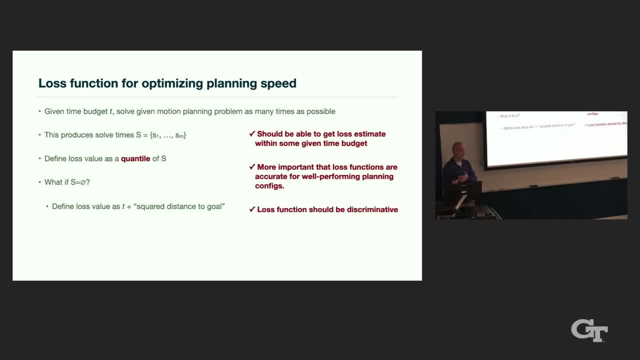 So that checks that box And it's somewhat discriminative between terrible and not so terrible configurations. So this seemed like it checks all the boxes of what makes for a good loss function. Of course, this is just one possible definition. Now, if you have this sort of general hyperparameter, 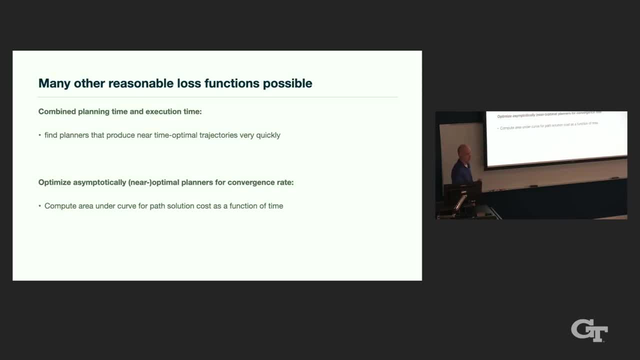 optimization framework. we can throw in anything else that we can now easily formulate. So we can say: well, we want some combination of planning time and execution time, We want short paths that also take short time to compute, Or we want to optimize the convergence rate. 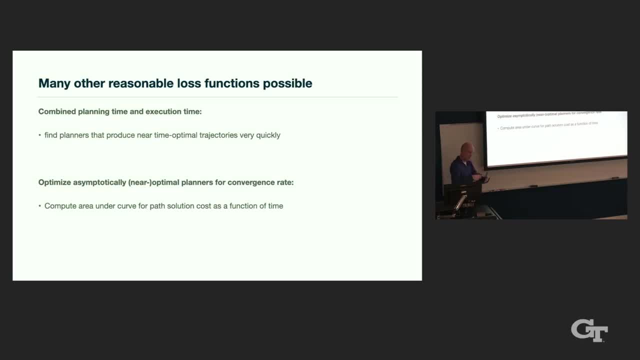 So there's all these planners that essentially never terminate. Maybe there's any time properties that we can return a solution, And I care that this curve of length of the path goes to the optimal path as fast as possible So we can come up with loss functions for that too. 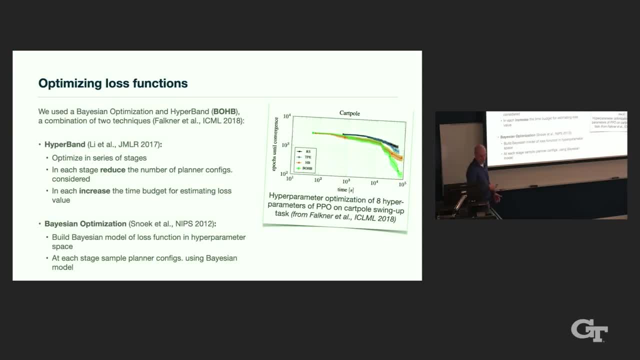 I won't present results for those two things, but I'll show some results for optimizing planning time. So a lot of existing frameworks out there. We use one of them called BOHB, which stands for Bayesian Optimization Combined with Hyperband, And the general idea is that we optimize. 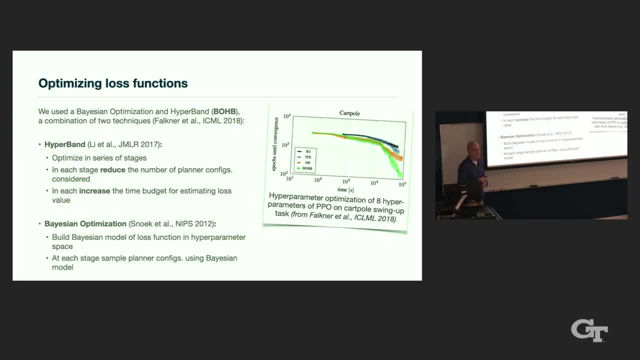 in a series of sampling different configurations. So we sample a bunch of different parameters for planners, planner configurations And each time. so in the initial rounds we have spent very little time. basically, a course, We do a sampling of the entire hyperparameter search space. 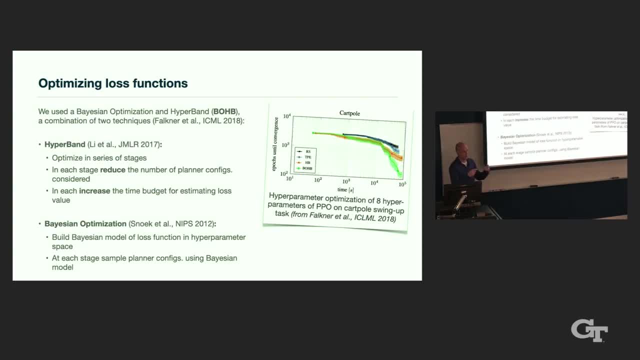 and have a very coarse estimate for our loss values. The most promising ones are kept and then basically we sample some more around that and in subsequent rounds more time And in pure hyperband we basically just keep random sampling. But when combined with Bayesian optimization, 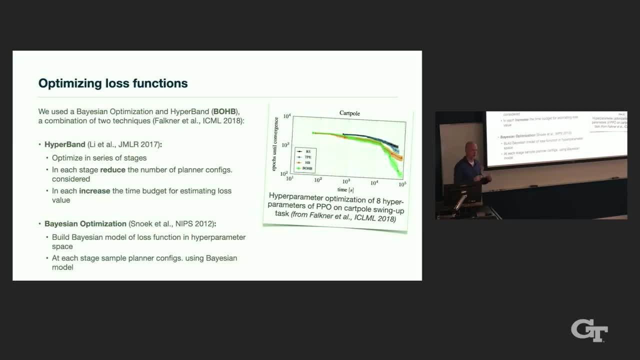 basically, during each round, we refine the Bayesian model of what looks like the most promising part in the search space. So, based on the loss values, we build some belief about: oh, this looks like the right, This looks like part of the parameter space. 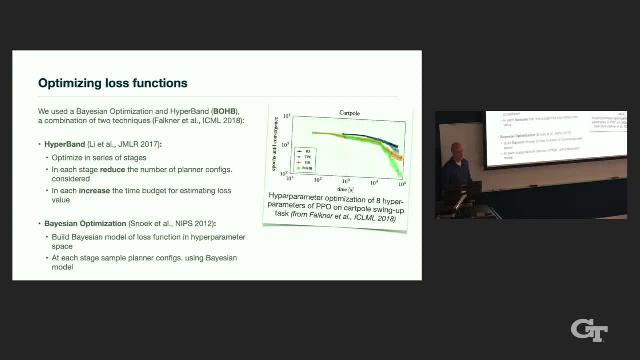 to be searching in And then we sample some more over there with some bias, And we still keep sampling everywhere. with some probability This is showing some results from a reinforcement learning problem, a carpool swing-up typical kind of reinforcement learning task. 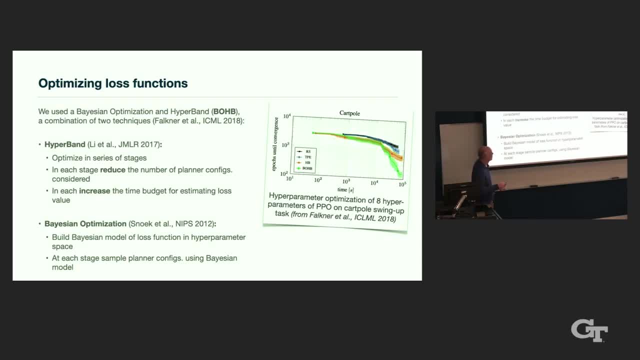 And it showed: oh yeah, this combination of Bayesian optimization and hyperband works really well. So that seemed really promising as a tool that we wanted to use. So we basically fit this problem formulation inside the Bayesian optimization And then we did it. 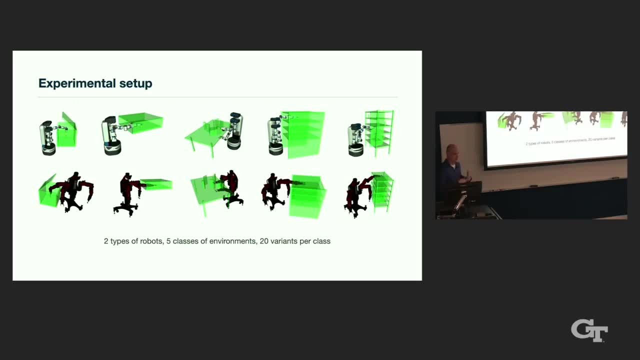 We did it, We did this framework And it worked really well. And how did we know this? So we tried two different robots in five different environments, picking things from inside a box, from a shelf and tabletop, and different kind of shelf arrangements. 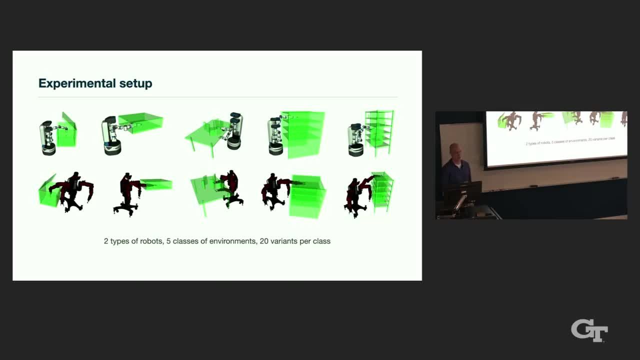 And then we basically did a lot of randomization, lots of variance of each problem. This is just showing one thing, But we moved these different cylinders around inside the shells to create different configuration spaces. So yeah, different spaces to plan around in. 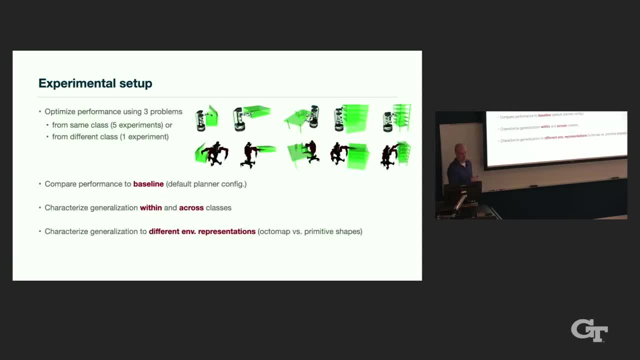 And we did a number of different experiments where we basically take different instances from the same class and see how they generalize across classes or take different problem instances from each class to get basically a more diverse experience to train on and compare that against a baseline. 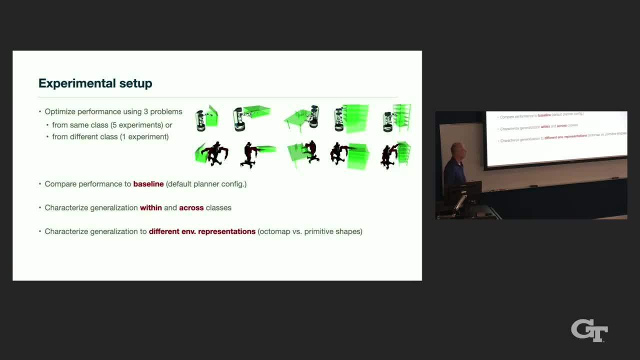 sort of like the default planner, which is, in this case, RT-Connect, since we use Movit and characterize some notion of generalization And also try to generalize across representations, which is maybe not a clearly obvious thing to think of, but this is something that happens a lot in practice. 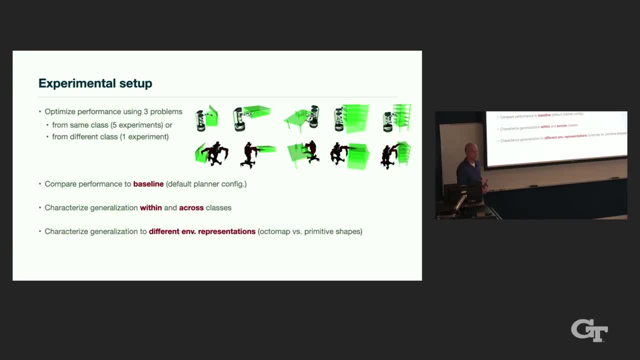 It's nice to have this model of the world and planet. It's nice and clean. In practice we often have just depth images, point clouds and OctoMap as our environment representation, which is the sort of voxel-like representation. It would be nice if a plan that was optimal for this kind. 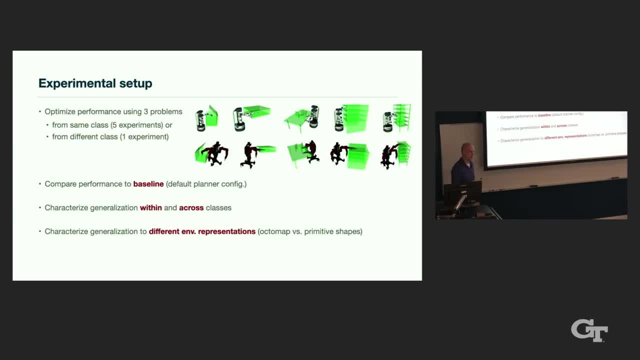 of mesh representation would also be fairly optimal for something that is the OctoMap version of this. It's like it's not guaranteed. Maybe it's terrible. Maybe it doesn't translate at all. Luckily, there's some good news. 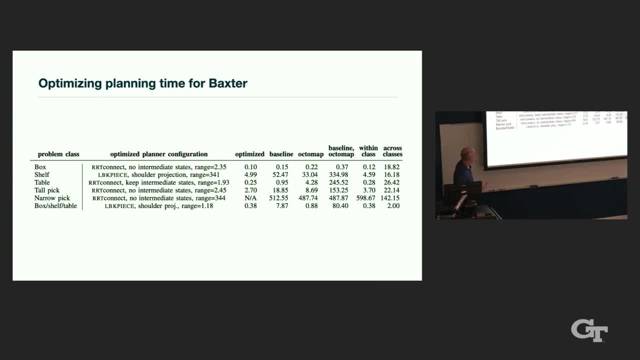 There's a lot of numbers in this table and I won't try to explain all of it, But let's take the simplest example first, this box row. So we started with a baseline of 0.15 seconds to solve this. Actually, this is the loss value. 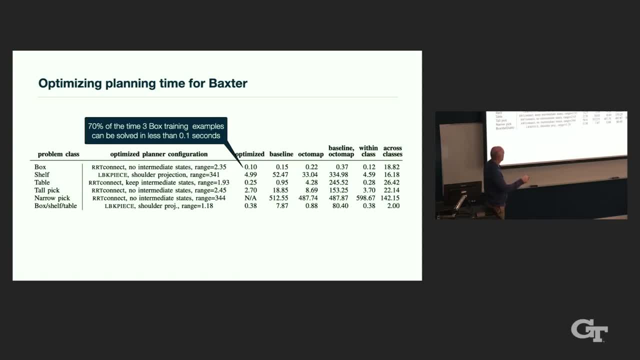 but in this case it is also the solve time And it's optimized. It's 50% faster, a little bit faster with RRT connect still, and does it a little bit faster, And performance is somewhat similar on other problems. 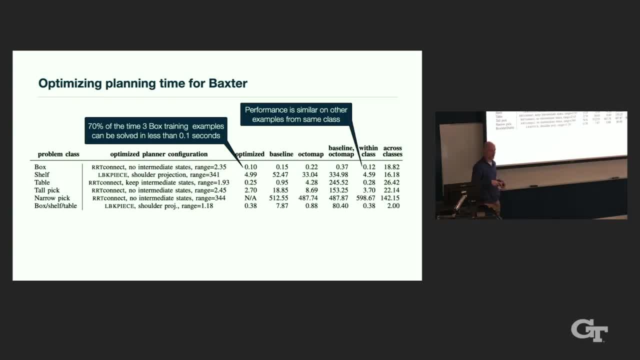 of the same kind. so picking things from a box from slightly different configurations and slightly different arrangement of cans inside that box is about the same. Then, when solving the same configuration using the same configuration for other classes, it's terrible. It doesn't scale very well. 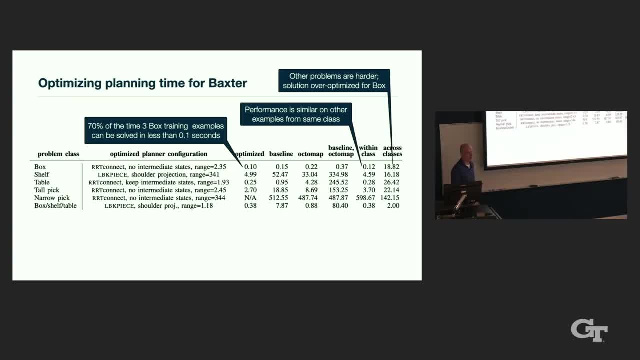 All these other problems are actually harder. It's not that it's It doesn't generalize, It's just these problems are by default already hard. But you can sort of look at the baseline and see like, yeah, all these problems are harder. 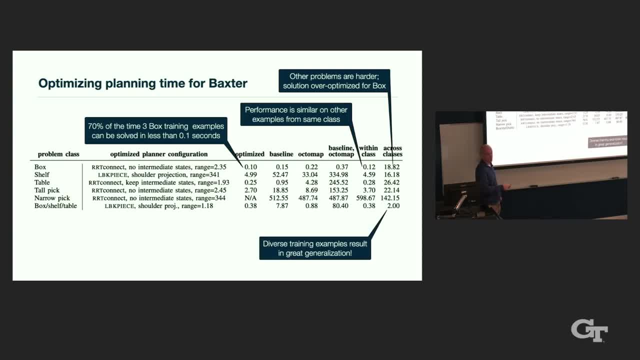 But what's interesting is that we can actually get pretty good performance across the board. Oh sorry, With this last row where we say, OK, take three instances from three different examples: the box, the shelf and the table environment. 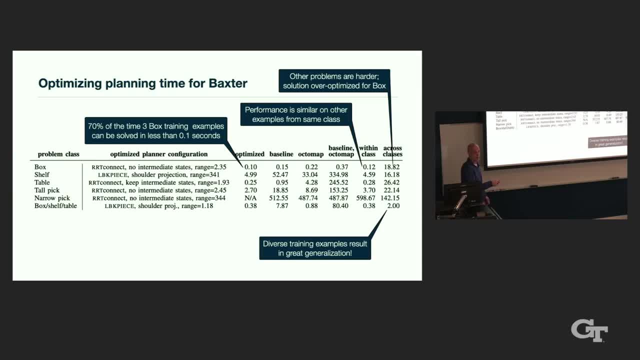 and now we see really much bigger, Bigger in order of magnitude, the difference between baseline and optimized, And on top of that we get good generalization And also- actually I didn't show it here, but- good generalization across representations. 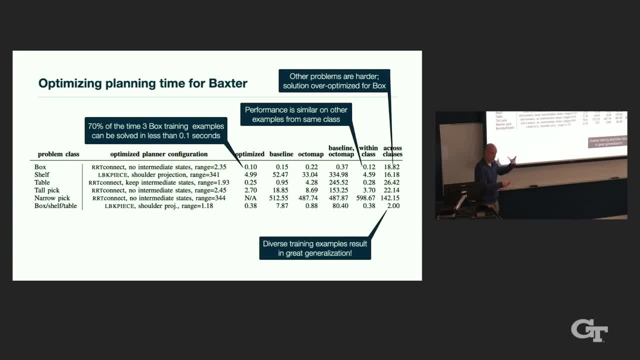 So the Octamap representation is a little bit slower because it's geometrically more complex, but nowhere near as bad as this baseline representation. So as a tool this is just an incredibly practical problem. The contribution really here isn't trying to come up. 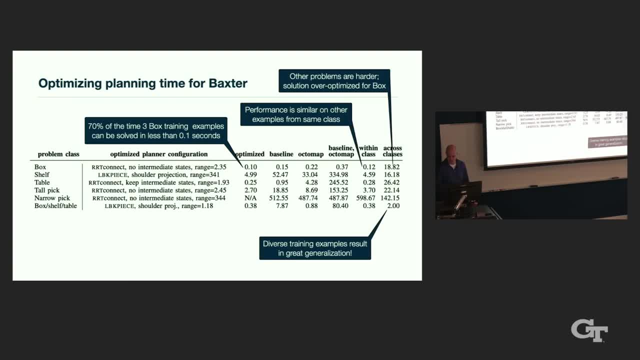 with a good loss formulation that gives you meaningful information. But this is a reasonable way to find a well-performing plan of configuration, With one caveat: if the initial representative problem that you picked is really hard, then optimization may not converge at all. 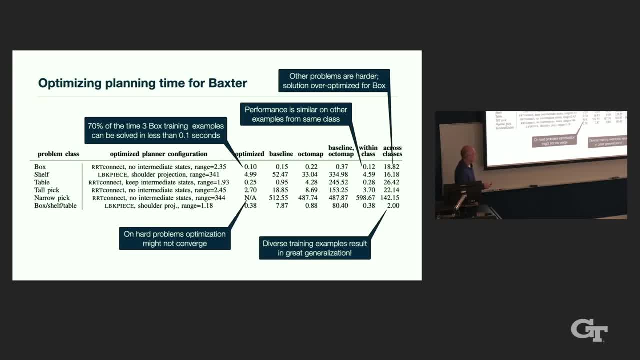 So you see, the baseline was struggling, But in the optimized case, basically, we were timing out And whatever it came up with was terrible. It didn't perform very well at all. So it's a good loss formulation And it seems like this is ripe for some sort of curriculum. 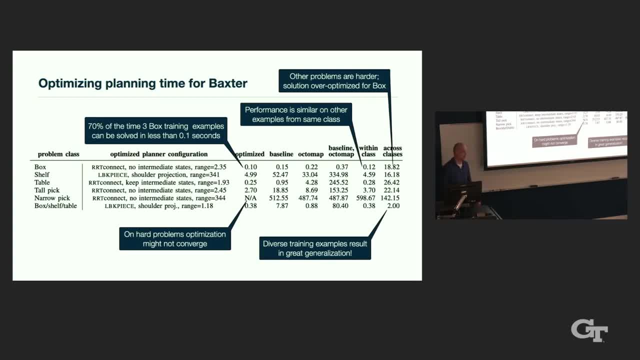 learning, where you basically start with easier problems and optimize that and then maybe hopefully generalize to more complex versions And maybe you have to retrain a little bit more on that more complex problem. But yeah, we are planning to make this open source. 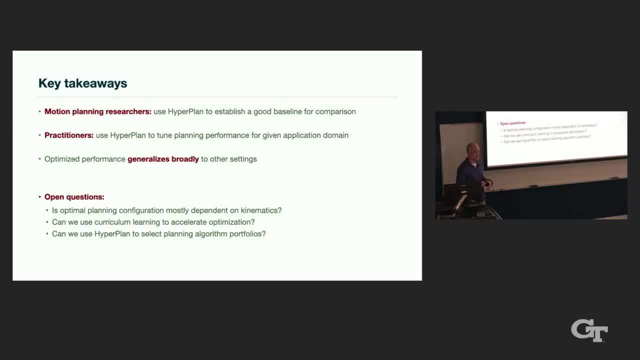 and hopefully make it a useful tool for the community so that anybody who's doing motion planning research doesn't have to make some educated guess about what's going on and which plan to use and actually do a more informed establishment of baseline performance. And luckily this generalizes very broadly. 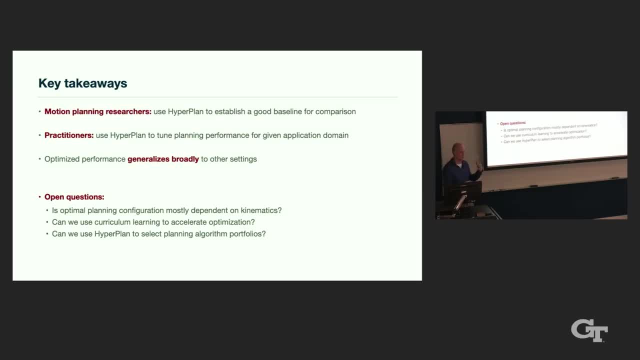 But one of the things that we are still kind of wondering about: how much of it is kinematics dependent? Is it basically just once you've optimized for one robot, is that good for all problems, Or does it still depend a little bit on the problem specifics? 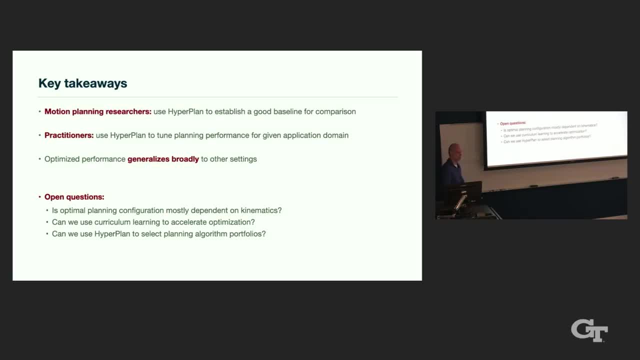 And I already mentioned curriculum learning as a way to bootstrap the learning and start with simple problems, Optimize the configuration And then use that to refine on more complex things. I already mentioned a little bit about this: running multiple instances of an algorithm in parallel. 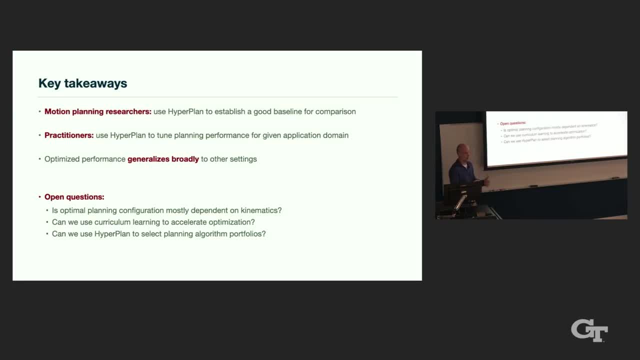 Instead of having instances of the same algorithm, we can use this to use different algorithms, have a sort of competitive portfolio, that sort of hedges against all adversarial scenarios. Like you don't optimize for one problem, You have sort of a bag of tricks. 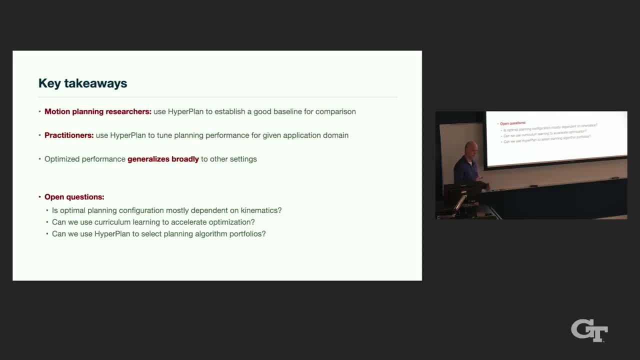 and you run all these algorithms in parallel, And surely one of them will be successful against the particular environment if you engineer it, And so this may be a way that you can find a way to competitive portfolios. All right, So that's all I wanted to say about planning. 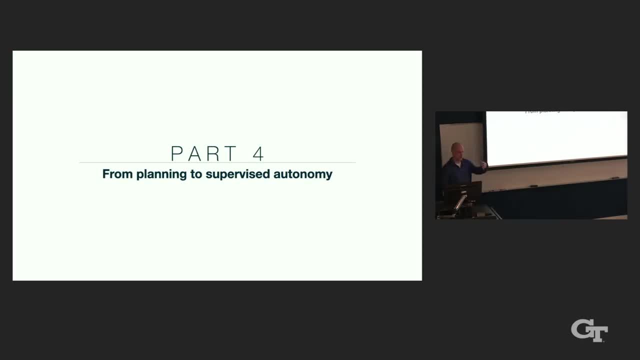 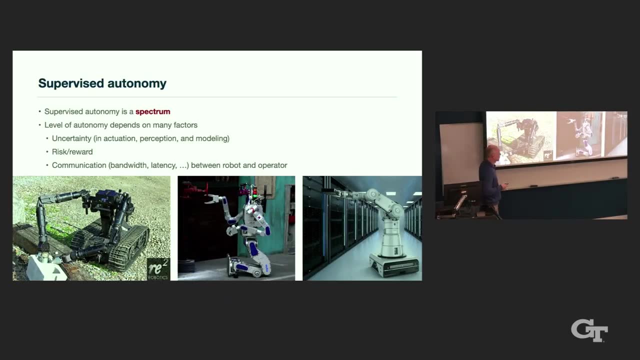 Now I wanted to sort of go back to that earlier example where I showed this robot doing things inside the space station and figure out how we can use this now to move towards more autonomy. So the, I think, everybody who's interested, I think. 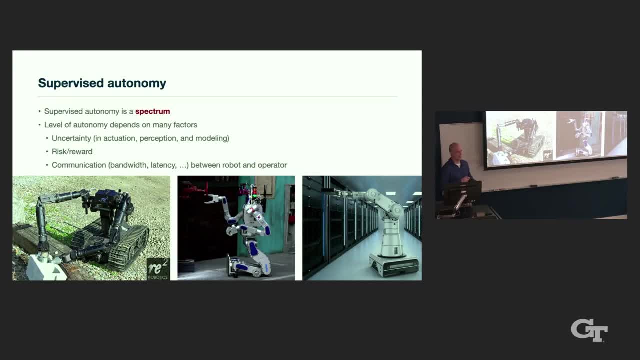 everybody who's spent significant time with real robots will realize that there's a lot of things that it's to make 100% autonomous and have it work all the time in the field- not in a lab setting, but making something really reliable that you can just hand. 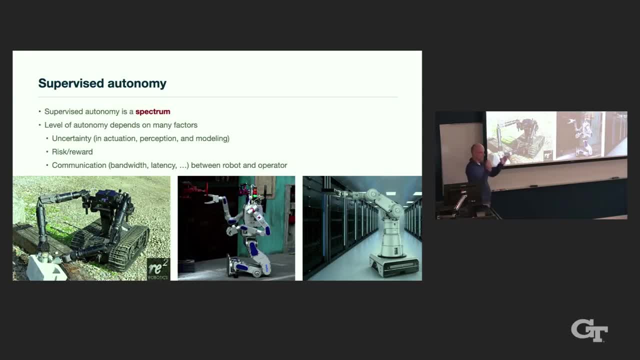 it off to a non-roboticist, Like here. this robot performs this task 100% reliable. Like autonomous cars, there's often still a call center, for the rare exception that a human driver or a remote driver can intervene and take over. 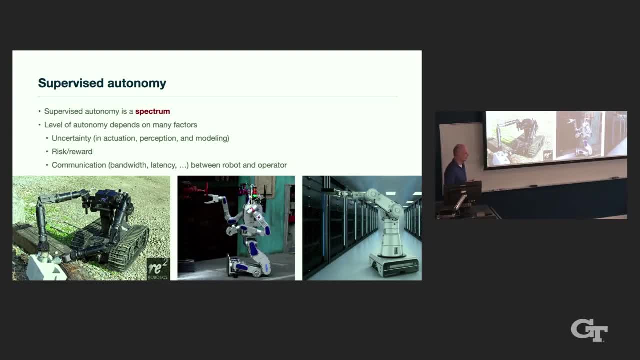 But vacuum cleaners, mostly no human in the loop, But for anything more complex we'll still need a human. So here is: how much human involvement you need depends a lot on this level of autonomy. It's really a spectrum, And how much autonomy you want depends on lots of things. 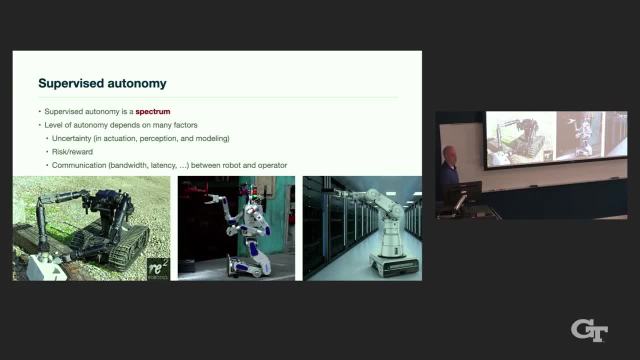 like uncertainty in actuation, perception, modeling, risk-reward. So here this is an explosive ordnance disposal robot, High risk-reward if the clock is ticking. maybe you want to take more risk if the clock is not ticking. 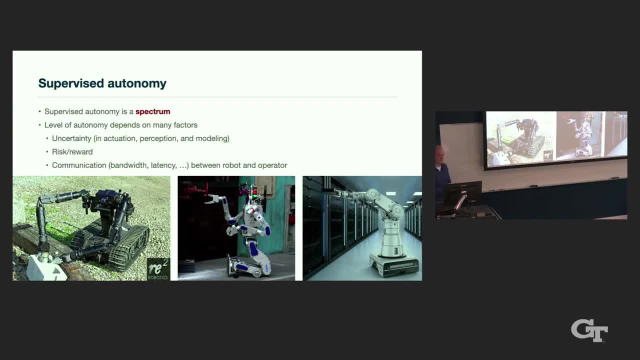 You definitely want to take your time and maybe have a little bit more human involvement and not just press autopilot. Here's a picture of a DRC challenge. This is supposed to model the Fukushima nuclear disaster, where you really can't put people in there. 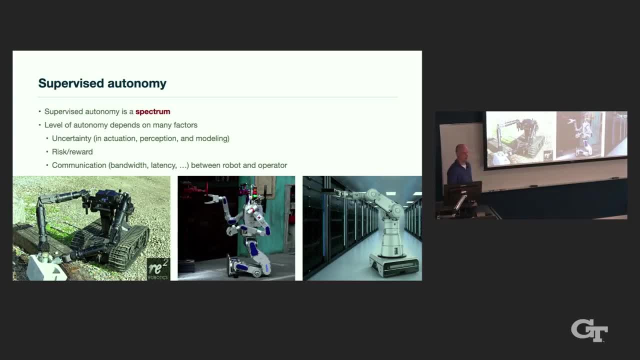 need robots in there, but there's basically bad communication, So maybe joysticking robots is just not an option. You need some autonomy. You need to get some useful work done. What's the best way to script tasks? And we're relying on planning and good control. 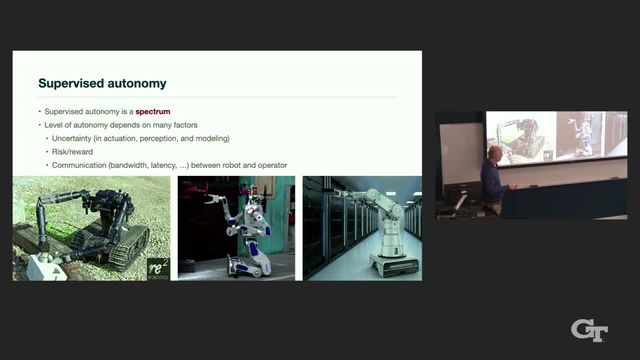 policies and good perception. And then the right is an example that's sort of most clean, where you have a data center where a lot of companies don't want people in data centers anymore because that's contaminating things And it would be much nicer to have. 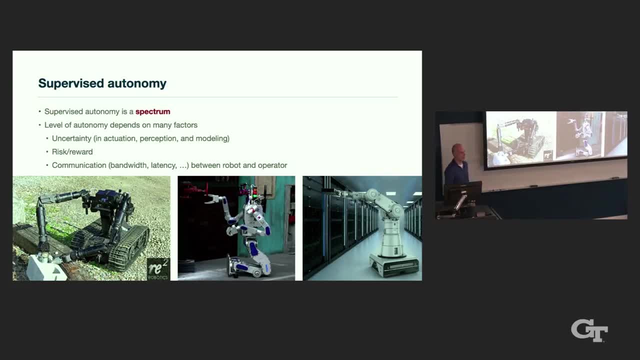 robots just swap out computers, hard drives and cables. They're all known objects. Things can still go wrong every once in a while, but it seems more amenable to almost fully autonomous, where we can have some minimal level of human supervision. but it's possible. 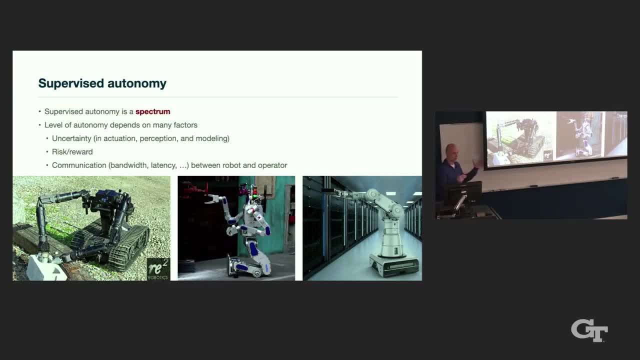 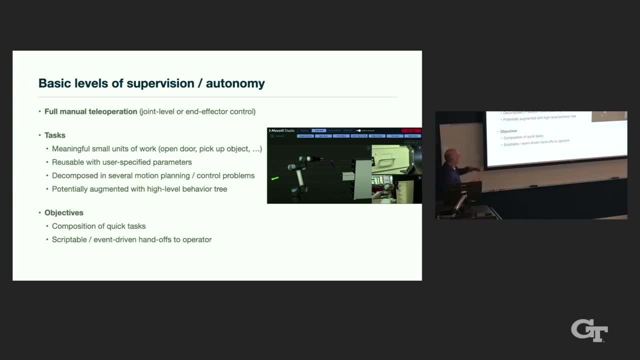 that we can have one person control 100 robots in a day and lots of data centers around the world. So on the spectrum of full autonomy, we have full manual teleoperation, which is not entirely satisfactory. It works for some cases And actually an explosive ordnance. 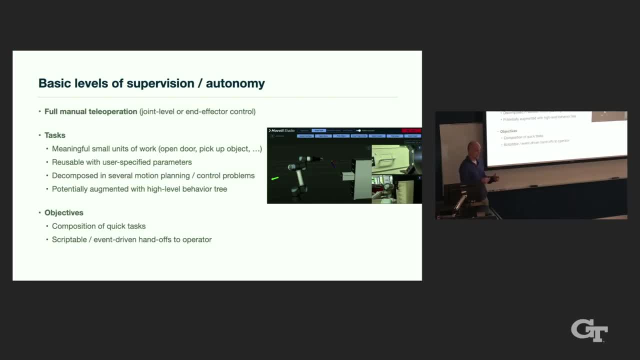 is a lot of people who are trained for that get really excited that they have these game controllers. They plan in joint space, which is the worst. They're controlling individual joints and they get a kick out of being really good at it. 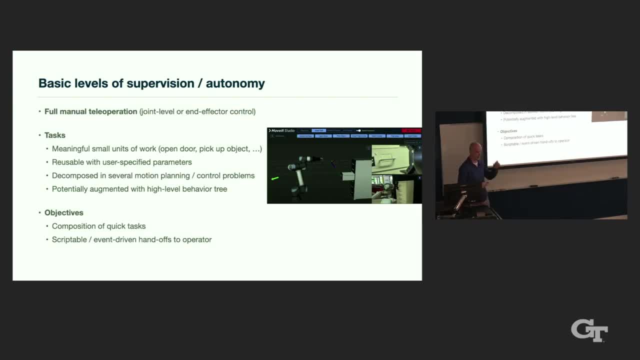 And if you tell them, hey, there's an easier way, just press this button and it will just move towards the bomb, And no, they don't want that, They don't trust it. So there's also a human element in there. 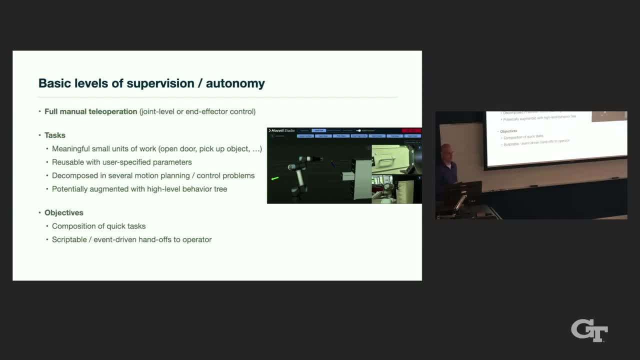 How do we get people to trust robots And how do you get them to see that there is a better way? And that's a whole other question. That's a whole other side to the story, Just demonstrating that it's possible to do this reliably. 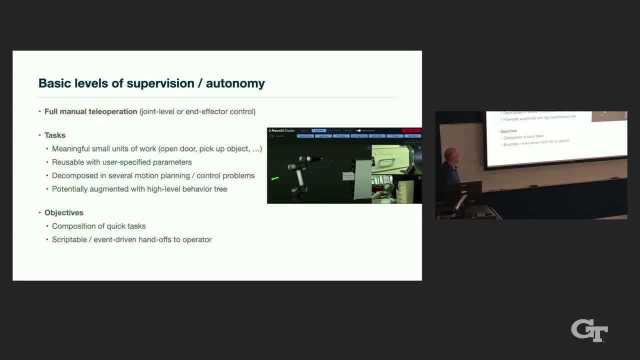 with minimal user inputs is a hard challenge, But we can definitely identify small units of work that seem like they're. you can kind of think of them as canned behavior, even though they're not quite canned. If I approach a door with a mobile robot with an arm, 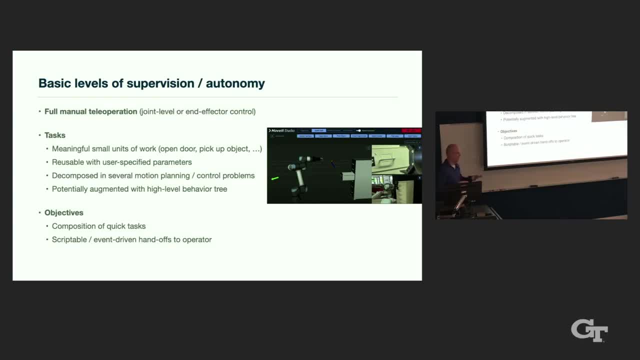 each time it's going to be standing somewhat differently And the handles may be slightly differently oriented And the doors are mostly standard but not quite standard, So the motion has to be adapted each time. So there's definitely room for planning, But once I've identified important parameters, 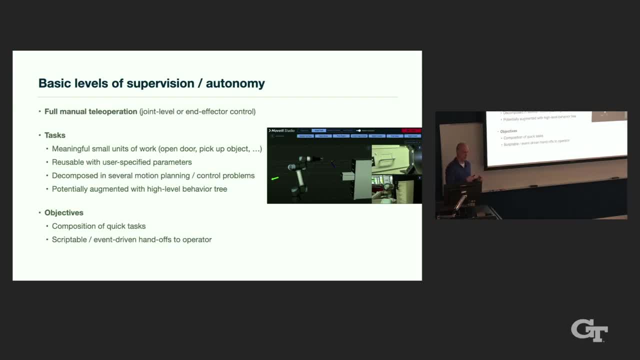 where the hinge is where the handle is where I stand relative to these things. I can fill in the rest right with motion planning, So we only need the human to kind of verify that. I identified the critical parameters right, Like where's the door handle? 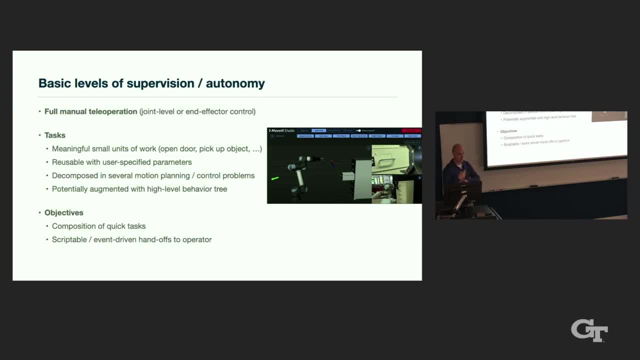 Where's the hinge? Where do I stand in the world? Then everything else can be left to planning and control. So that's the part that we're working on, where we this is. I'll show you a video in a moment where we're basically showing how you can open doors. 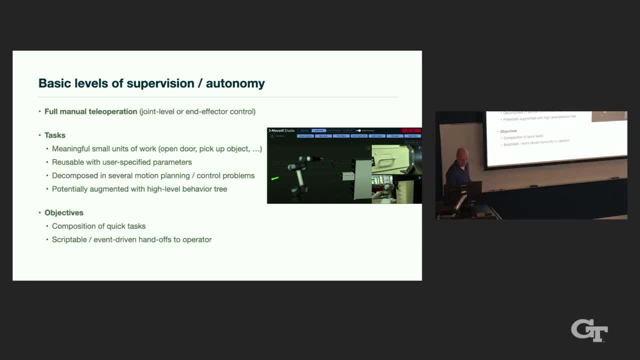 or open doors with a robot with sort of minimal inputs- And these are sort of reusable building blocks, right, Some parameters that are usually provided or verified, And we can have some several motion planning problems along the way. even for something as simple as open a door, maybe you have a free space motion. 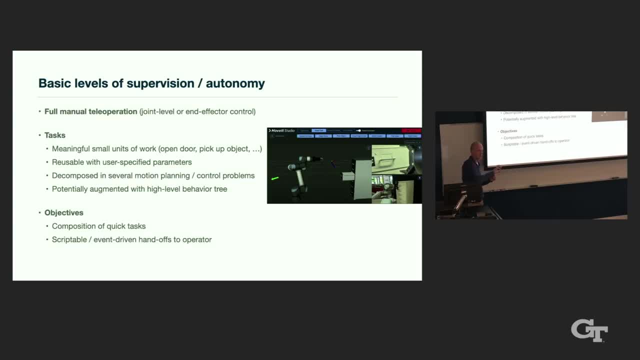 to kind of approach and kind of Cartesian motion where we sort of approach the handle and close the gripper and pull out in a certain way. That already is like even something that simple is really decomposed in sort of several motion planning problems. 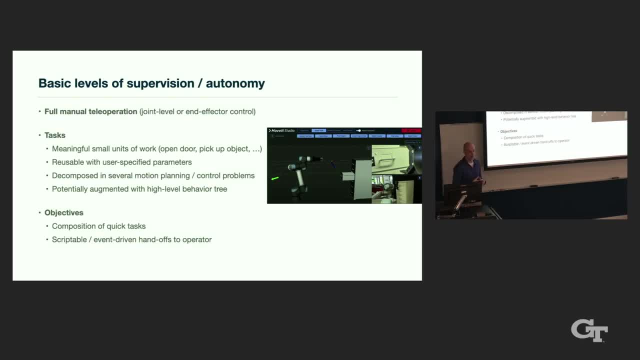 And then we have some possible backup behaviors. like things can go wrong: Maybe the door jams and I have a backup behavior, or I may try to pick up an object a few times before I decide. okay, I need a better way to do grasp post detection. 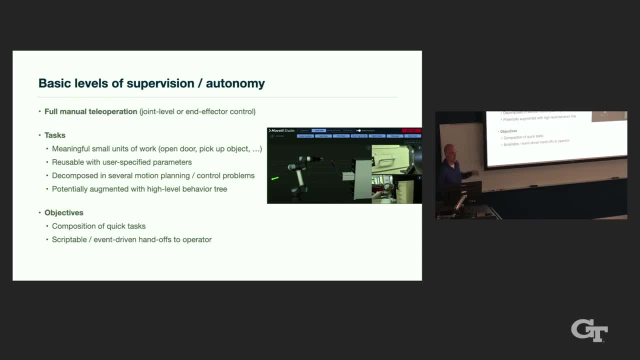 So there's already there. in this basic task, there's just enough complexity that it's not just one motion planning problem. there's policies involved and controllers involved. Next step that we want to get to, then, is objectives. Now we have these basic building blocks. 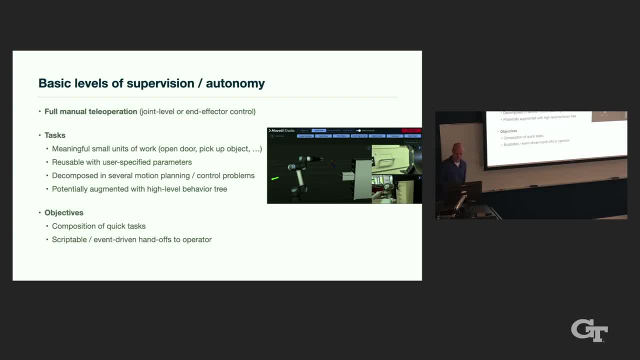 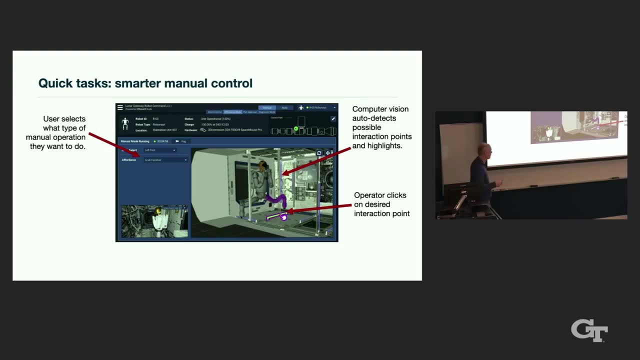 we piece them together into bigger tasks. So this is a wireframe design, so this is not real just yet. but the idea is like, let's say we want to walk inside the space station. we basically just select at a basic level, just like: oh, which foot? 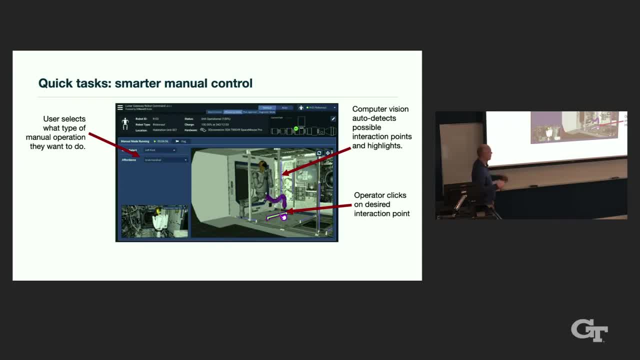 we want to move next And once we decide that we are walking within that context, all we care about is where handrails are. if we just select the handrail, not the particular position on the handrail, we don't care, just say, move to this handrail. 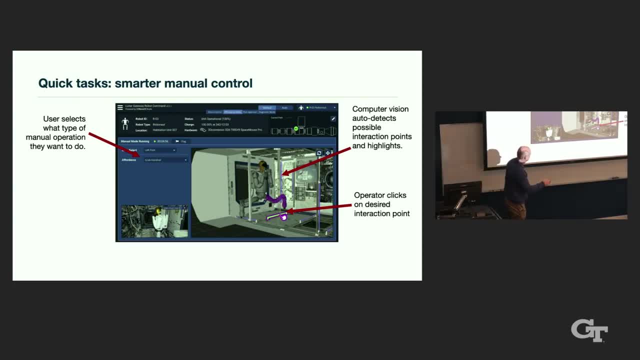 and it will solve the rest, Because it may be that this particular exact position is unreachable or undesirable for whatever reason. So we leave the planner enough freedom to sort of figure out the rest. We just say: only the symbolic high level bit needs to move to this handrail, but where exactly? 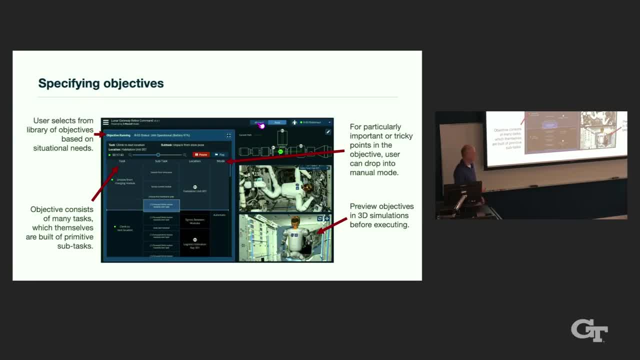 we'll leave that up to the planner And once we have done that, we can basically piece these blocks together. this is sort of a timeline where we have different tasks with different subtasks and we can specify along the way like: oh, at this point. 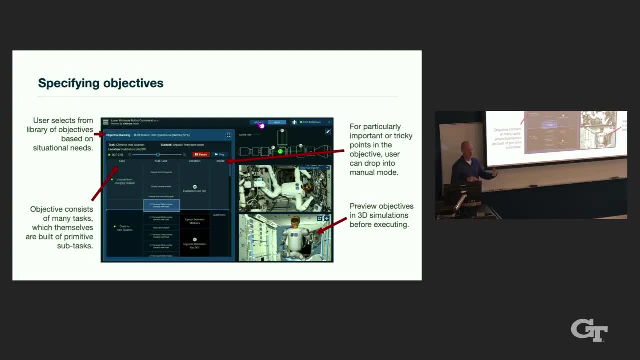 let's insert a breakpoint. I want to manually inspect. Or we have some event-driven thing that they'll basically call a human operator say: oh, at this point we need to definitely check everything is still on track And as we move through this timeline we can show. 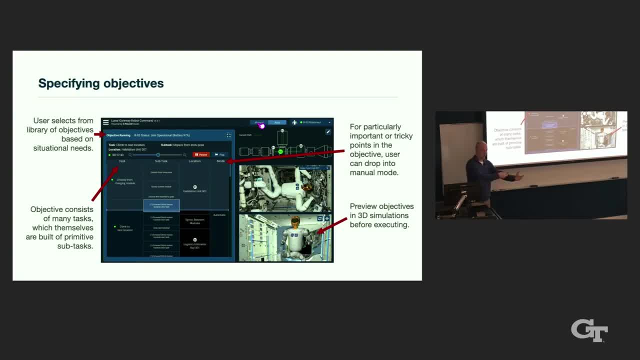 a visualization of a canonical rollout of the policy that we've computed, but of course, during actual execution we'll see the actual video of actual execution. A lot of this is still sort of in the pipeline. This is kind of where we're headed. 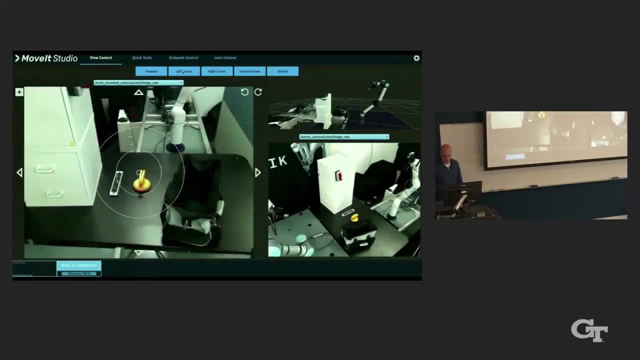 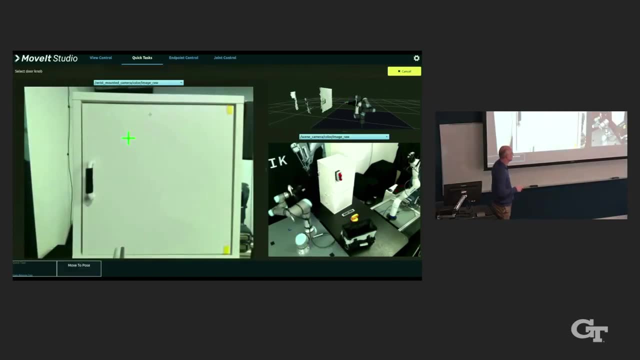 To give you a little bit of a flavor of where we are now. this is sort of a little setup that we have in our office. We have a UR5, we have a little cabinet that we can do door opening and drawer opening. So here we mark the handle and the hinge. 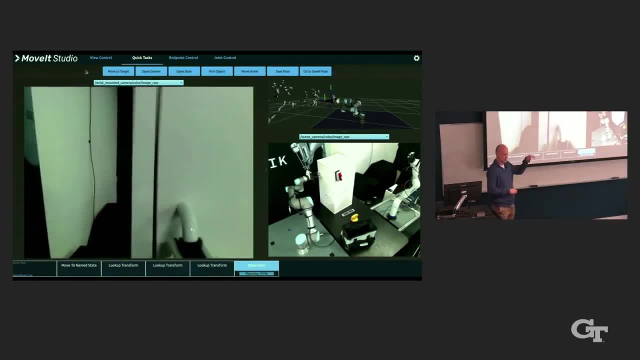 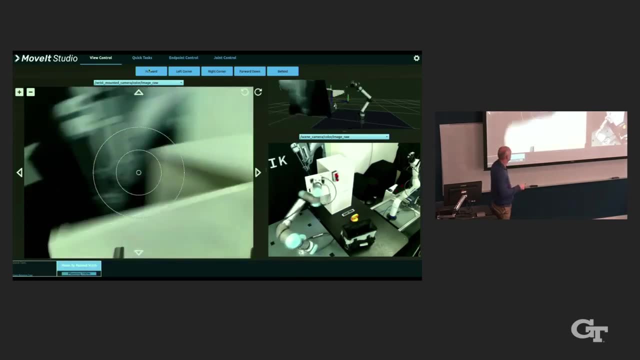 Of course in the future we hope that perception will just kind of suggest like: oh, it looks like the hinge is over here, and then we can have this constraint that it will not rip the door off the hinges and open a door. 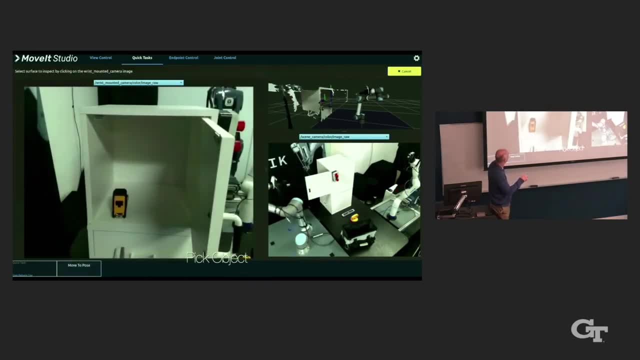 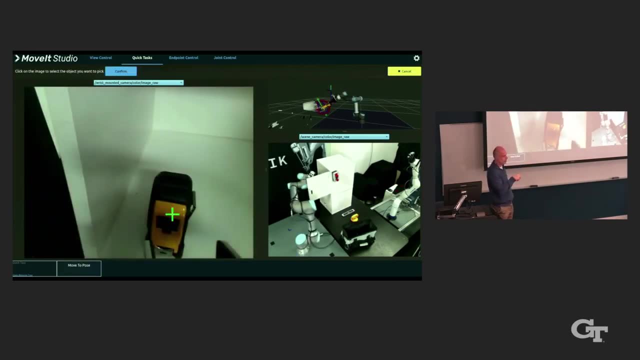 And then there's different ways to do inspections. We kind of have. we can basically specify a certain distance that we say, oh, I want to get this close to the object. We can do a lot of these things in the image plane. 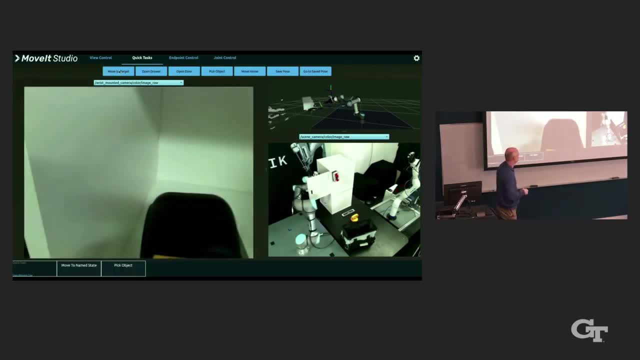 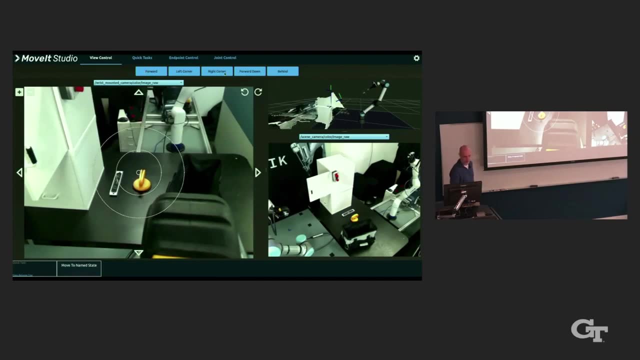 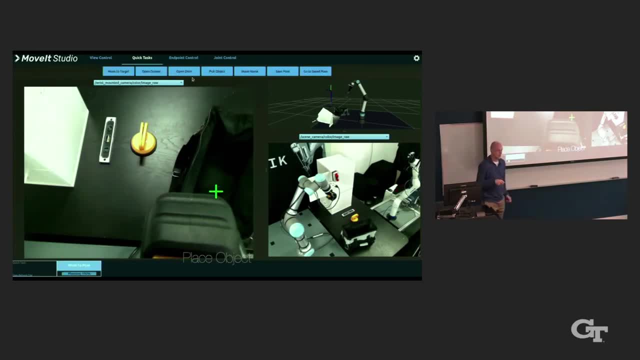 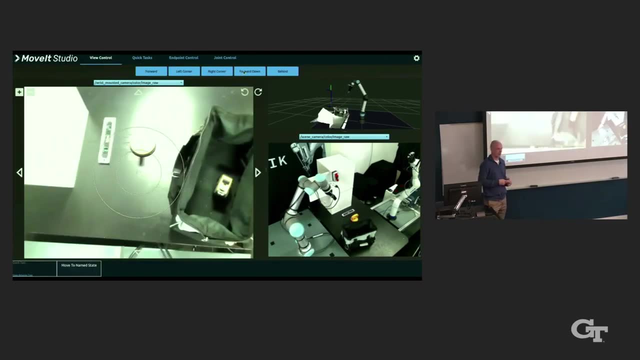 for situational awareness that flash there for a second, We can say, rather than having to drive the camera around to figure out what the world looks like, we just say look from the left, look from the right, look behind. So you kind of take away that part of reasoning. 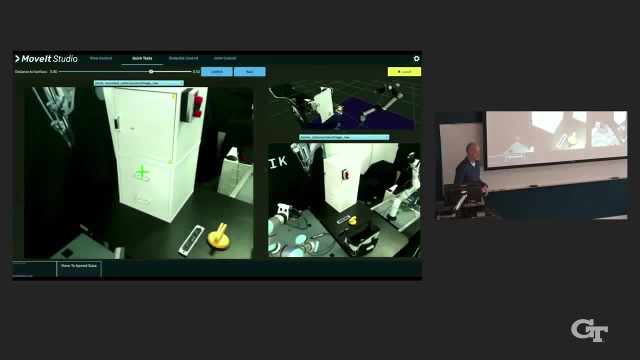 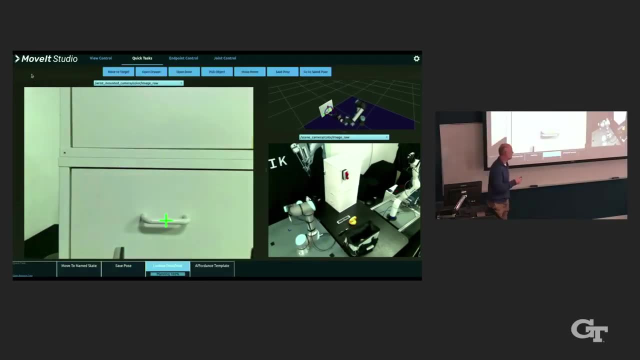 about the kinematics and trying to avoid singularities and joint limits, So that's much easier to lead up to planning. It's definitely possible to give you manual control, And we can, and we do that in some cases, But for things like situational awareness. 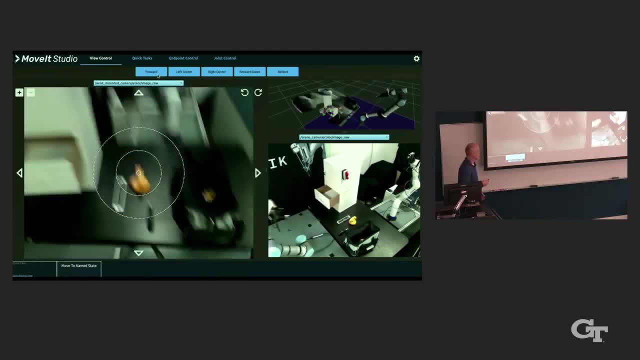 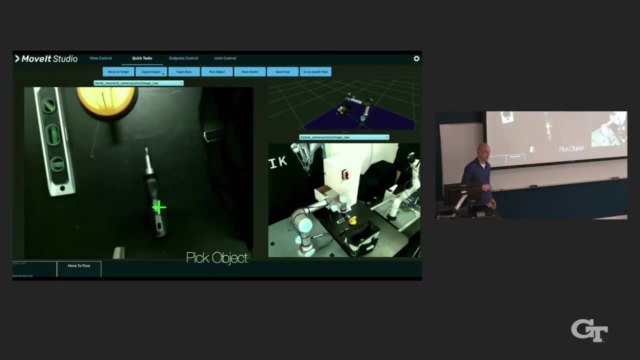 it's just so much easier to just say: look from a few canonical viewpoints and give you that kind of perspective, And at the bottom it shows you kind of a linearization of the policy. right, It's like: oh, it goes to these different states. 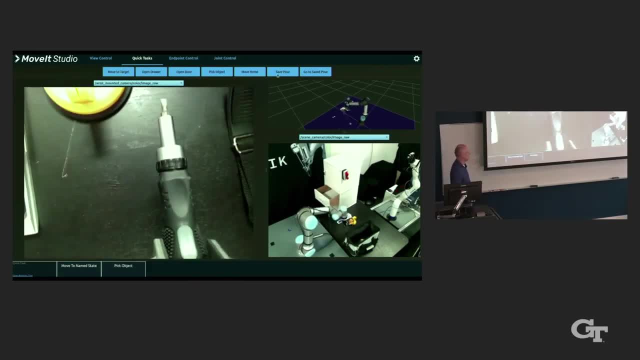 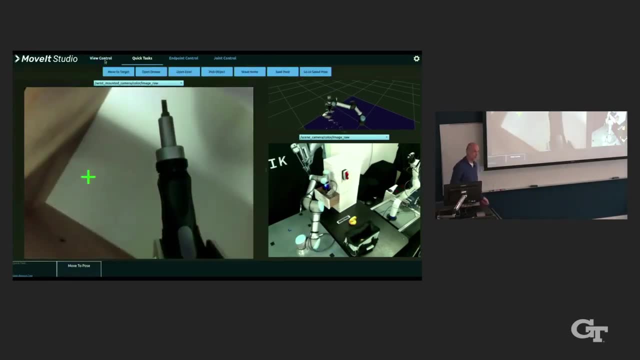 but under the hood there's more complex policy. that actually is more like a graph. But yeah, ideally in the future, like when I have the basic building blocks, you can say: fetch me a screwdriver from the filing cabinet and it will just be able to go through. 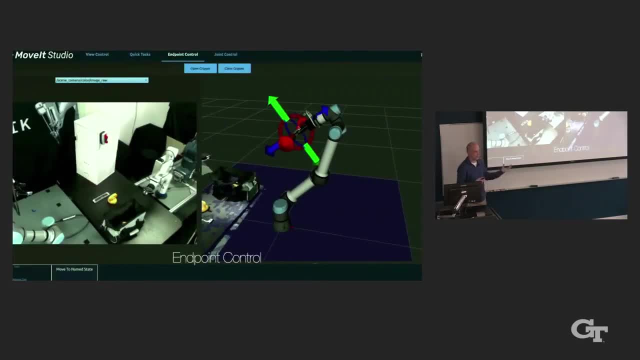 sequentially through the drawers in some order until it finds the screwdriver and get it back to you right? So that's, this is just showing like basic building blocks. Next is just building on top of that. This is showing you just like low-level capabilities. 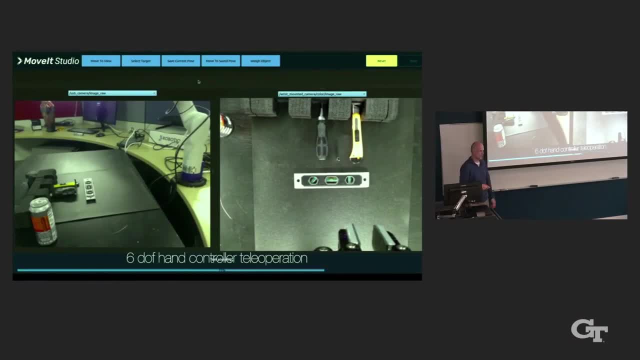 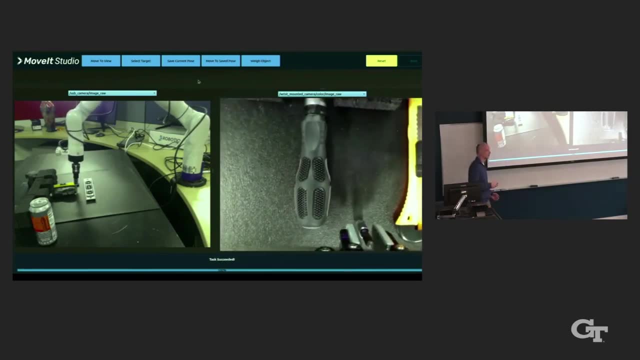 Like, yes, we can still joint control because in the real world many customers still want it, Like the EOD guys, the explosive ordnance guys still want to be able to, when needed, to, go to joint control or have really fine end-effector control. 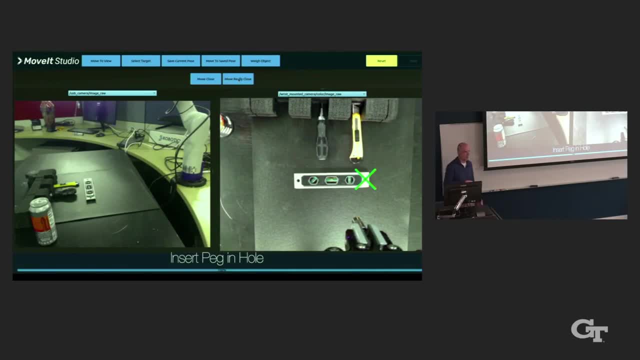 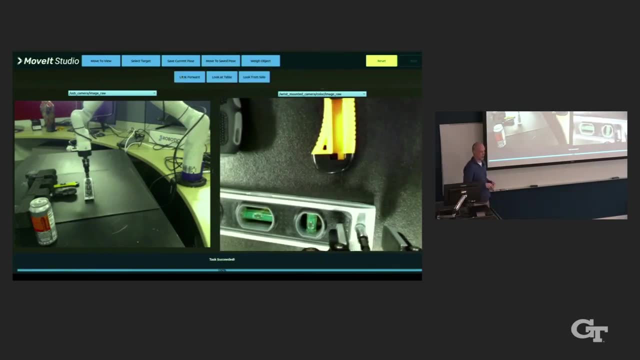 This is right now. it's shown in in a QT app. if you're have a partnership at Foreman's, which is maybe a company some of you have heard of, It's a cloud robotics companies- Now you can just log into your browser. 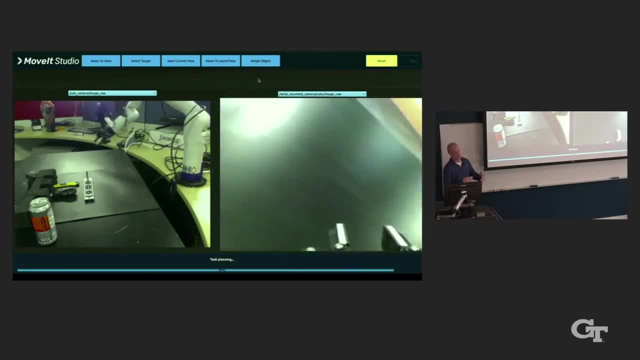 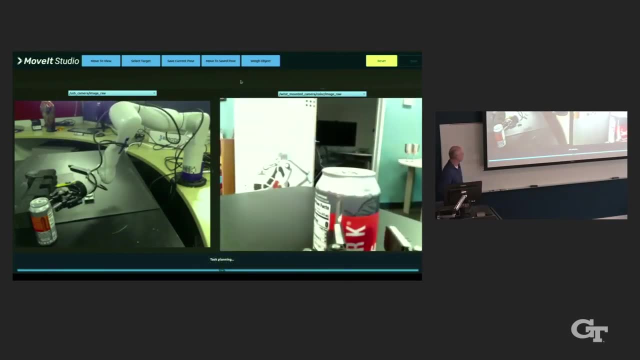 and sort of: once you log into your browser, select the robot you want to control, select the particular release of the software for that robot and that you care about, because you know everybody has their own version of the software and you can sort of remotely control robots. 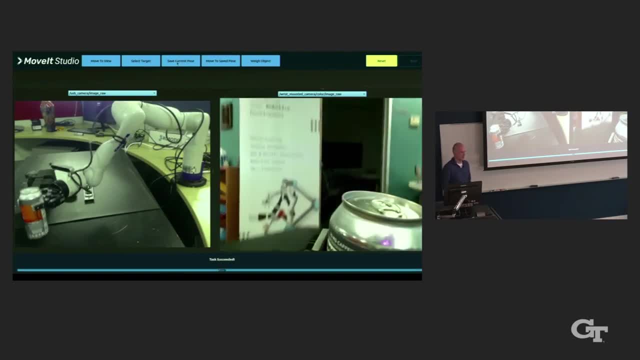 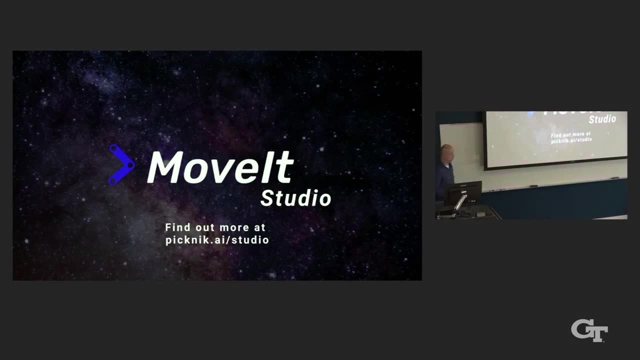 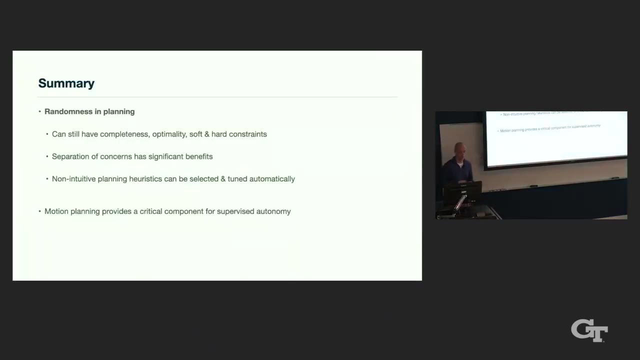 And it's- yeah, it's- really fun to play around with. So we are a remote, friendly company. a lot of our developers are elsewhere in the world, but they can still test on real hardware with just a simple web interface. Yeah, so a few takeaways from this presentation. 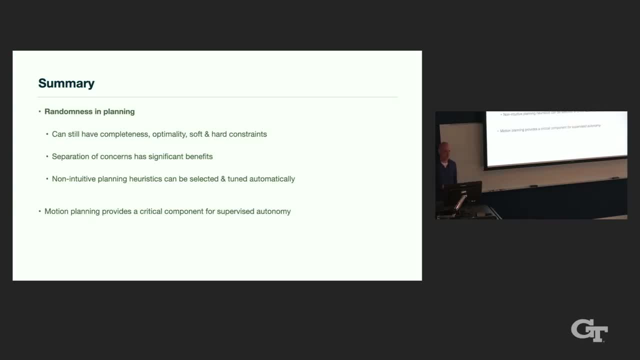 One is about randomness in planning. I think a lot of people when they think of sampling-based planning. still, you know, the stereotypical image is like: this is how your robot moves. with sampling-based planning It doesn't have to be that bad. 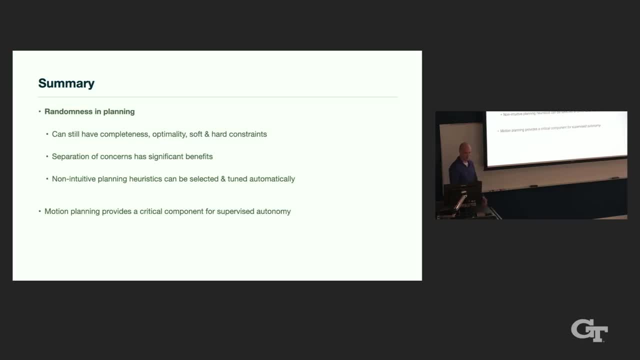 Careful tuning will help a lot. With randomness. you can still have completeness, optimality. you can have soft constraints, cost functions and hard constraints. Separating out these concerns is important so you can really basically accurately optimize for the thing that you care about. 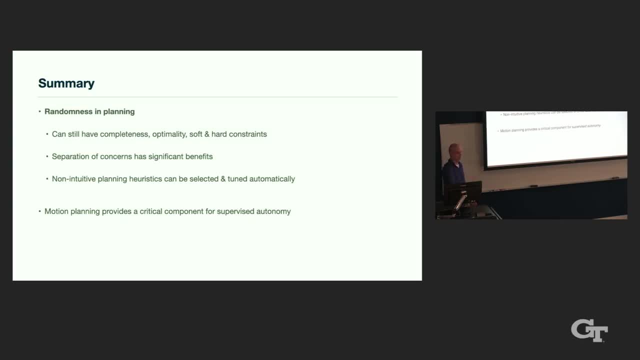 And this tuning can solve a lot of the sort of awkwardness that you see in sort of atypical behavior, in my opinion, and you can actually get high quality motions with a little bit of tuning work. And this motion planning is basically, I think. 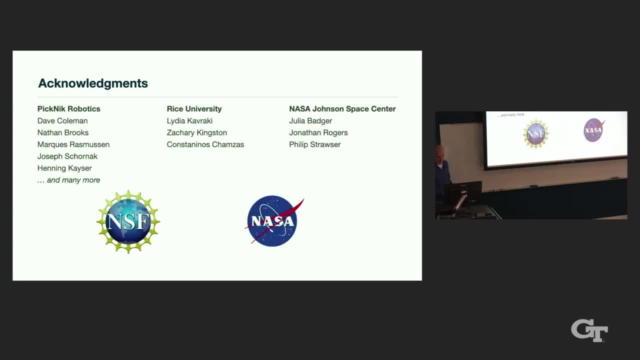 an important building block for supervised autonomy. All right, I see that I'm over time. Sorry about that. Real quickly, a lot of people at Picnic contributed to this. A lot of the work on motion planning was done in collaboration with Rice University. 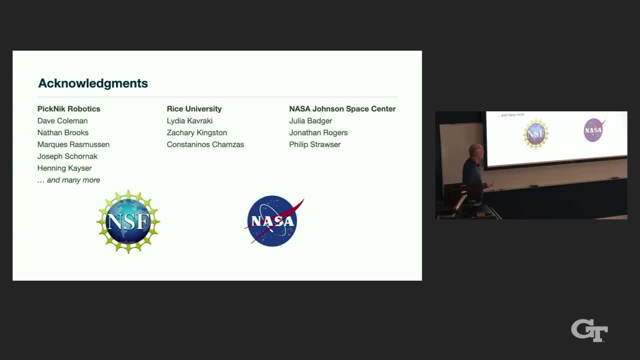 where I spent a lot of time with Lydia Kavracki and Zachary Kingston and Konstantinos Hamzas, And a lot of the work with NASA was done with Julie Badger, Jonathan Rogers and Philip Straar. All right, thanks. 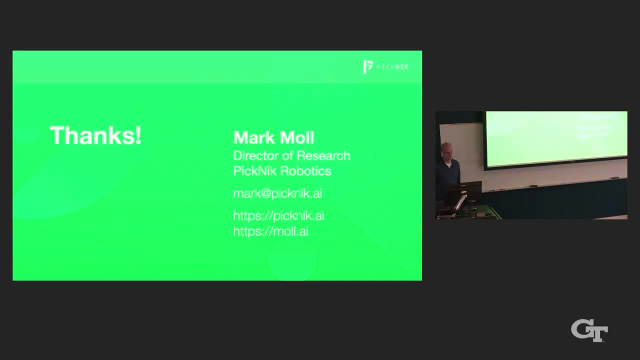 We have time for some questions. Yes, You mentioned actuator uncertainty. What is? how do you currently handle planners where the system didn't actuate the plan given to it? Is there an interface Do you build that into? I can't do this control. 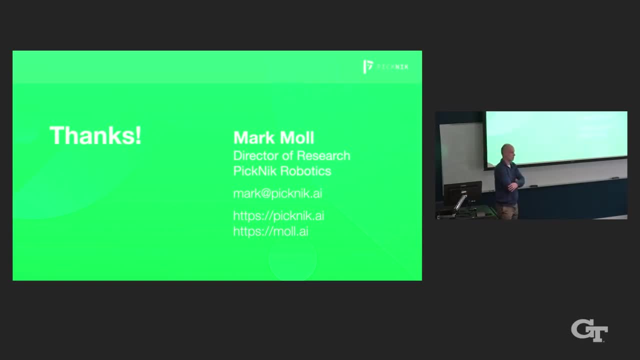 I thought I could. I can't, So is that built back into the planner or is that a decoupled problem? you, just some middle layer handles the control to planner. Yeah, there's different ways to deal with this. One is to: yeah, basically don't do planning in certain cases. 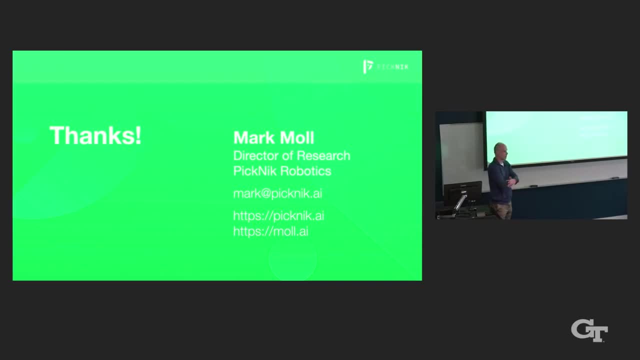 and use visual surveying. That's definitely one solution and that's definitely built into this supervised autonomy software that we have that as a capability. It's like in some cases there's too much uncertainty. We just don't know where everything is. 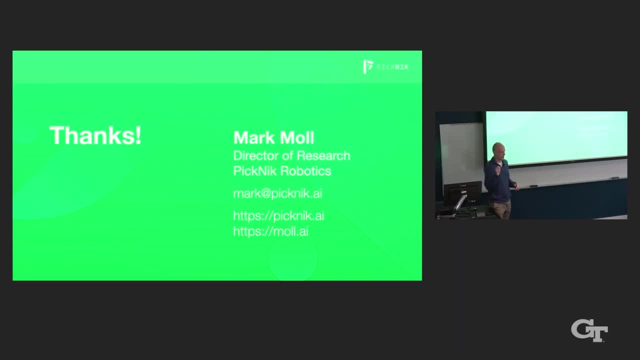 In other cases, having a robust controller, or just, for instance, when you're doing some sort of insertion task, insert past where you think you need to go, just until you basically hit some force limit, It's like don't close, basically keep going. 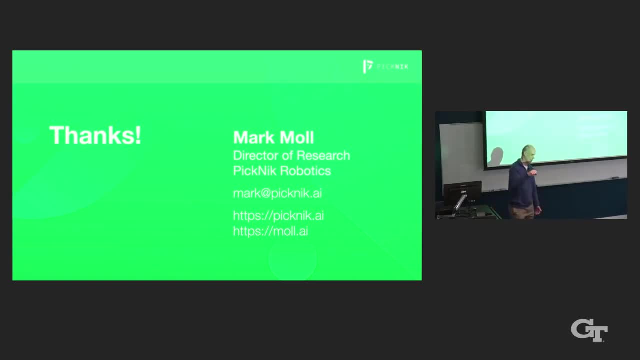 keep closing the door, even beyond where you think it's closed, so that you're really really sure it's closed, because you don't know exactly how far you've moved. Things like that can help. Thank you, Yes. Yeah, just to confirm. 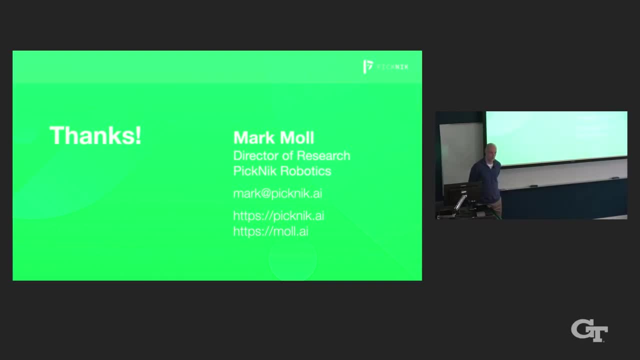 So when we use a normal robot in practice to mill or polish the surface, we're not using inverse kinematics but some kind of more complex motion. Yeah, so for things like polishing and sanding, where you're tracing out something on the surface, with force constraints. 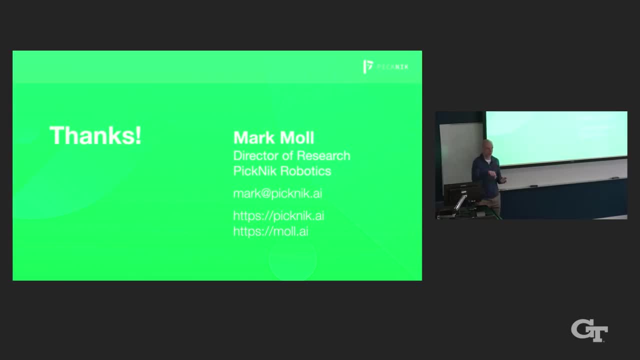 you could plan a global path, first to say, roughly, this covers the entire coverage plan, but then you feed that to a trajectory generator that will say I'm gonna execute this, but subject to this force constraint. So during execution, like epsilon position, error is terrible. 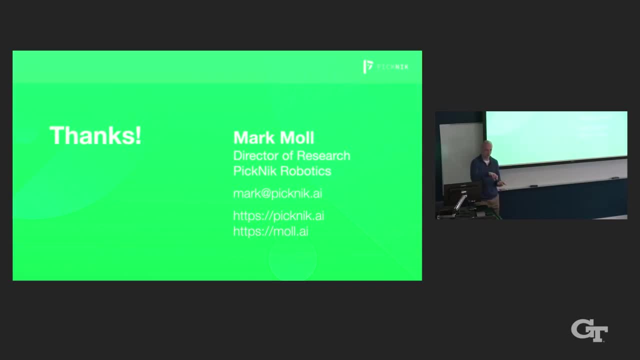 because basically it means the difference between sanding and not sanding. You really need to make sure that the force constraint is satisfied, And so you're basically shifting the priority then towards staying close to this force constraint, So you just have a controller that takes that path. 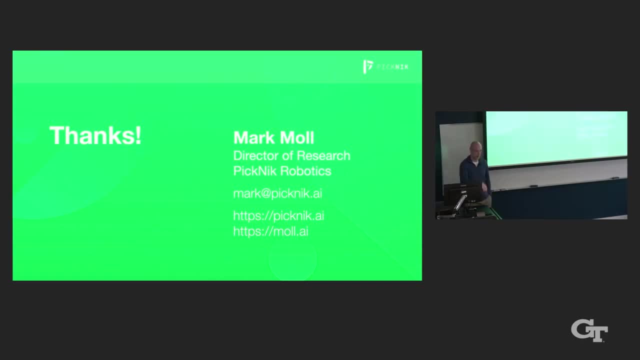 as a reference path, but is free to deform it, subject to that force constraint. Yes, Oh, was there a question in the back I need. Do you have a question as well? Yeah, Yeah, but I can wait. All right, I think he was first. 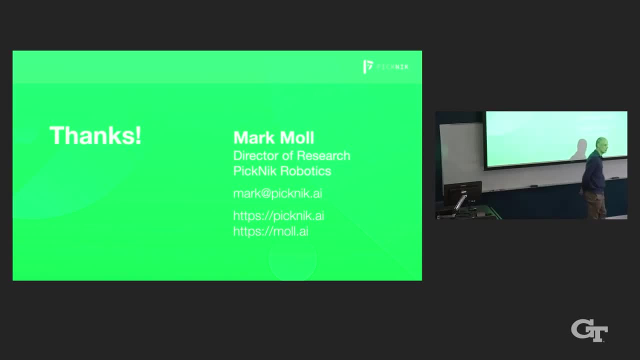 so I'm wondering if you could answer- Okay, Yeah, back on the slide for talking about decoupling planning from the constraints- like, could you elaborate, like, what part gets questioned on the side? Because like there was a diagram but I wasn't quite sure. 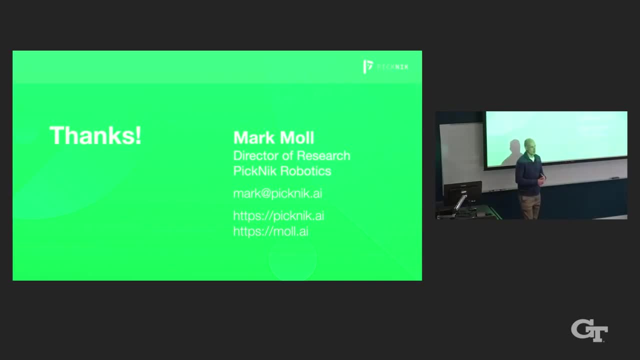 Yeah, For the longest time sampling configurations was seen as like a atomic operation that was inherently a part of the planner, when really you can think of where to sample and how to sample as two different operations And basically what we're doing is we're changing. 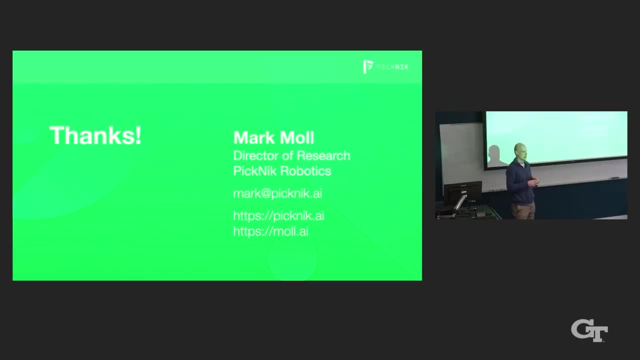 how to sample. we just basically abstract that away to say there's some way to randomly sample. Maybe it's uniform, maybe it's close to uniform, We don't know for sure. but we're doing our best to sort of randomly sample everywhere. 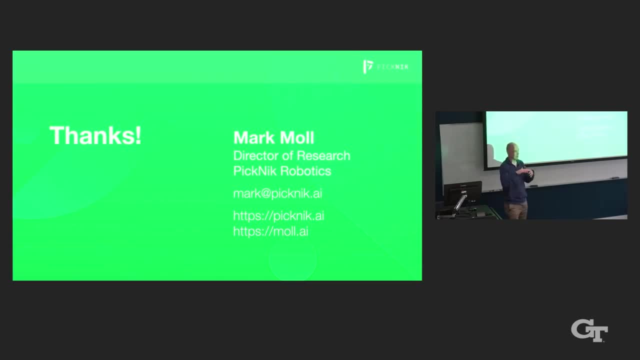 And that's now pushed into this implicit space We don't have. the planner has no control over that part. It's just give me a random sample. But it can still say sample somewhere near this other configuration and that's where some of the heuristics come in. 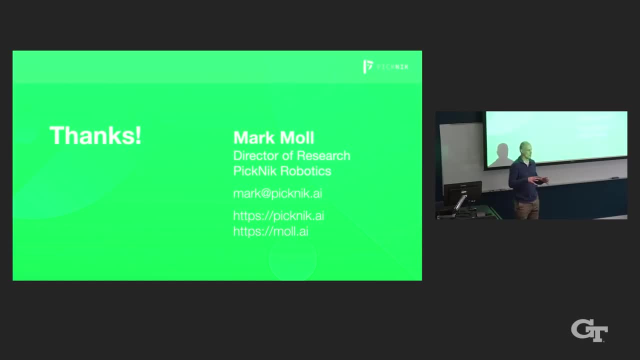 on where to sample next, So it controls the exploration exploitation trade-off. It says: okay, I want to. this state seems like it's close to the goal, let's sample around some more until I get to the goal, versus let's sample to some part of. 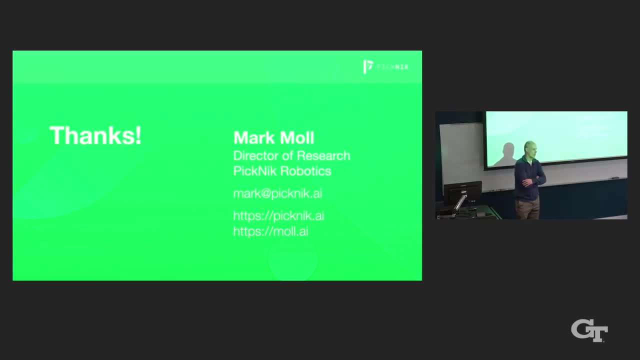 the space where I have no samples, So you can. there's different ways to do bookkeeping and how much coverage you have in a space, But that's what the planner should decide on: how much it should expand everywhere versus greedily moving towards the goal. 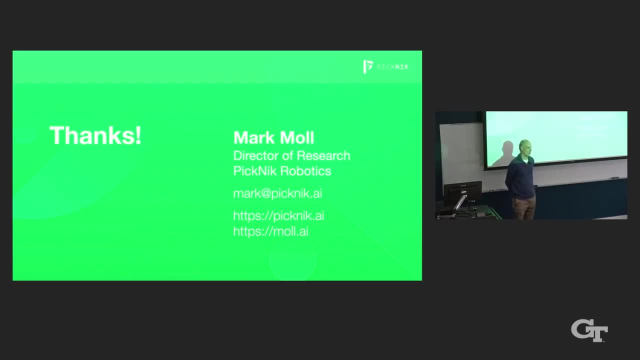 But it shouldn't decide on just the basic operation of randomly sampling itself. As we push that into the state space abstraction, then we can sort of solve these things separately. So a question regarding the hybrid line product: Mm-hmm, Is there a trade-off? are you doing a trade-off? 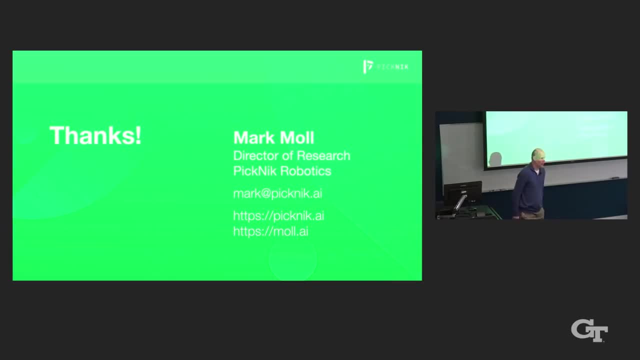 between generalization and specificity when we do the hyperplug framework, in the sense that we can overfit the parameters for the particular environment and gain better performance, rather than what optimal parameters are For sure. If yes, how much are we losing by not overfitting the parameters for the environment? 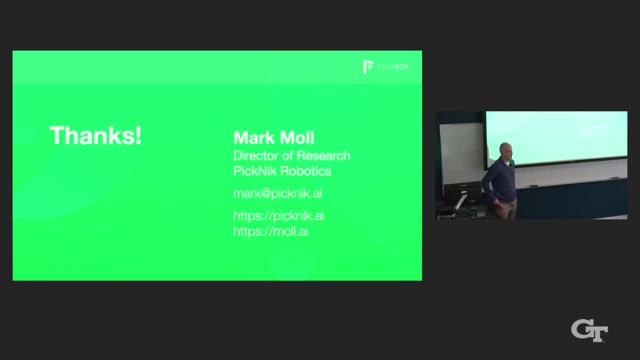 That's a great question And, to be honest, it's hard to say, because how many different robots and how many different sort of different problems do you need to decide that It's hard to say if I- I mean I- showed results. 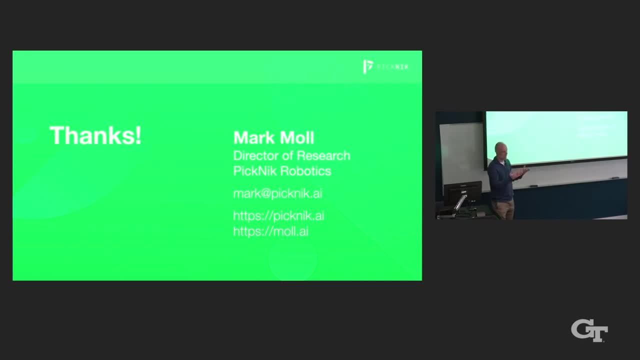 for five different environments, two different robots. They could say something about it, but it doesn't cover the full range of kinematics or geometric complexity of real-life scenes. right, There's a lot more possible. I have no idea how well this translates. 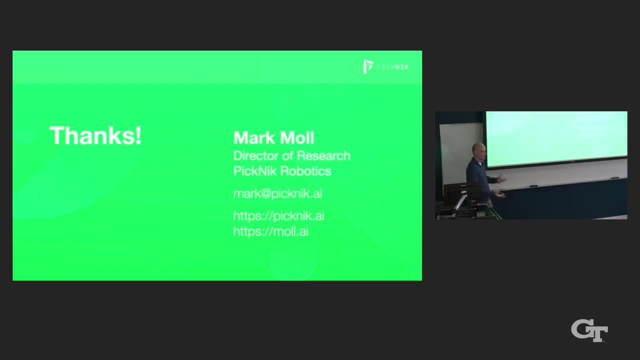 to the results for a stretch, whose kinematics are very, very different from a Baxter robot, And so it's also- I mean, we are at a university, so it's kind of an academic question to ask, but in practice most people have just the one robot. 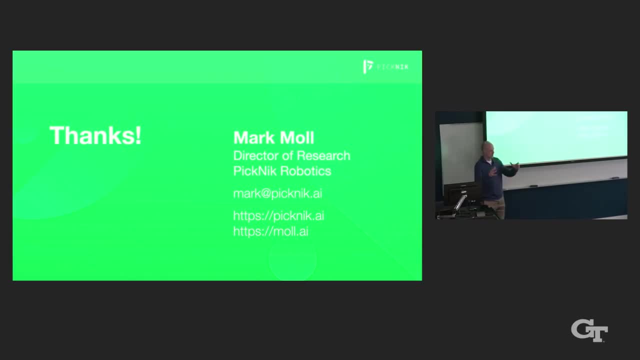 or the one application they care about. and then being able to just say, for these kinds of applications, with this robot, this is the right kind of planning configuration is already extremely valuable, And they, you know, in real-world settings it doesn't matter as much. 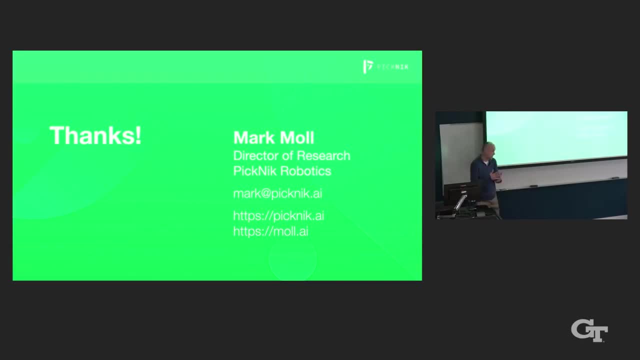 whether it translates to a completely different robot, especially because it's just, you know, a little bit of compute that you have to do once per robot. So yeah, Yeah, Yeah, Yeah. Okay, that's pretty much it. I will take the last question, though.